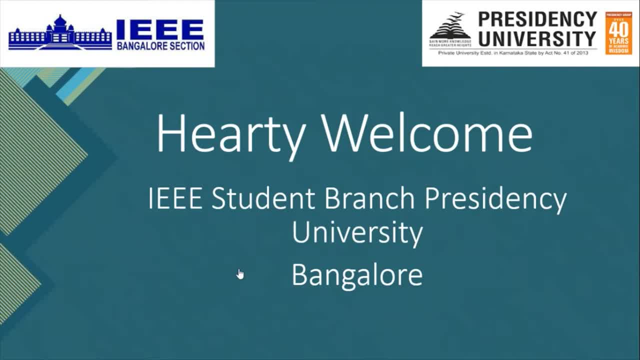 Bangalore section and Department of Computer Science and Engineering Presidency University. It's an international webinar and today we all we welcome you all. Thank you for joining us for this webinar. My name is Shaleen Bhatnagar and I'm Assistant Professor in Department of Computer. 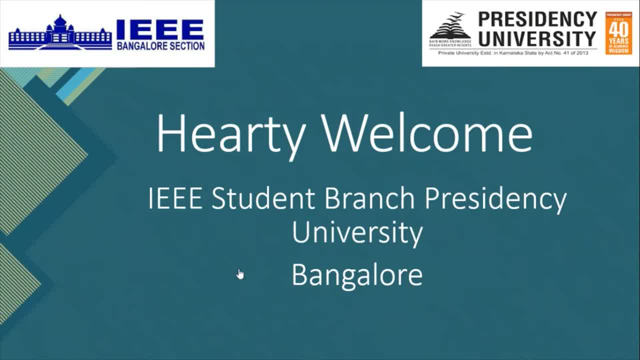 Science and Engineering, And I will be your host for today's event. Now I would like to request Miss Mitali Halder, Assistant Professor Department of CSC Presidency University, to address the gathering. Mitali ma'am. Thank you so much, Shalini ma'am. 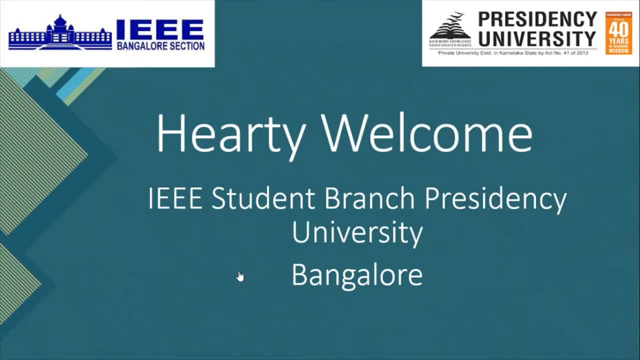 With the mantra: Guru Brahma, Guru Vishnu, Guru Devo, Maheshwara Guru Sakshat Par Brahma Tasmai Shri Guru Benama, With the blessing of God Almighty, I'm so joyous to present And welcome you all on the teachers day and I'm so happy that you all joined this great event for 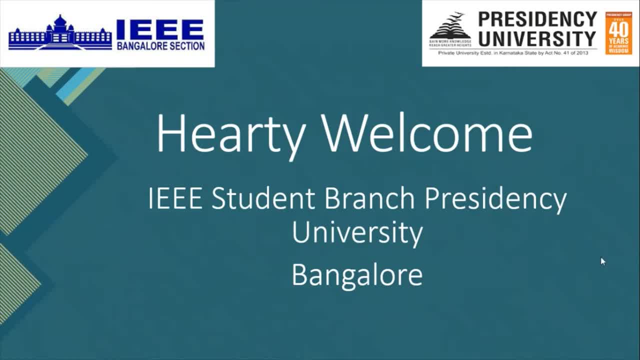 international This live knowledge sharing event. I am Professor Mitali Halder from the Department of Computer Science, Engineering. on the behalf of Department of CSC, I welcome Chancellor, Honorable Nisar Ahmed, Sir Doctor, rather ma'am- Honorable Vice Chancellor, 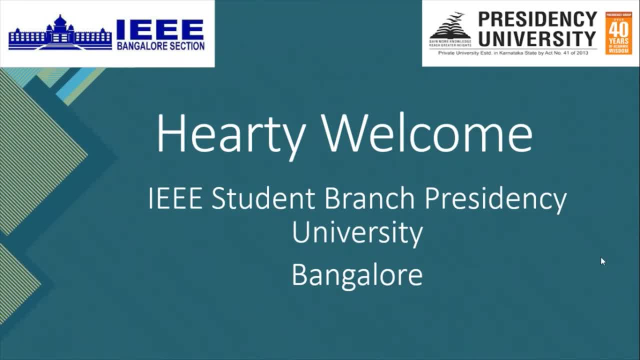 In there: Doctor Sudhendra, Sir COE and Preview Pre, Pro Vice Chancellor, Associate Dean Collider, sensor Department Head Doctor KG Mohan, Our IEEE mentor, Doctor Tevahkuran Sir, All the faculty fraternity, all the participants, all the loving students and the most special, our resource person, Mr Ashish Tiwari. before proceeding, I just want you all to introduce with our resource person and about his credentials. 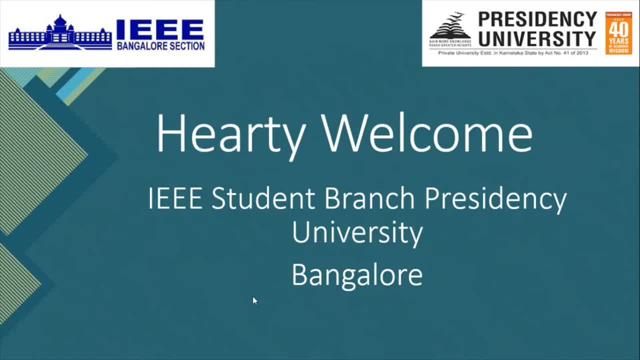 As many of you already know about Silicon Valley, California in the United States, That serves as a global center for high technology and innovation, not limited to autonomous car startups, machine learning, AI, robotics, etc. Today, we are so happy to have Mr Ashish Tiwari, one Silicon Valley robotics engineers, among us as a speaker. Mr Tiwari is a senior software engineer and architect in robotics R&D. 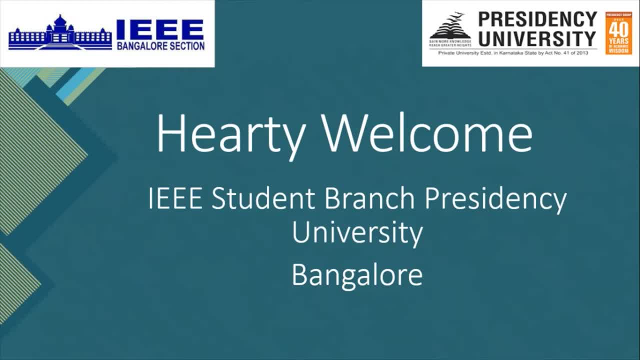 Mr Tiwari is a senior software engineer and architect in robotics R&D. Mr Tiwari is also a research and engineering director at Silicon Valley, California. artificial Ready Bing Inc. A BB Inc Incorporation, which is a pioneering technology leader in robotics. power heavy electrical equipment. 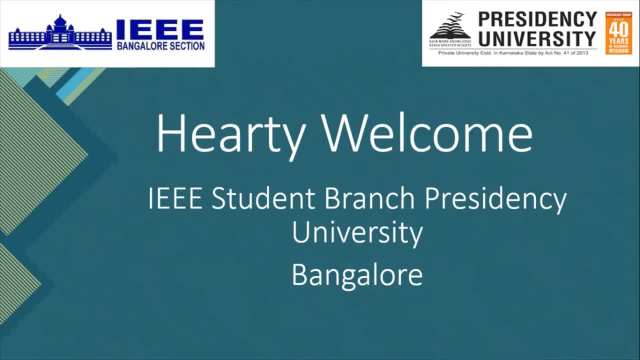 And automation areas. Mr Tiwari owns research interest in machine vision In robotics. Mr Tiwari works are based in three division: data segmentation, Treaty, object recognition applying three D point, cloud based machine learning techniques, automation, extrinsic calibration, automotive, modern technology and engineering. 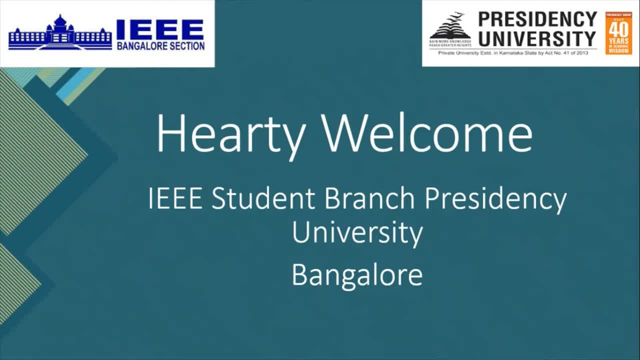 Between engineering AI robotics and webinar AI robotics, sharing this information in the digital arts of Tony. A simple brief: CTO, addition of digital neurobiology and Page Connect technology, NFC, etc. Automated, especially calibration of its work. вами, DePaulo, Then I would like to invite Mr Trudy, Mr Piwari. 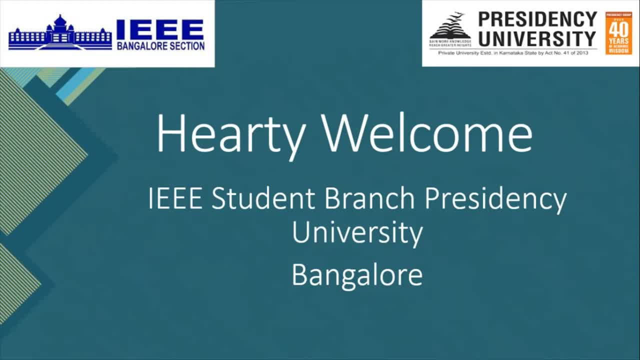 He's a gold medal at CSIC of depth sensors- online calibration of depth sensors. he and his team are trying to solve complex research problems in robotics using machine vision. After finishing engineering and masters from Premier Institute in India, Mr Tiwari also had a master degree. 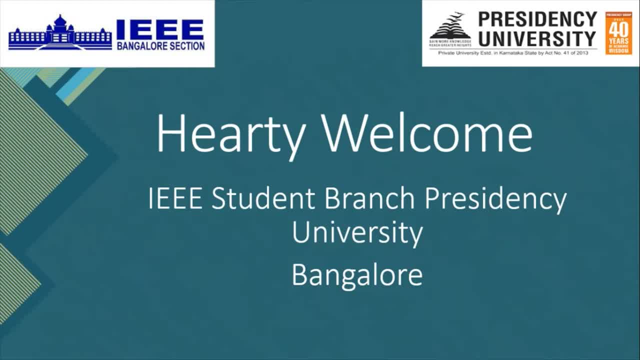 from United States Research University and has been part of research labs. Mr Tiwari will be speaking with us today about machine vision in robotics. So before, without much delay, I like to request to Mr Tiwari to come and share his valuable knowledge with all of our participants. 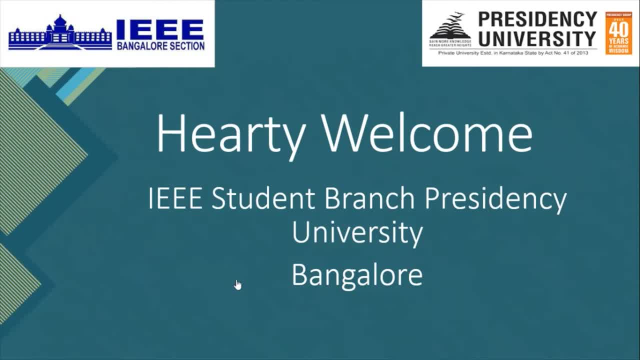 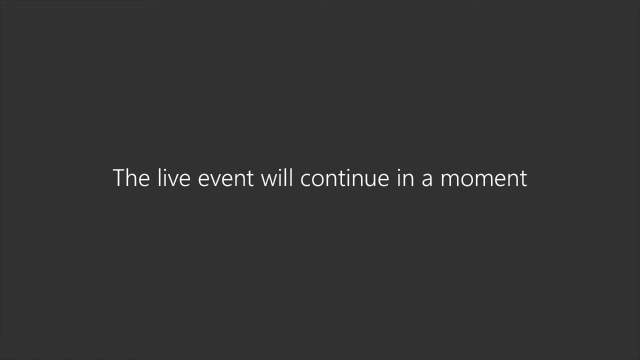 Mr Ashish Tiwari, please welcome. Yeah, hi, good morning everyone. Thank you, Mitali, for introduction, And first of all, happy teacher's day to everyone. You guys able to see my screen right? 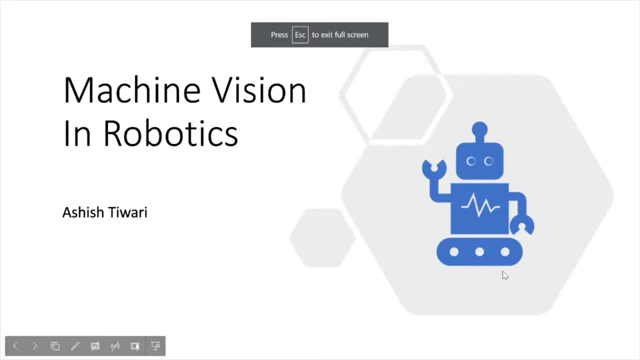 Yes, sir, Okay, So basically, yeah, thanks for introduction. And basically, if people are joining from India, it's very good morning, or if some from other country like good morning to them as well. Maybe we can say all the time. 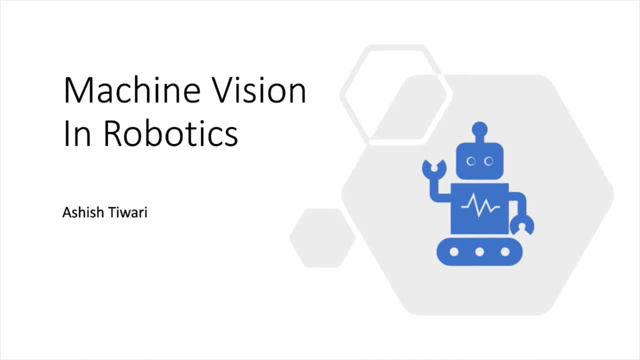 is good morning. so my name is Ashish Tiwari and, as Mitali have already told you guys, I work here as a senior software and architect into the robotics industry and basically we are trying to use machine vision in robotics and try trying to solve some different complex problems. 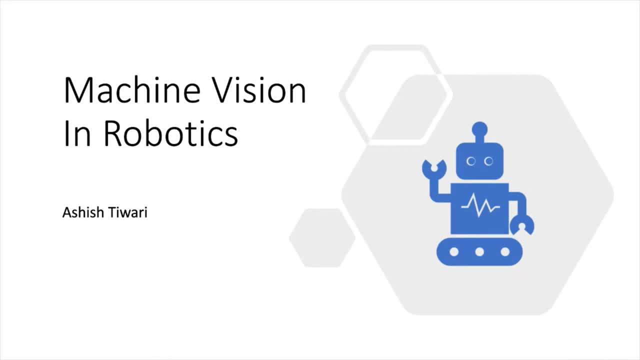 so ABB also work in robotics, one of the segment and we have. basically we are into the industrial robotics segment and there are different application industrial robotics, like you know: car painting and their warehouse automation and all there. we need this machine vision. so me and my team, we are working in this area and today I would like to give more. 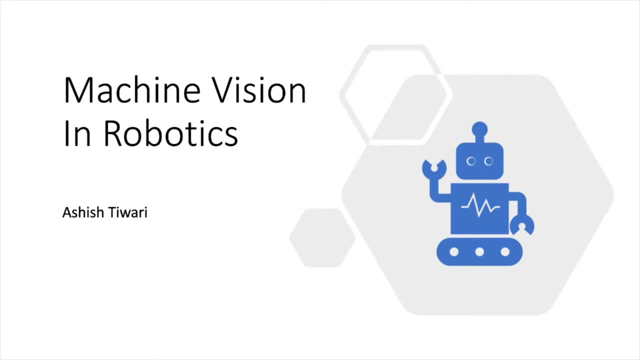 brief about this machine within robotics area and I have been told most of our audience are students like third year or final year. so I have prepared basically like introduction about the machine vision and some are professionals. they are also welcome. they might find some repetitive, but just please bear with me and if any question you guys can. yeah. 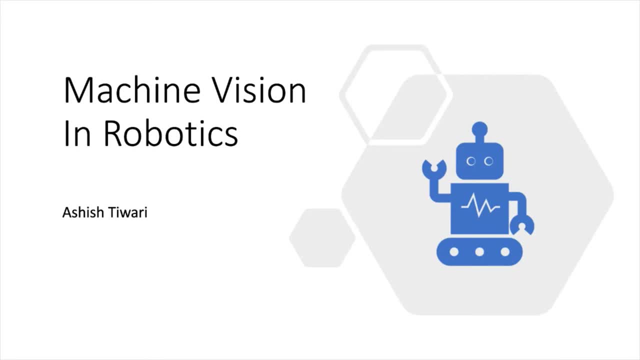 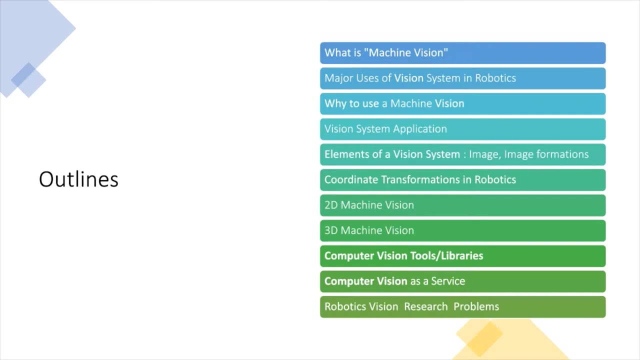 you can put in a questionaries and we would happy to you know answer those queries. yeah, so with uh, so I'm gonna start. so, basically, our topic is machine vision in robotics. so now the agenda for the today presentation is like I would like to divide in different sections. 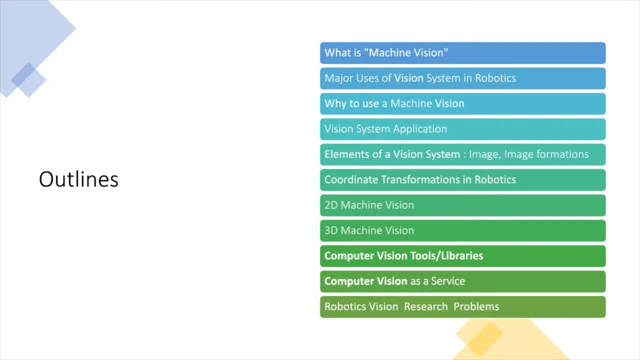 so basically we are going to cover what is machine vision, then major uses of vision system in robotics. then we are going to see why we, why we should use a machine vision. then in general there are vision system applications. then we can find out what are the elements of the vision. 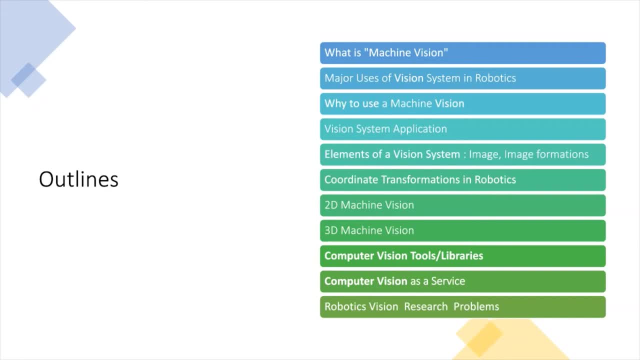 system that could be image, image formation, then if we go in a robotics area, so there are coordinates transformation in robotics, then there are. we also try to segment in machine vision, in 2d machine vision, 3d machine vision, and there are some important and good 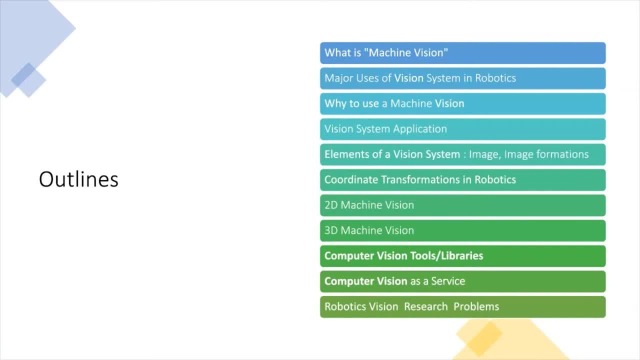 resource and some vision tools for students or newcomers, those who would like to have, you know, career in machine vision or computer vision, and then computer vision as a surveys and there are some research problems. so this would be the agenda. so I'm gonna start about the introduction, right? 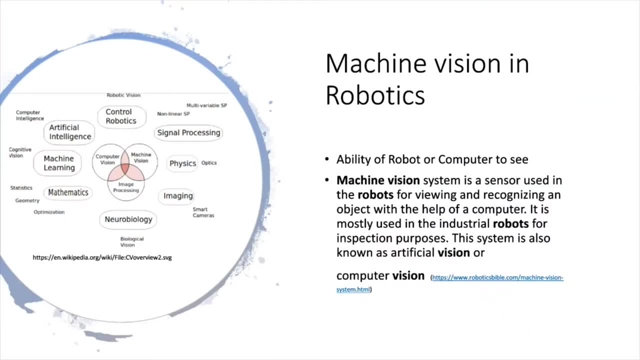 so basic introduction about the machine within robotics and, first of all, what is the machine vision? so, if anyone of you are listening, so basic motivation comes for the machine visions from the human. so what, what is actually? researchers are trying to do? right, researchers are trying to do. 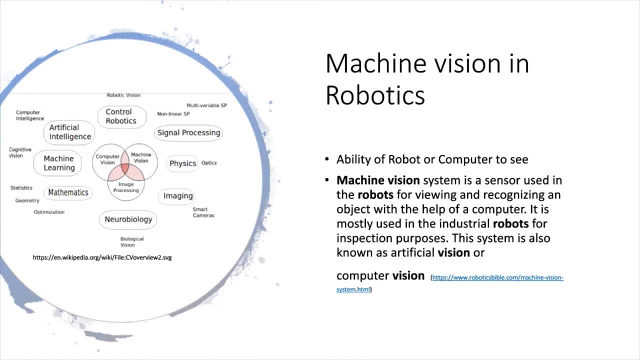 to make a robot or or or enable the computer to do things like robot is, can able to do whatever the human can do. now, human, human have different capabilities. right, so we have a senses: we can hear, we can taste. right, then we have a vision, so we have an eye, we can see things, and then we can. 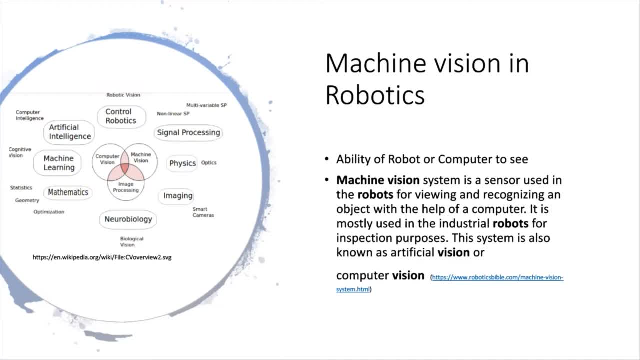 decide. so now human has the eye, the similar manner now robot or computer would like to see things and would like to decide who would like to take some decisions. so basically, one sense of the human is just a one sense that the eye, the vision. so similarly, the ability of robot or computer to see. 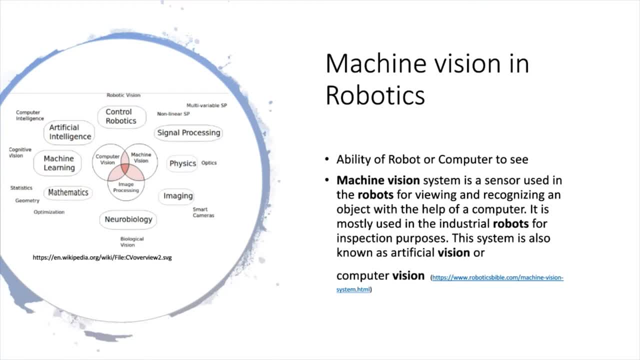 that we can say that's the computer vision or machine vision. So now we can say another sense if we go in a robotic context: so robot is just machine vision, is just like a sensor that using that robot can see and using those some computer, some algorithms we can process. if there are different applications, if industrial robot. 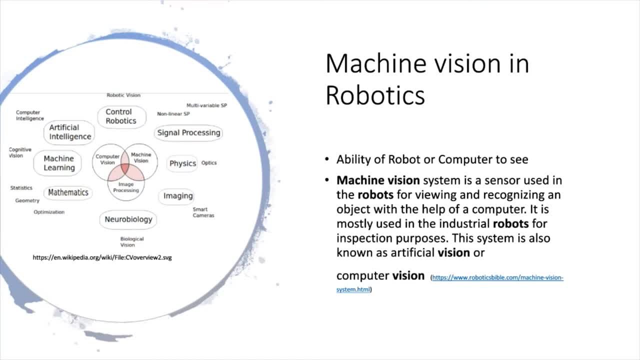 we can. we can have different application like inspection or okay. so machine vision is also, if you see the left hand side. so I have taken this graph from wiki just for introduction. this is basically computer vision and the basics of computer vision also is image processing, so it's also called machine vision, image processing. there are different signal processing, so these: 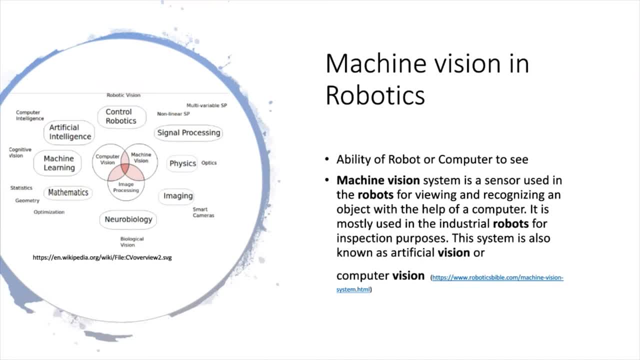 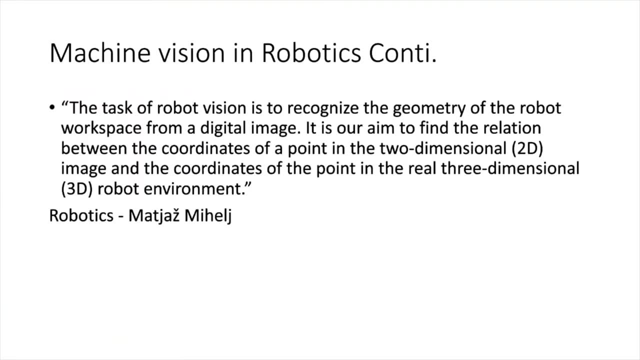 are these areas, and I would call it machine vision, is deep learning. so later stage, later slides, I would like to explain it more about it. so that is so. now I would like to put it into code, one from books from my hills. so the basically say: if in only the robotics, 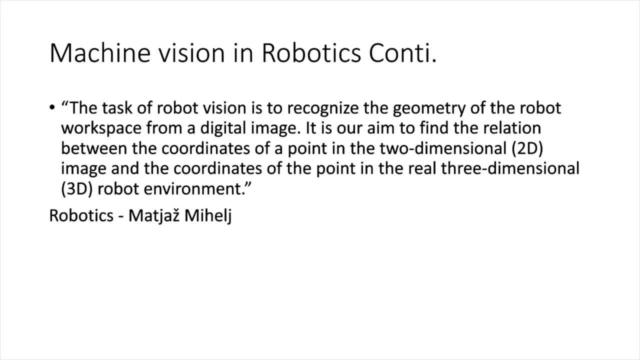 context. what is the machine vision in robotics? otherwise it will be very huge and very broad definitions. so basically I will quote as it is. the task of robot vision is to recognize the geometry of the robot workspace from a digital image. it is our aim to find the relation. 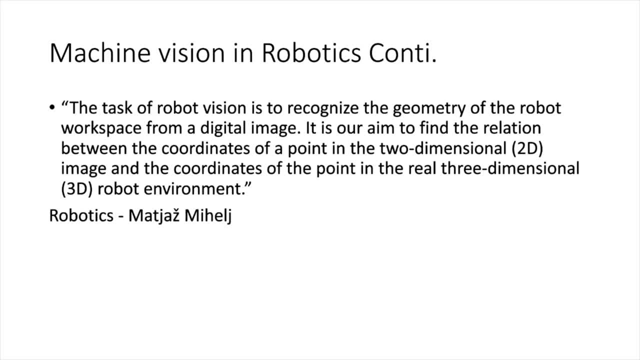 between the coordinates of a point in the two-dimensional image and the coordinates of the points in the real three-dimensional robot environment. so we don't- you don't have to worry if some people are new. what is three-dimensional, what is two-dimensional I would like to have. 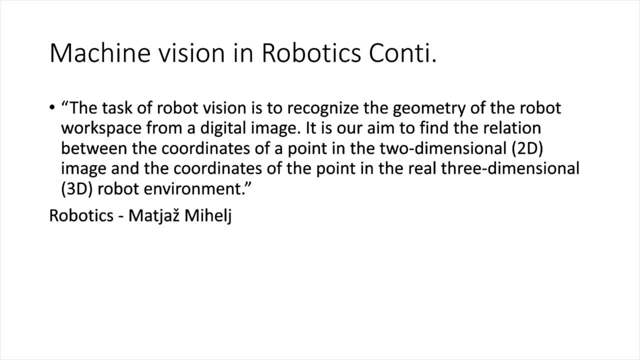 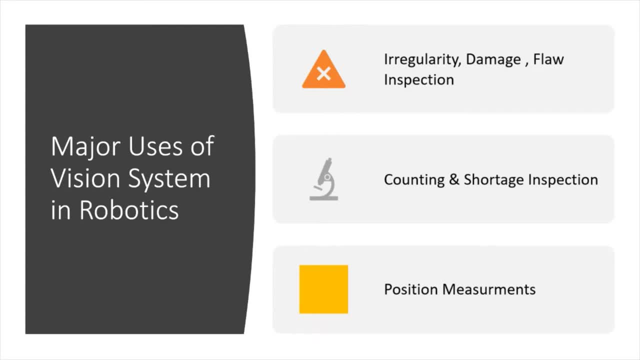 some slides and some detail about it, some introduction about. okay. so next we will see what are the major uses of vision system in robotics. so when we have a robot system, when in industry we have a robot, or in all those factories have a robot or there are warehouse, has the robot right so we can? 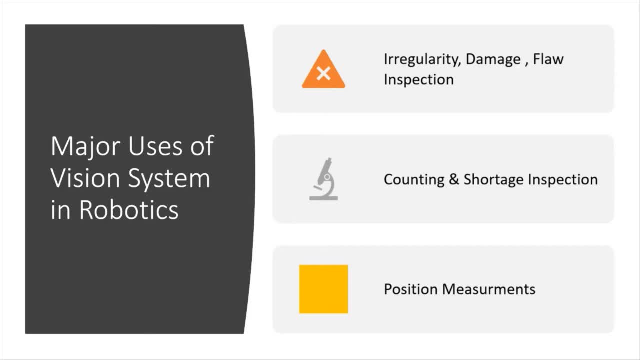 do different things, there will be, like in general, there are many applications right now. I was telling here- major uses of vision system in robotics. so so, like finding out irregularities, the damages, the flaw, inspection with a similar manner, if the task is given to human, if somebody is painting our car, by seeing our eye we can say there is a dent. 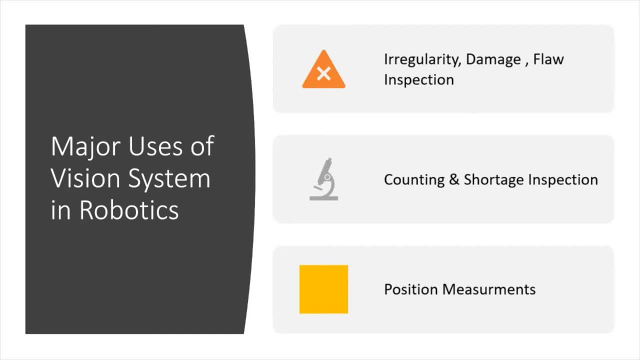 or if the paint is not done correctly. right, how we do that, we don't know right, we cannot explain it, but we do it. our brain see by via the eyes and it can tell you whether it is correct or it is not correct. the similar manner now, if you would like to automate this process using 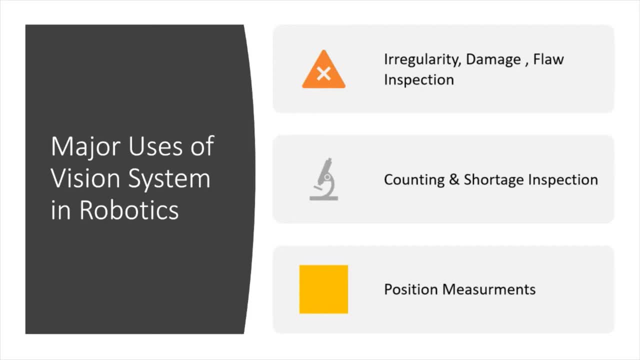 the robot or using this computer or some application, how we gonna do that so their vision system comes into the picture. different applications like counting and sorting, inspection, so we can count the number of objects. like we are in India, like you guys, we use Amazon flip cards or in all. 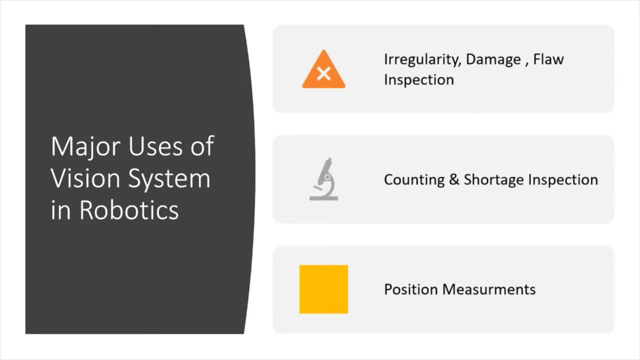 over world. we use Amazon. so if they have to send some objects like that, five or ten objects has been ordered, so they also have to count it, or there are solid inspection, how we can automate things. and then the third one is basically like position measurement. so now 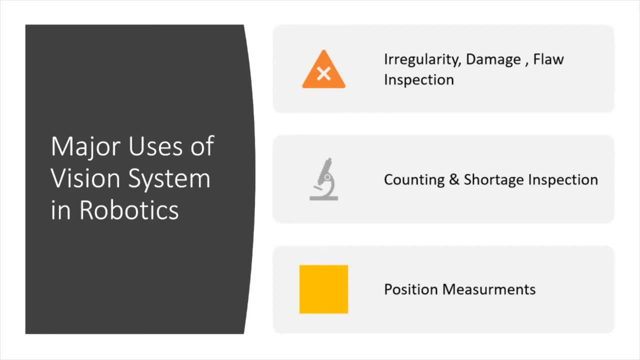 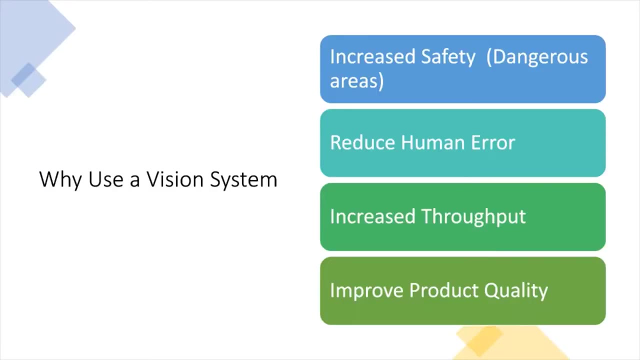 if robot has to pick something and drop, pick and place application or some. so now robot has to know what the object is, in what reference, how much they have. robot has to run to reach to that object, how to grab it. so this basically measure uses. now I would call it why, why we should. 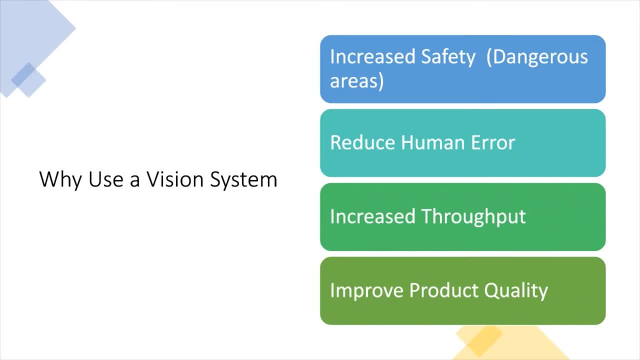 use a vision system now again in general in in robotics context in general, why we should use it. right, we can do with different application, or what is the motivation behind it. so imagine the motivation again comes like a: so now we have to go to Mars. or now there is no oxygen right, so now we can send. 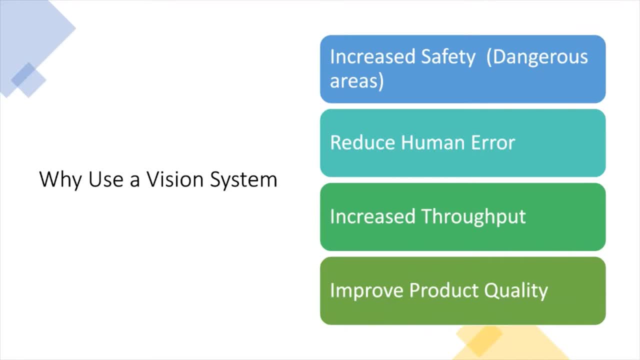 the robot there. but robot has to see, robot has to understand things. so their vision comes to the picture. now we have intelligence- human are very intelligent species, but we also have our own limitations. right, we, somebody have maybe the height, fear, or somewhere there is a fire and there is a hazard. so now we don't wanna put, we don't wanna go into the dangerous. 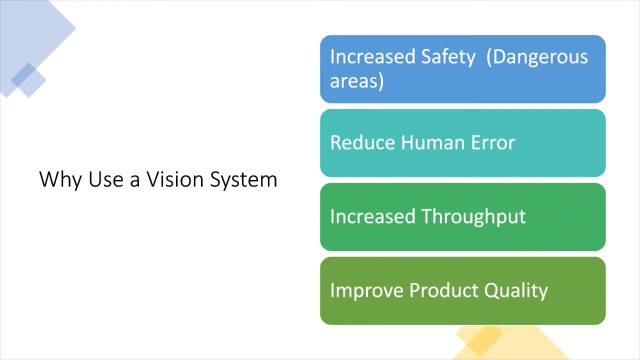 situations. also we can take utilization of these machines or the robot. now there are very repetitive tasks. so even with the human has his intelligence, but with many repetitive tasks we can do those, uh, human errors right. in general we just call it human error. that can be reduced if this task has. 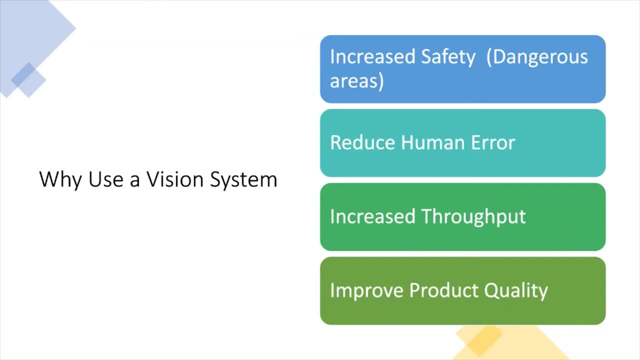 been given to robot or some machine because they do not think much. they just programmed for doing something and they can repeat the same thing. now, the similar manner for increased throughput. this is maybe in some context to the factories or warehouse or somewhere. so again same thing. we are human, we have our intelligence, but we have our limitations. we have to get good sleep. we have. 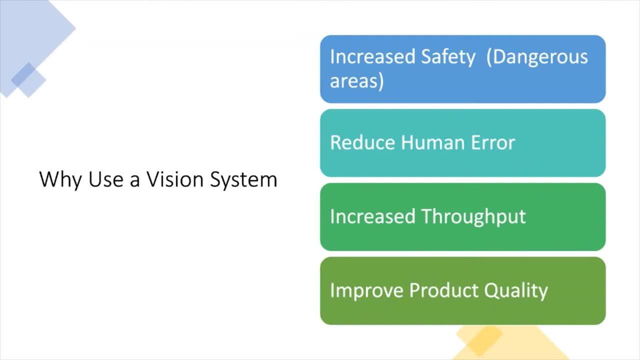 to take a break. right, we have to eat, we have to take bathroom breaks, we have to take uh. we are emotional as well. like people are emotional as well. they are angry, they are happy and they need. so they cannot work continuously, but, uh, if they have to produce a lot of uh products. 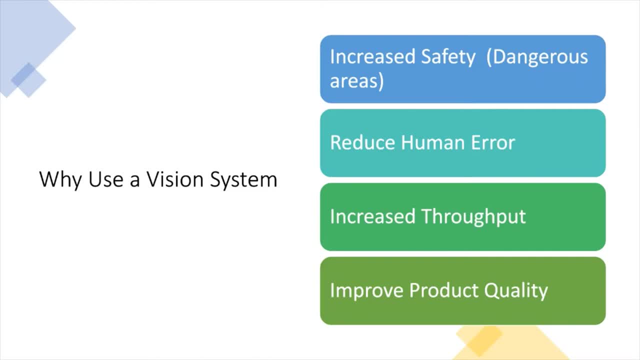 for the world or some. so they need a lot of automation and then they can involve the machine in that case and they can increase their throughput. now, similar manner is the improved product quality, because we're doing repetitive tasks and set to one task. so definitely we'll. 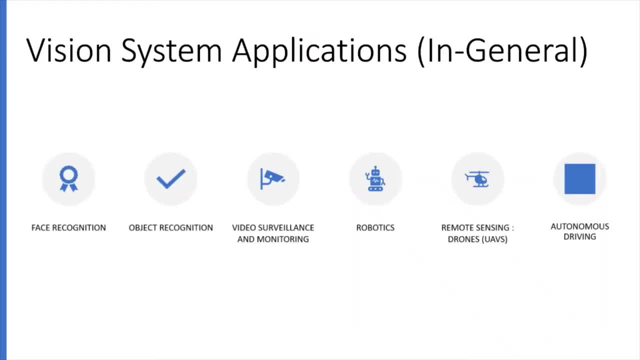 have good product qualities. now i'll talk about uh vision system application in general. though our topics i would like to focus more on the vision system in robotics now there are in general application, so i would not go very much detail about each topic, i'll just give brief. 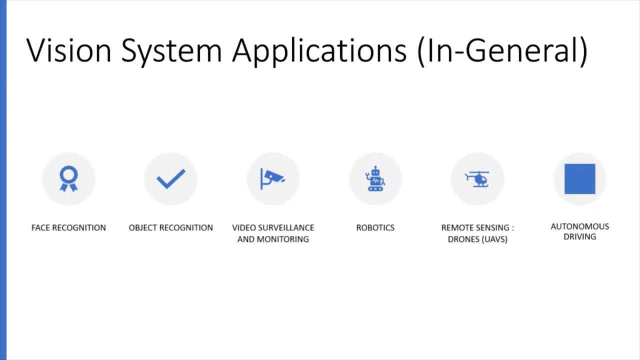 of each uh or each of this topic so that, uh, some of you are interested in the future. you can take this as a career option, you can learn more about it. uh, you can go into the research, you can go for your higher studies or you can have your college projects, your experiments. 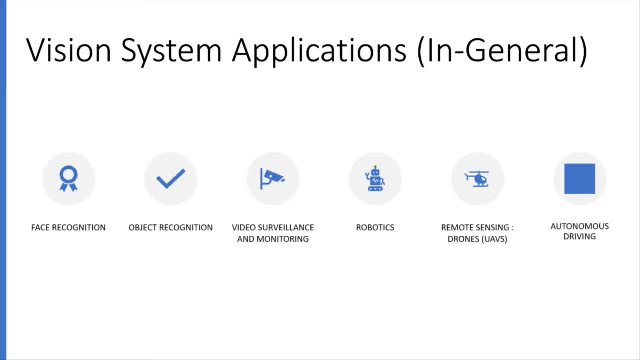 so these are the different. in general applications, uh, you can use a vision system. so now, like everyone of you knows, vision, uh, face recognition, object recognition. we have video surveillance, robotics and remote sensing areas, similarly in the autonomous driving. so now i would like to say: now we also happen. we are in the third year, or final year. i was a student, like once upon a time. 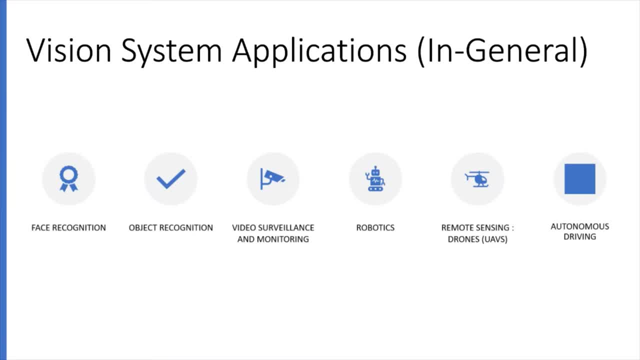 i was a student as well, right, so everybody. so now we can say: we learn programming, we learn c, we learn c plus plus java or all this kind of language, and we say: we have a skill and now i will have job forever. it's a one thing. so 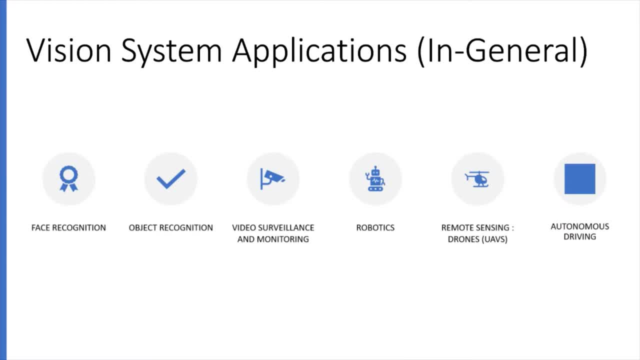 one of the motivational things i would like to talk here. so there's, nothing is permanent, things are changing. even in our computer industry or research industry, things are changing. so one good joke i found it, so i would like to share with all of you. so if you say like, i have these skills and 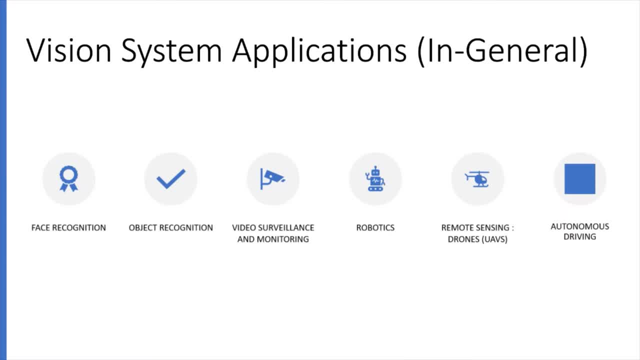 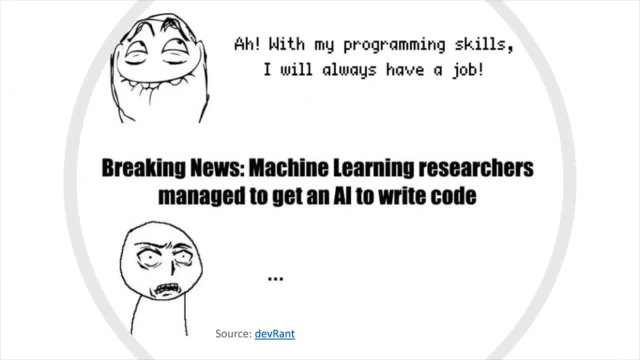 i have my permanent job for all the time and suddenly something happened, and then you will be surprised. so one joke i found i would like to share with you guys. so that joke is that the similarly like it's a. i don't have to explain much, i i guess here. so we say, with my programming, 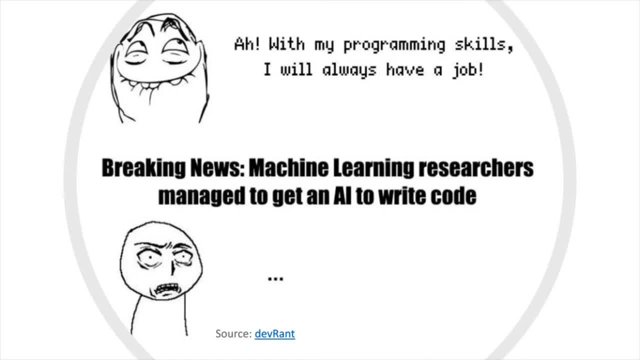 skills, i will always have a job. and then suddenly, the breaking news comes: the machine learning researchers. they manage to get artificial intelligence to write the code. then what then? what about those programs? so why so? change according to the time, like you find your interest, what you like, what you would. 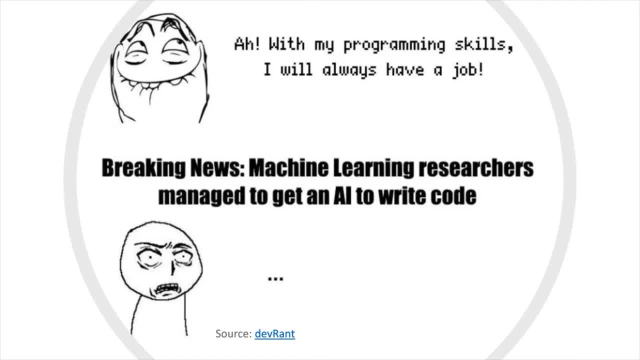 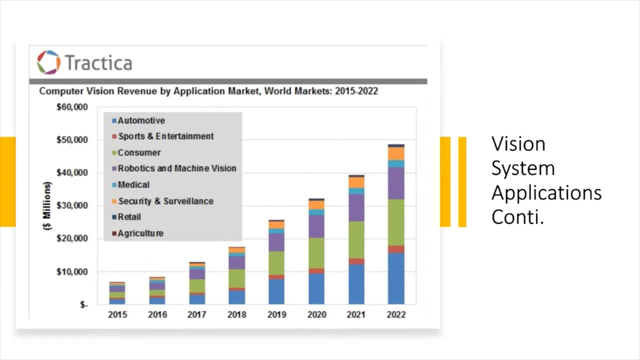 like to do and this just follow your passion, your whatever the good idea. so now we would also, um, that being like one of the funny slide i found in that machine learning and computer vision area, so i would like to uh, just share. so now, further, i would like to talk, uh, what, what are those vision system? 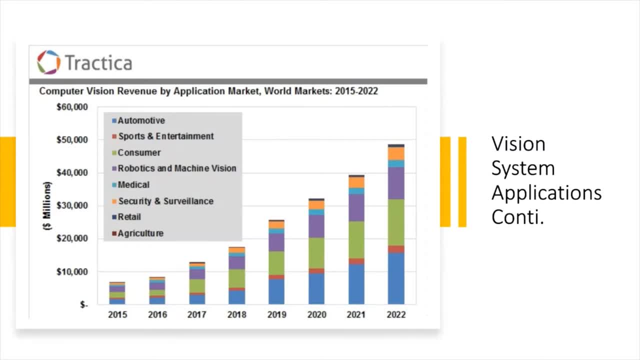 applications. so even like we are engineer, many of us engineer or many were like work in industry. so you know we like numbers. so why like? what is the revenue? what are the benefits of using this computer vision or in this industry? so these days, this is this. uh, we have taken by this uh. 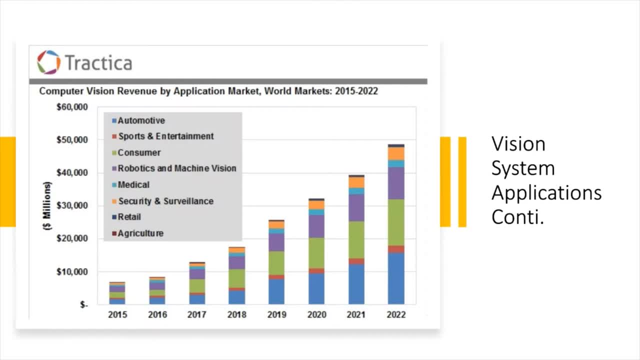 tactica. that's the source and they have predicted by 2022. there's a prediction model and their different segment. uh, the computer vision is popular these days. they are going to be using this uh days. so the different segments. so like automotive industry, sports and entertainment industry. 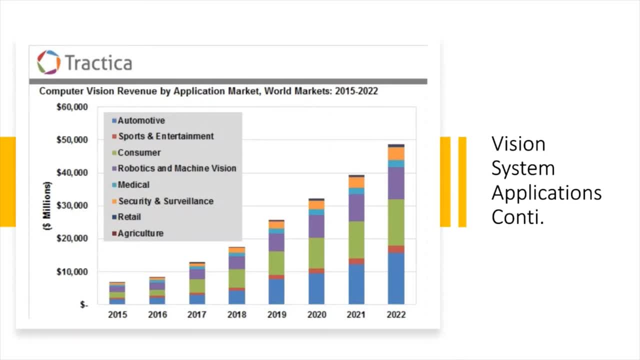 there is a consumer industry- the robotics, machine vision, medical industry. then there are security and surveillance, their retail industry. there is agriculture and if you see this graph, so basically this automotive industry and robotics industry are into the top notch, so they are covering most of the area, and also security and surveillance also some places in the consumer market. so if you 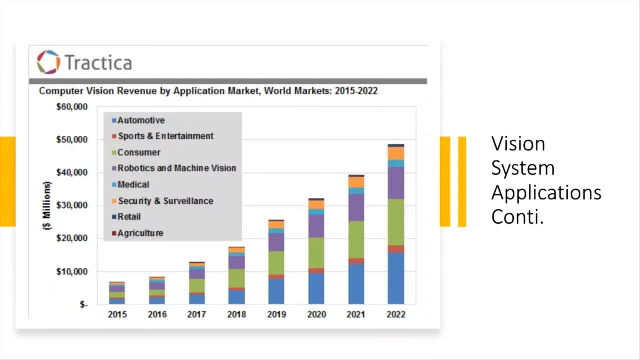 see this: uh, surveillance and the security also is one of the hot topic, or like along with that automated car. so this is a good industry if you are also wanting to choose as your career, or you want to be researchers, or want to be you know, develop, or you want to do anything, your innovation. 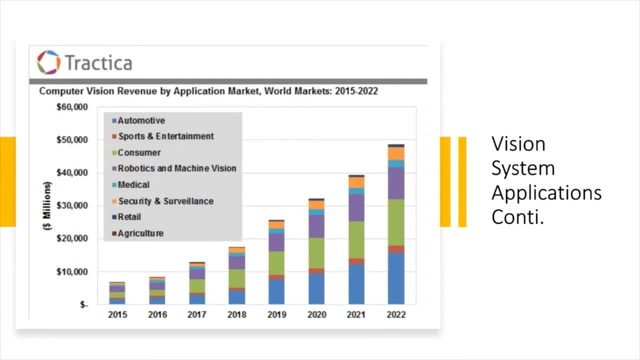 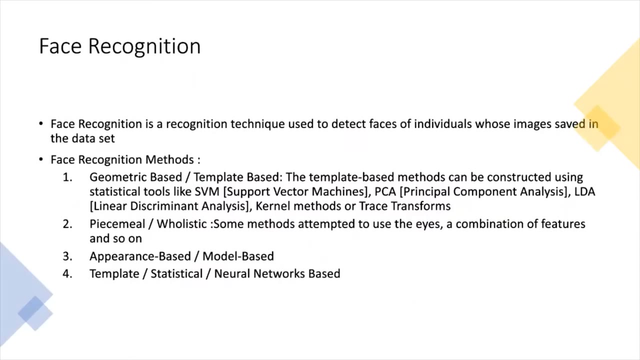 or any startups, so you can see a different area. you, you guys, should try to solve the problems that helps millions of people. that could reach too many people. like you know just the normal thing. like you wanted to make a better world. those phrases now. so i would say that, as i told, in general application, we will just go brief about it. i'll. 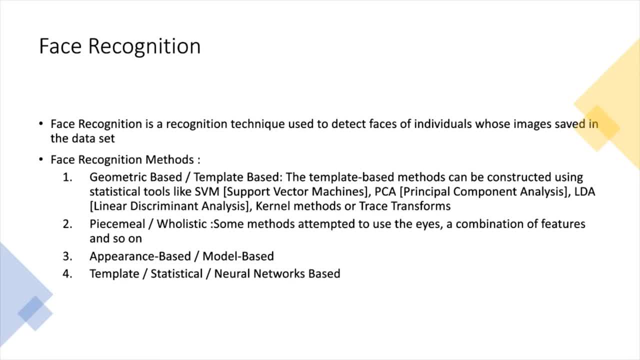 not go any detail because we have to go for the vision into the robotics area, so, but these are uh like just in general introduction about different topic. so right now we have face recognition, so favorite, like everybody we know, like even we have iphone or different camera- uh like mobile these days. 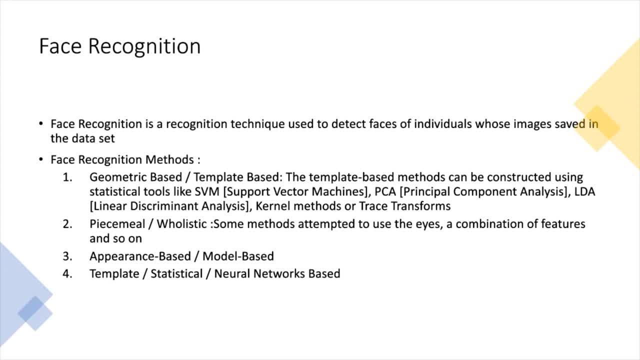 they has the face recognition feature. you can unlock or you can unlock your phone using your face recognition feature. so, like how it happened in background right, there are a lot of algorithms and a lot of things. it's like image processing. there is a face recognition. there are different. 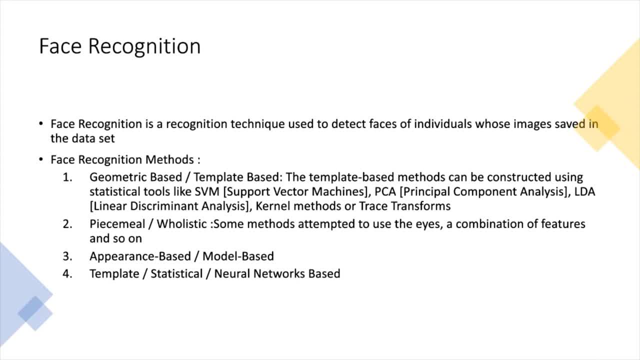 methods so they can do by geometry based methods or templates. they use those support vector machines, principal component analysis and- uh, dumb researchers. they also some methods are holistic, like the piecemeal, so they wanted to use the features. you know features so we can say: like our eyes, our nose, like eyes, feature the distance. 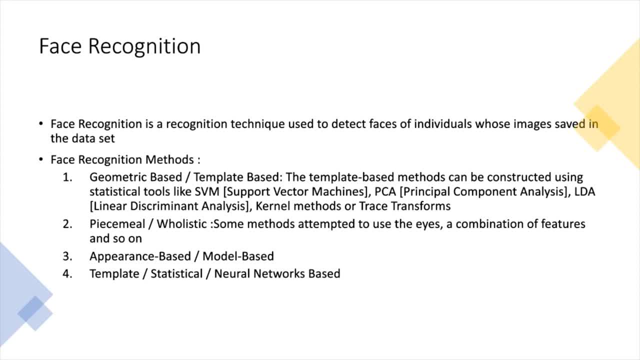 between eyes and nose and the different features. based on that also, they can take a decision whether this guy is this particular face or not like. and then similarly different methods are appearance based, model based, and then we have a template, so neural network based. so now neural network based is actually more popular. it's still more accurate. so one of 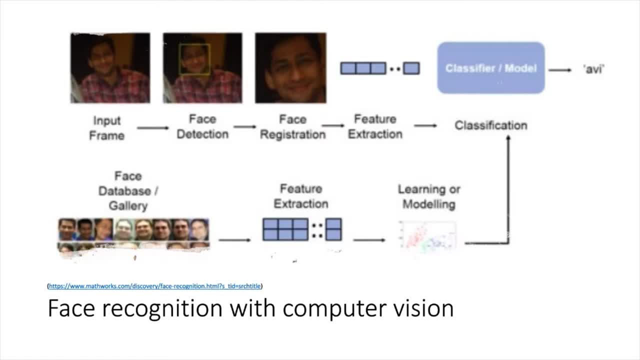 the example here i would like to show with this uh image. so now, if you see, we have uh, some input frames, so how things happen like using computer vision, later i'm going to talk you about. as i am again telling, computer vision is actually deep learning, or it's like. so this can be done by 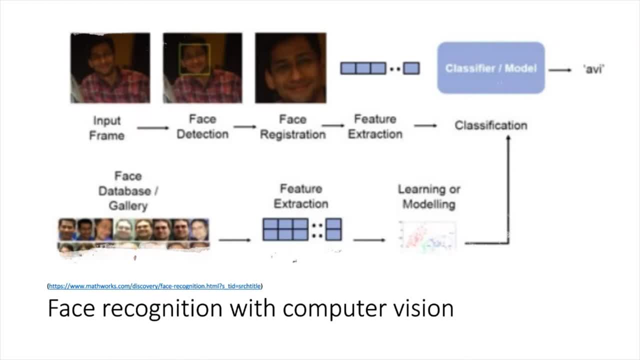 machine learning algorithms. this can also be done by the deep learning algorithm. so here, basically, we have a face database, we have a lot of face gallery with us, and then there's some mathematician or somebody. we decided some on some features suppose, like histogram features or some. 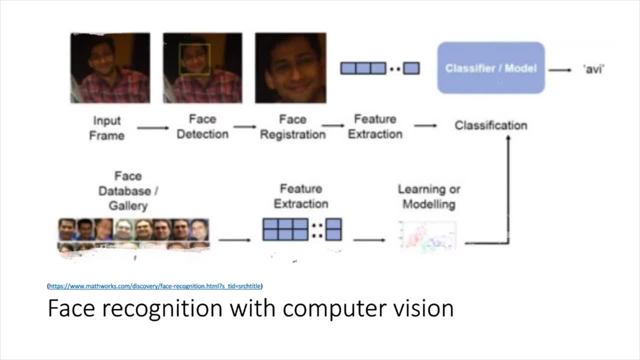 features like: if you guys do google search, there is a google image, find out, then there also, you can find out. uh, you know there is a, the face match. so we have an input frame and that input frame. uh, we can find out. the first we have to find out where is the face right, and then 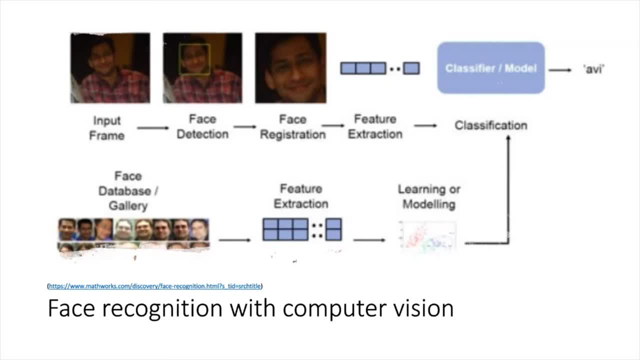 once we find out the face, using that, like some face registration, we can compute some feature extractions, some mathematicals, out of that face. we will find out some mathematical values, some model values and then we will compare this with. we have a database of different feature extractions. 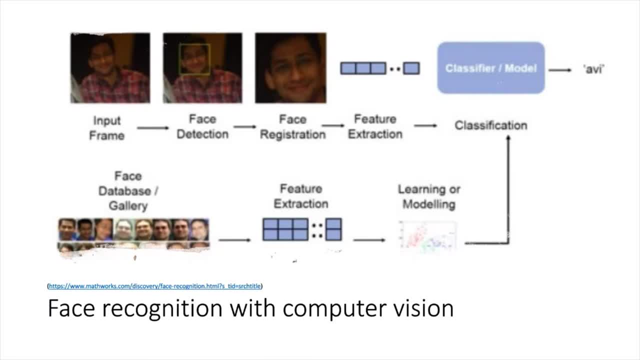 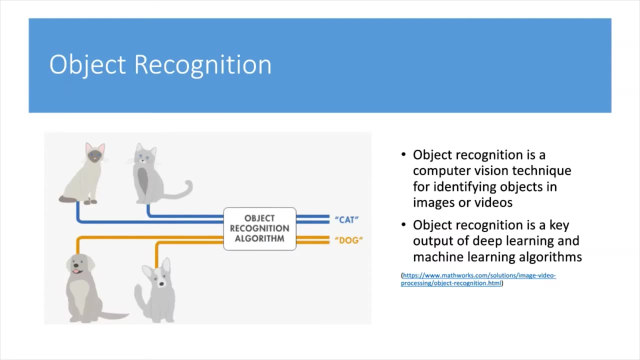 so now this could be one of the classifier. the classifier will match it more like a pattern matching. you have those feature extraction, then feature comparison and then you would have your results, how much close you are to your result in other manner. another application is object recognition, and this is very important and i would 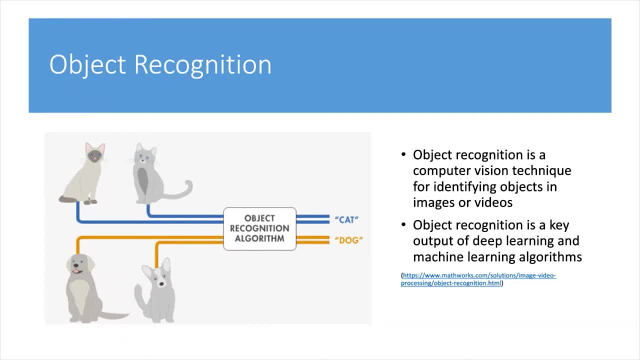 like. i would say this has a lot of applications as well, like so object recognition algorithm. so it's basically one of the computer vision techniques we have to identify objects in images or videos and so we can use again deep learning or machine learning. so suppose, as a human being, if we have given a task, there are 10 images or there are 10 types of cats and there. 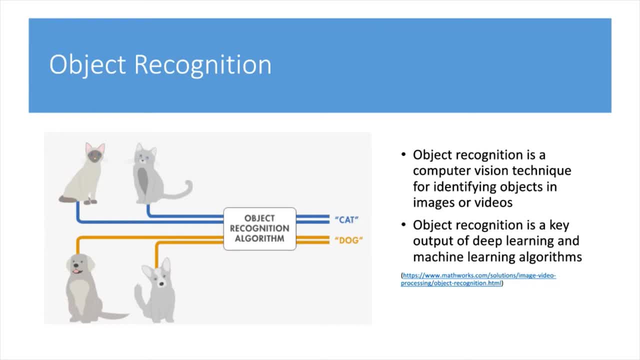 are 20 types of dogs. we can still differentiate which is cat and which is dog. how we do it? we don't know how we do it, it's just we. we learn from childhood. our brain has that knowledge and that utilizing that knowledge and we can take a decision now if the similar task is given to the 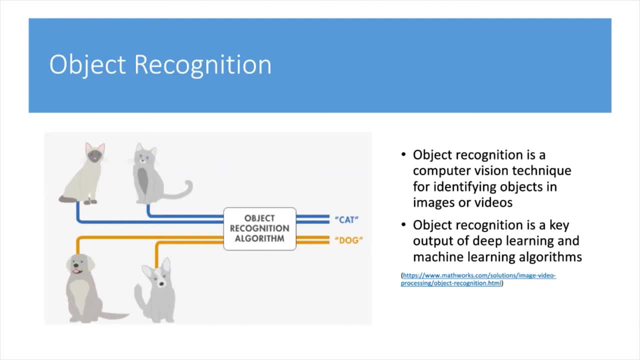 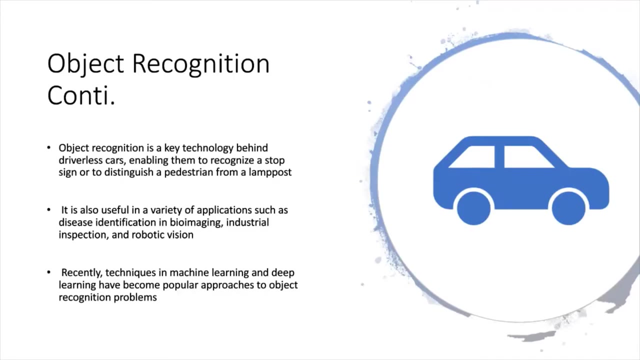 computer or to some robot how it will do that. so similar that motivations comes. it will use those computer vision and then deep learning, knowledge, and then it will take some decisions using algorithms. so this object recognition, now different application, another, this is the key technology. i would say later i'm going to- i have some slides for driverless cars. 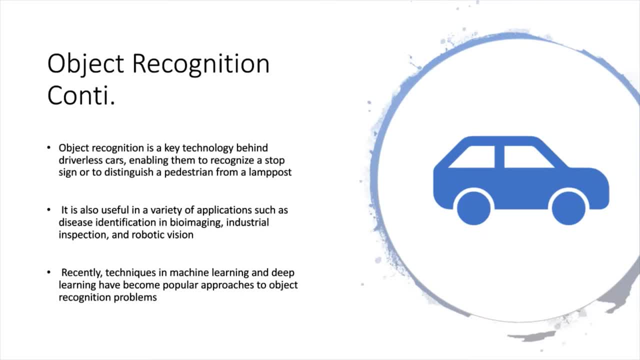 or those auto autonomous vehicles. so there also it is a very important technology right. it's in a enables to car to see the stop signals to all these. you know it can identify where is the pedestrian or where to stop, like when to increase, when to decrease, and there is a ton like so much. So it's very important. We have to recognize things and in different applications Also, this object recognition techniques are getting used, like we used in industrial inspection or in bioimaging. 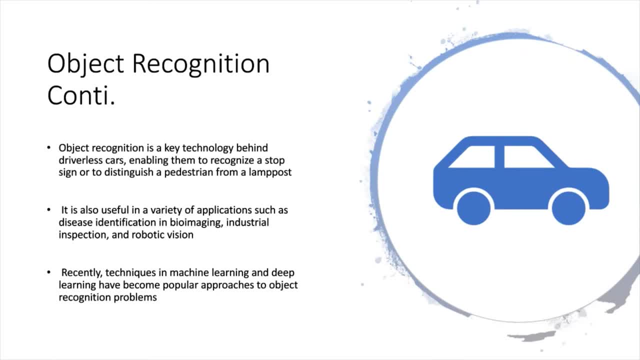 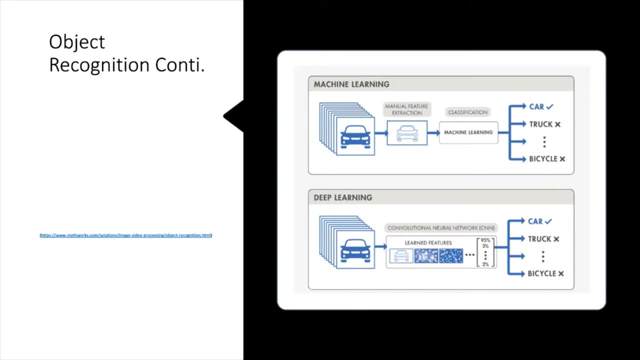 And now we can use, as I told, deep learning and machine learning. So we're going to see further. So one of the image here I would like to show, suppose what happened. This example will be more similar to that- cat and dogs. So now we have car, trucks or bicycle. So our task is, we have different images. Now, among those images, we have to tag them. What are the car, What are the trucks, What are the bicycle? 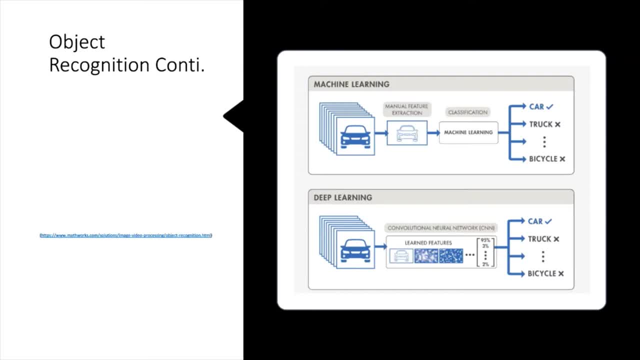 Now the similarly We have our and now we can also see the. what is the difference between machine learning and that deep learning here? So, if some of you might already know, there's a term called like supervised and unsupervised. Supervised means they have a lot of we have to do by ourselves. We have to extract the features, We have to train our system And then when unknown things come for the similar unknown things, we have to again compute a feature and that compute that new feature with the existing trained features. 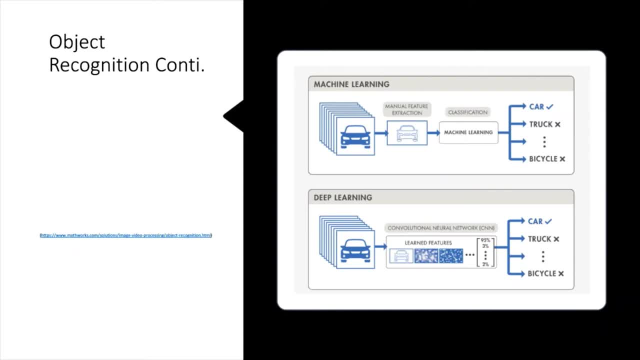 And then take a decision out of it. now, with the deep learning It is more about. I have another, another slides for this one. So there we have a different models, like one is a convolutional neural network- CNN it's called- And then we have a different layers. So, using those vision, you will have your trainings. You also have different layers, and then you can take up same decision. But we'll maybe. it's a good quality result. Now, if you say in another term, 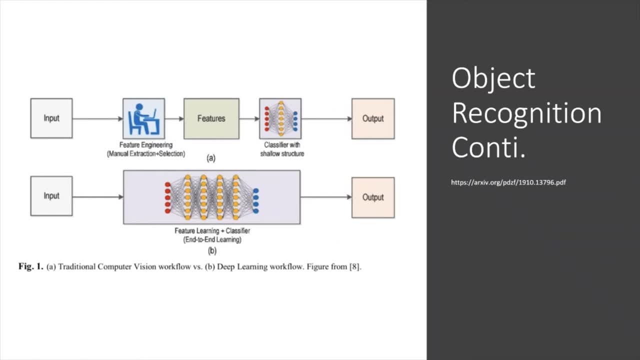 So in in machine learning in the section a, and then the B is the deep learning, section a. even with our human help we have our feature engineering. manually We can compute a feature like we just took a picture. Then we compute some feature. We store that feature in our database. Now some unknown things come. for that unknown things Again we compute this feature in similar manner. Now that one feature, we compute with our existing training and then we decide what label it is. 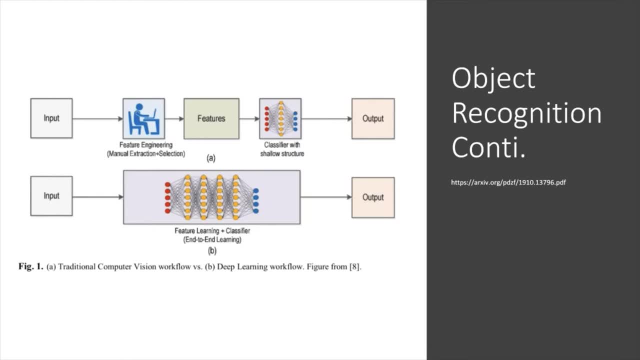 We can classify that. That's the output. That is basically the machine learning here. Now things happen little bit different in deep learning. So deep learning, We can also involve the training. but there are not just one training. It can have a layers of training. It can also utilize the pre trained data. so so you can see in this image there is a feature, learning plus classifier, and then another term called reinforced learning. It can also learn from its own results or, like it seemed, like a human. 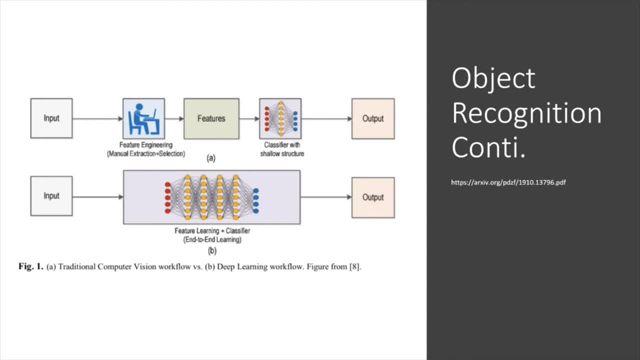 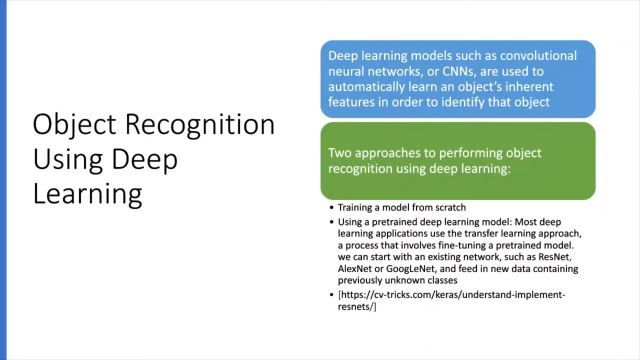 Right, the deep learning and all these neural neurons. There are motivation from the human. So now, basically, again, as I talked about it, this model, such as those, CNN, we are using for inherent features. Now, basically two types of, two types of approaches we can use here. One, we can train a model from the scratch. Basically I was telling about those machine learning or 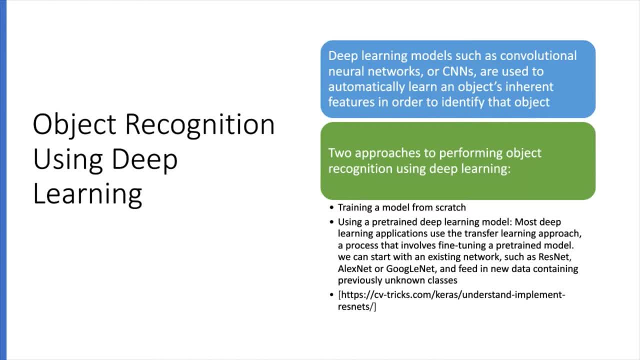 And then you can decide when to use what. so training a model from scratch? If you are having some application that is limited to 10 objects or 20 objects or 100 objects, so you can only train to that 10 objects, 100 objects, and then you can identify two similar objects in your factory. 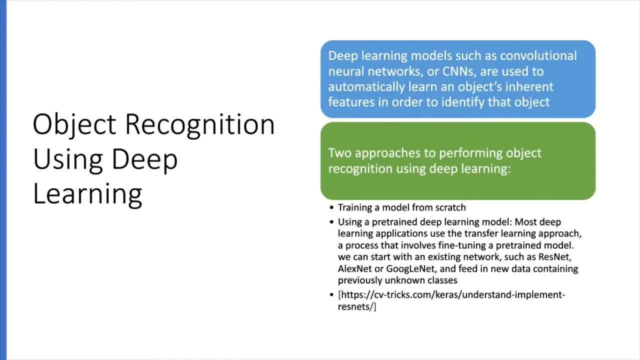 Like if your factory is only about Apple and banana, that's it. So you just train Apple and banana and no other objects would come into the picture. But if you have a broad object recognition Application we can also utilize. we call pre trained deep learning models that I was talking about. So there are different models into the market. There is a google net, There is a rest net, There is a lexnet. 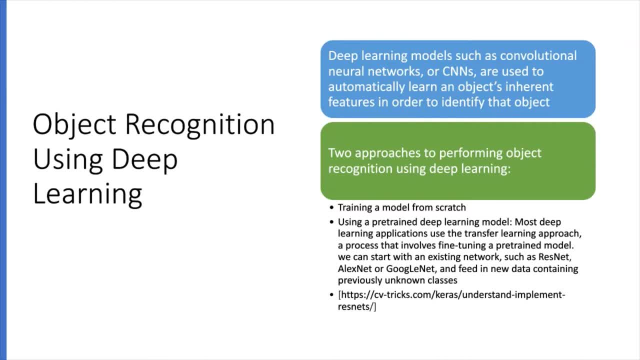 So there, they already trained their model with millions of images. There are millions of data is there, and now, top of that training, we can add our own training, We can train it again. and so this, this: if you, any of you guys, are interested, you can. 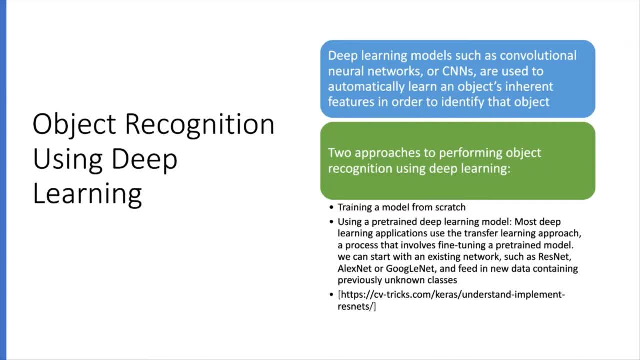 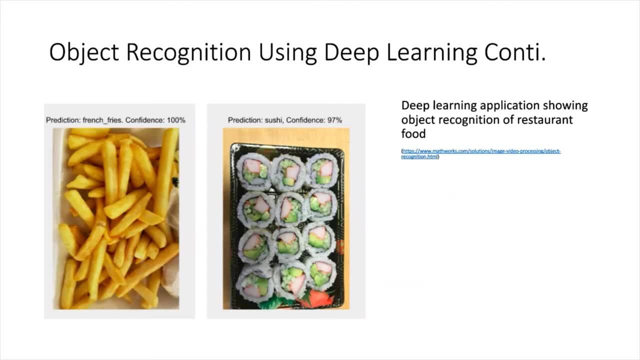 can go further, read about these models. you can go for this deep learning analysis and then, so similar manner, suppose another example, so i was talking about deep learning- can utilize for object recognition. so deep learning. so if we have given a task and it's give you. is this a french? 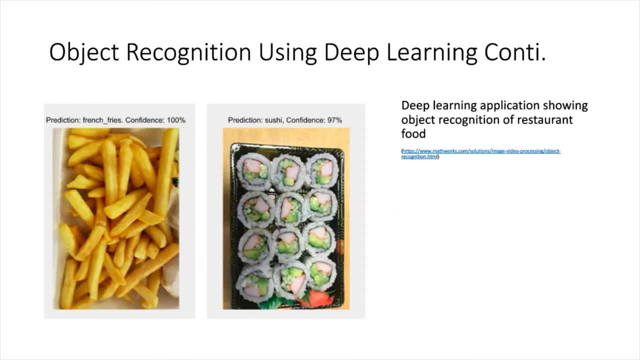 fries or is the sushi. so we have a prediction, we have given some picture and the deep learning model is predicting into the restaurant food: okay, this is a french fries and and this computer is 100 confident. but for the sushi it says, yeah, i am, i, i would predict this is a sushi, but my 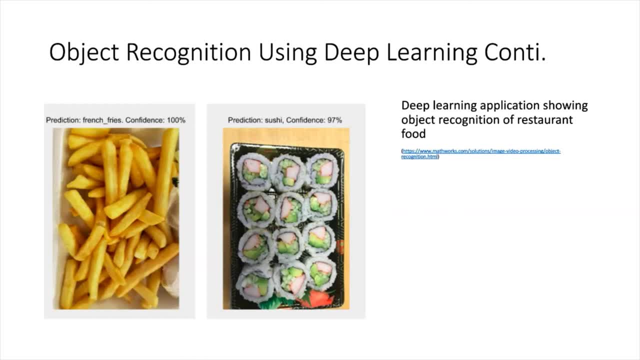 confidence level is 97 and there is also another research. you can also- sometimes you can- fool the computer because something is something that is looks like. this computer can also predict there are error case now. so the object recognition model is predicting into the restaurant food- okay, this is a french fries and this computer 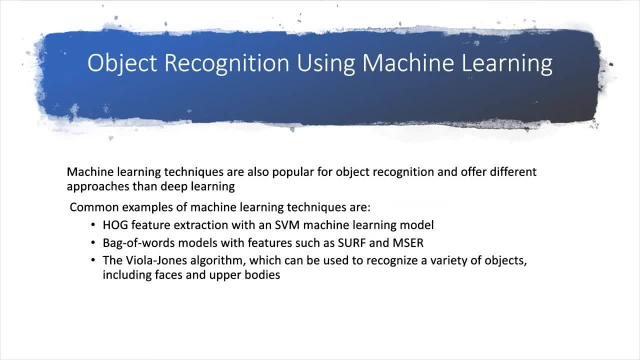 can also predict there are error case now. so the object recognition we did with the deep learning, object recognition you can also do with the machine learning. why i was covering this area? because they are very important and, as i told, in computer vision object recognition is very important. 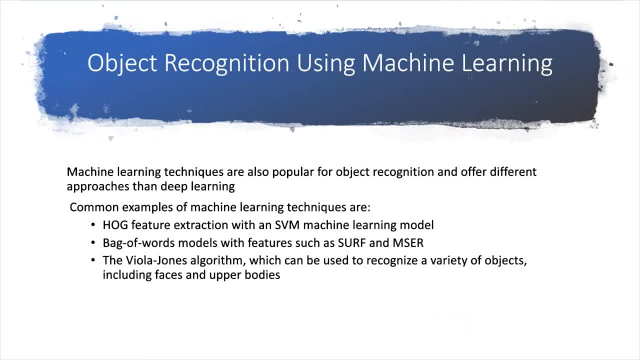 techniques. so now, as i told, if we do not need that much computing, if we do not need that much broad applications, we can also use our convene conventional machine learning algorithms. so there we can use, like you know, different feature based, so object recognition. so there are different features, like one is- you can again learn more about these features- the hog. 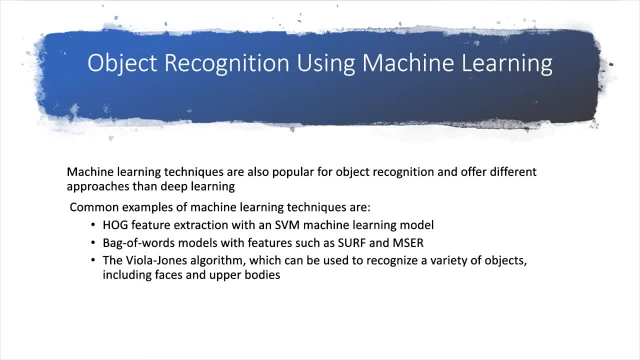 feature extraction, svm, machine learning models, the bag of word, the surf, and using these things, using these things or different algorithms, we can do object recognition and and they are less computing. so again, when we have a not like maybe the limited resource, not very good computer, not with very good hardware, 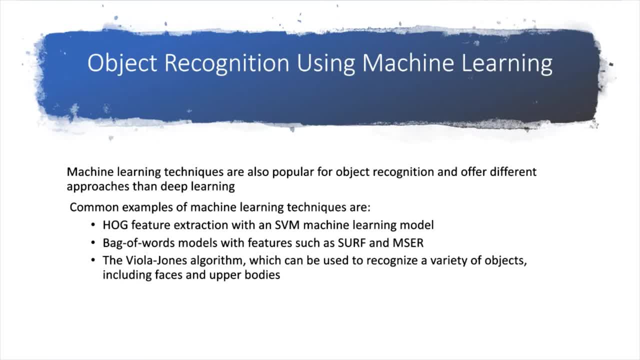 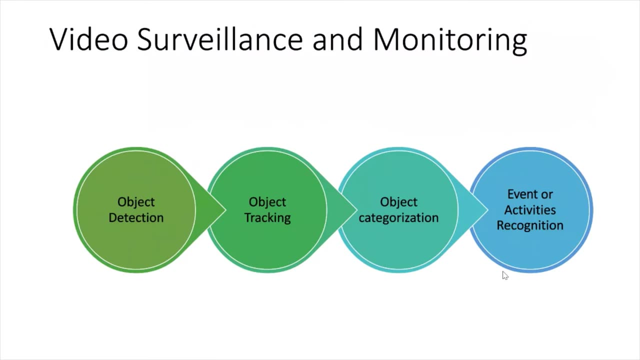 limited resource. we can choose to use this using machine learning. so the same time, deep learning is good, it gives you good results, but it's also resource hungry. you might have to train for millions of millions. uh, you know images, and then computing power. now another applications i'll talk about that's a video surveillance and monitoring. i know many of you guys are scared, or? 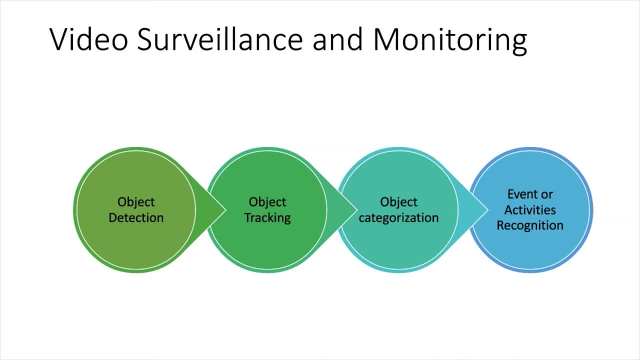 you know, seeing like, but yeah, this is one of the applications that we are using in. computer vision is one of the applications, so at the same time it is a. it is good or bad. so this machine vision or computer vision is also enabling system to surveillance. so now, if any of you like, even in 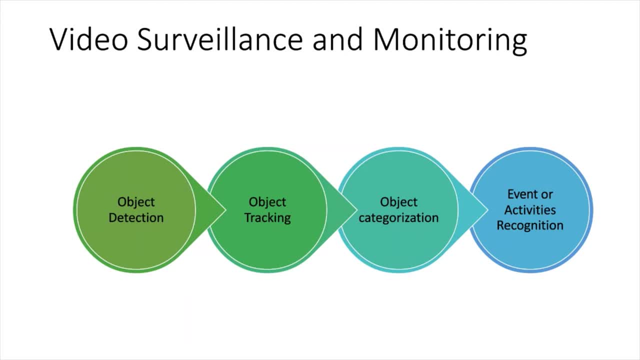 india now we have in new delhi or bangalore. you would see a lot of cctv cameras. here in united states also, we see a lot of cameras. you know and i heard and i have different like news baidu or in china. they also use this lot of traffic signal. 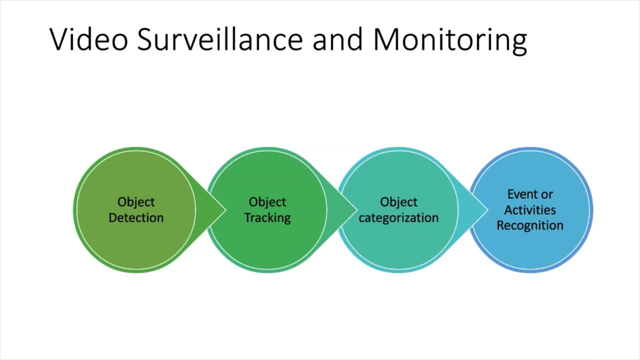 to, you know, do surveillance and monitoring. well, this lot of controversial topics. i would not like to go into that, but i'm saying it. it can go beyond right like: so, video surveillance and monitoring area, so basically in general workflow, if you see, for the video surveillance. so so using 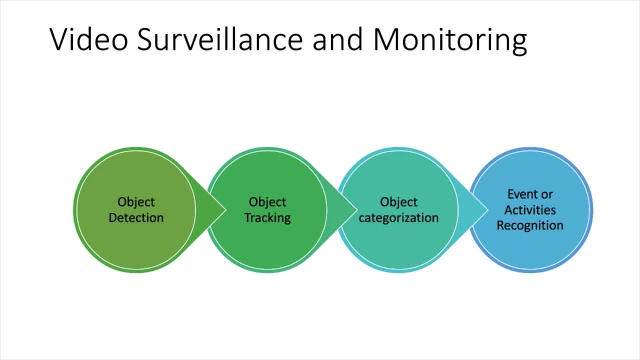 those computer vision technology, what you can do. you can identify the object, you can recognize, you can detect if some person- john- is missing or some person john is trying to hide using those- uh, you know those- traffic signal cameras. and all government can find it, they can maybe look into. okay, first they identify this is john, now now they can also track the john. 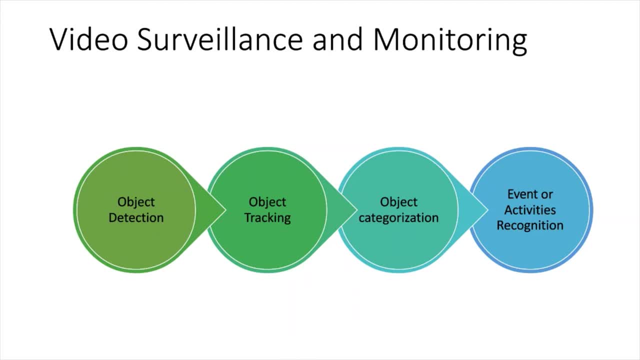 you know, that's just example i have taken. like if somebody name is john- please don't be like so it's just person x- we can also track it, object tracking. so wherever person x is going, we can track it. then we can also categorize and this is the person we can also get. 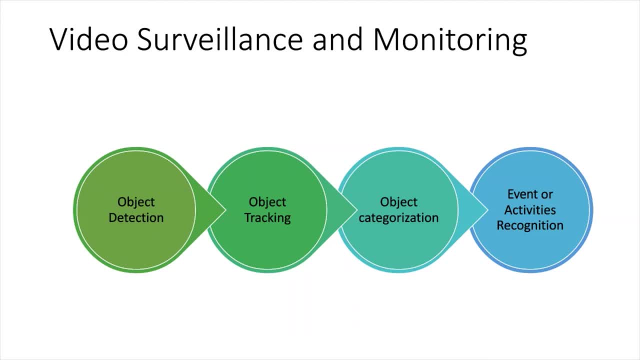 uh categorize within objects, like we say dog, cats or different labelings, then using this uh surveillance techniques or those machine vision uh technologies, you can also find out if it's the event or activities like: suppose people are protesting, right, people are their angry faces so they can understand there is some kind of protest. or people are angry, or people are circling around. 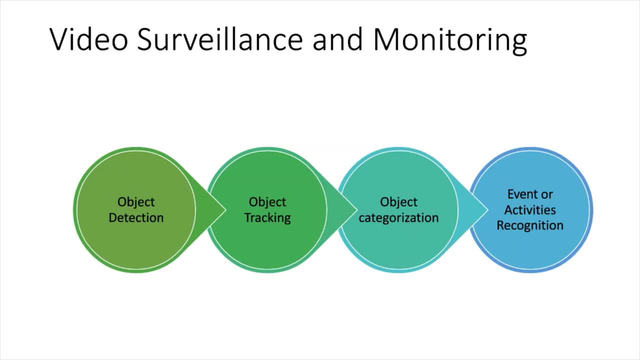 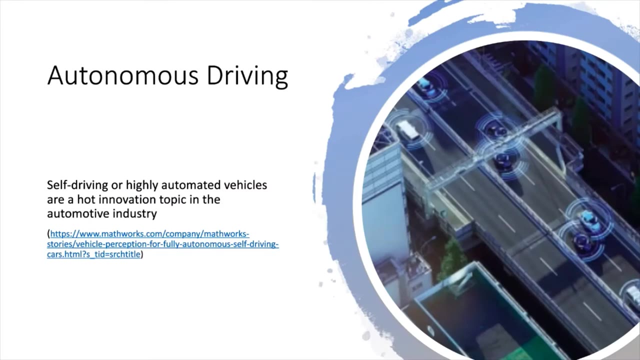 or people are running, or, or they can, they can judge, or they can they can, you know, judge the and guess the mood of the people. so there, at the same time, there are a lot of things they can be done: events or activities. they can find out what is happening. okay, so well. so i'll go to the next. 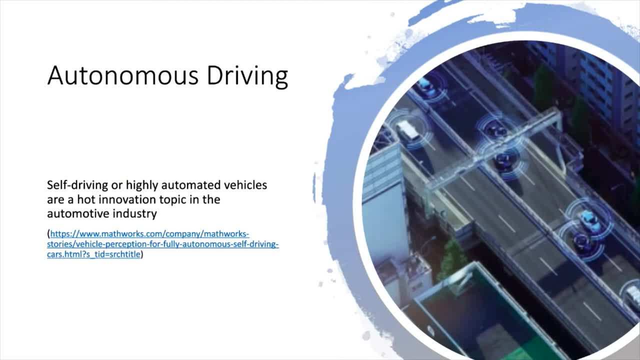 very interesting topic. so i also like this one of my uh favorite topics in the computer vision, so autonomous driving. so maybe many of you also would like to imagine, maybe you know, having a like autonomous car or some like. though it's again, it's not, it's not a norm yet. 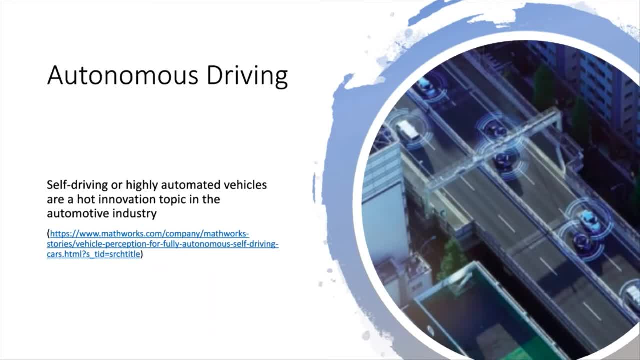 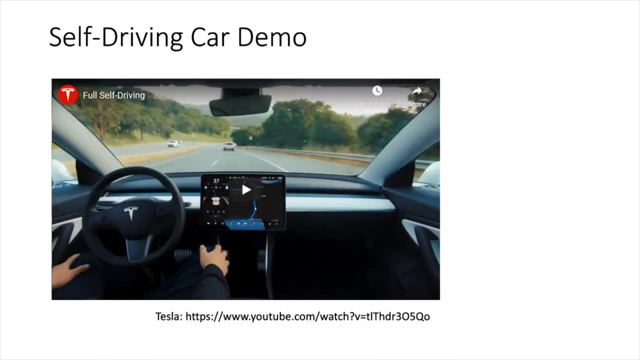 but i don't know, never say never. like it can come, maybe 10 years, 20 years, who knows? like we already have here in san francisco right some, some label. so these are very hot topics in this computer vision industry. so basically i would like to give you guys one demo here. so here in california, tesla. 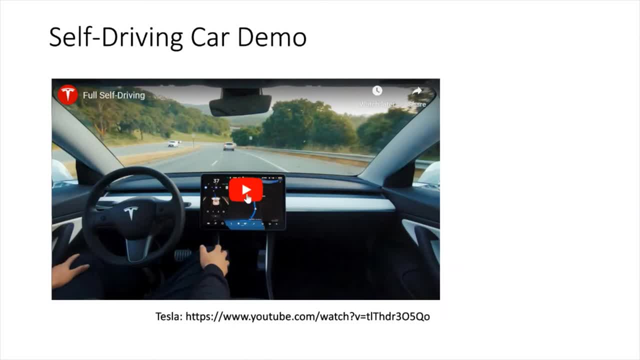 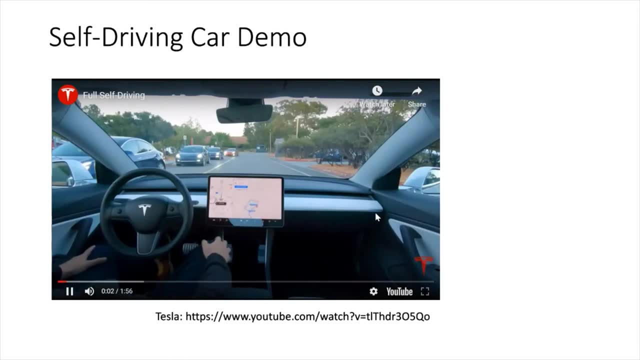 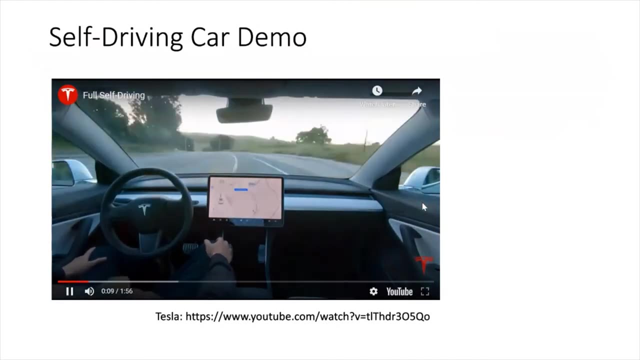 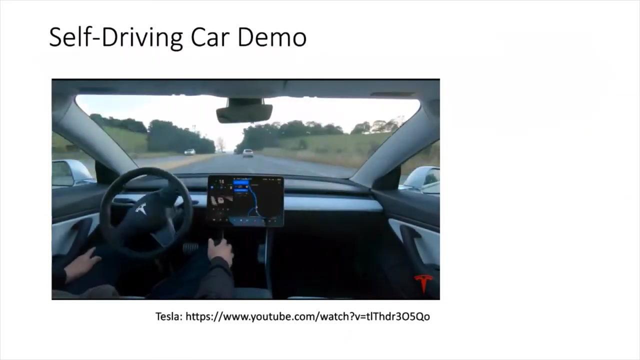 is very famous. you would have seen it. so just a second. so there is a no audio in this, uh, actually in this video, so you would not see the audio, but you see. so now, using this computer vision, how this car is enabled and you see human are still behind but it's not holding hand, and then the car is able to identify: where is that? 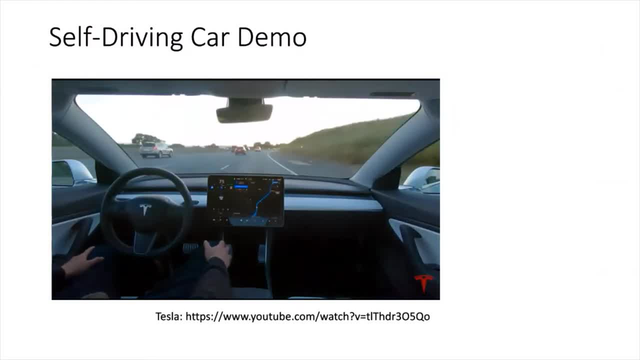 a stop signal when it has to take a turn. a lot of cars and there are. there are car driven by the human and there is autonomous car and it's taking it right lane and sometimes it has to change a lane and then then it will go also right. you see somewhere stop signals, it will go exit. 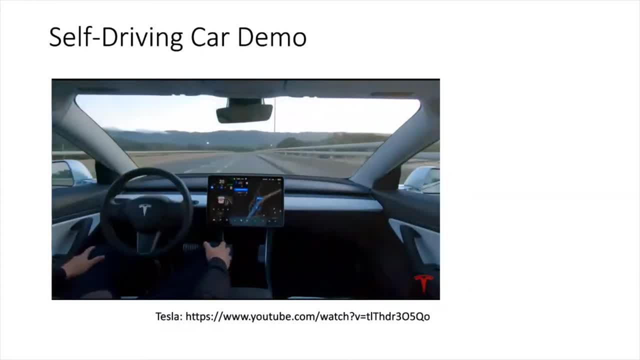 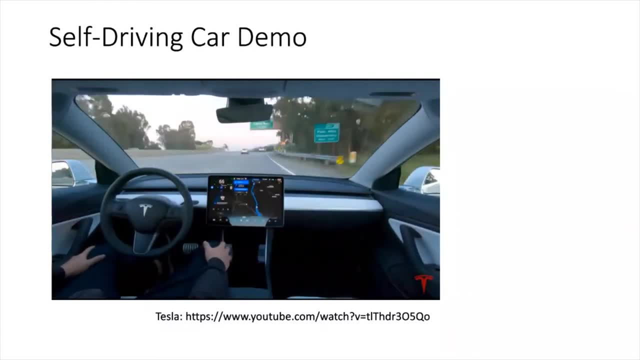 end, and if it's a green light, it will go continuously. you can try to figure it out. so, yeah, it's very cool, okay, so today i'm going to be sharing with you something very cool about what people think about a Tesla. they think that it's super cool about the future. 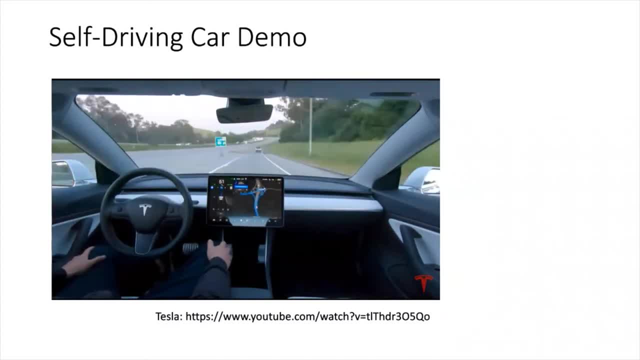 it's super cool, because it's very cool that someone is going to sell a car to a bunch of people like what would they do? it's very cool. so i would like to share my own personal experience, like i've been with the tesla, you know, uh, and it's very cool. sometimes that is scary, but it's. very cool and it's also completely not permissible like you have to still behind the wheel, like you don't have to hold the wheel but you have to be on the seat. so if anything happens you can take control. so they allow you. but you know, if you're a customer and you are driving a car, you could give it to yourahce as you want, but the other is that car is not here. 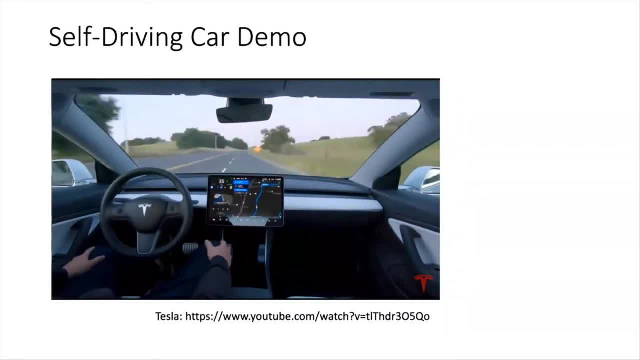 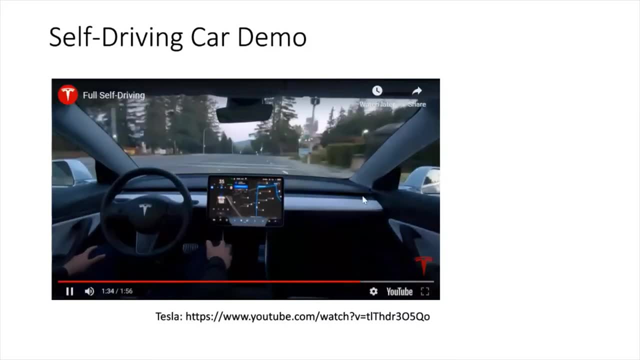 But they are pioneer. they are very much ahead right now. So there are different companies that are working on this self-driving car demo, So maybe I think you would have got some idea. I can go for the next section. So you see, there is stop signals. they stop it. 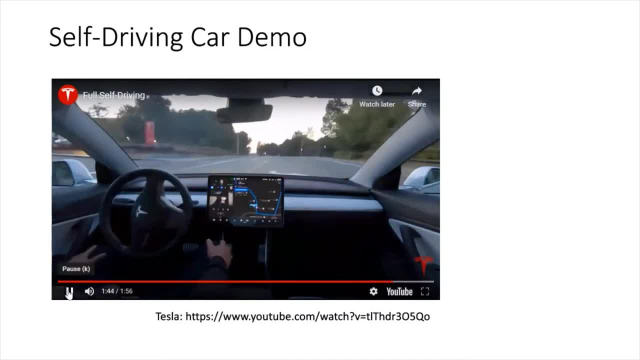 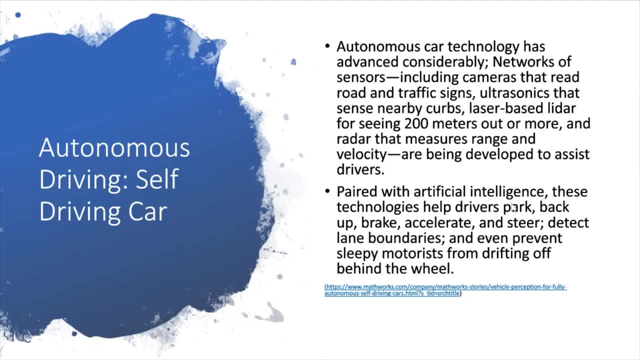 So now, what enables? So if you talk about what enables this autonomous car, what enables how they see it, and there is a link. So now, if you see now autonomous car technology, but how this car can see, what empower them to do this? 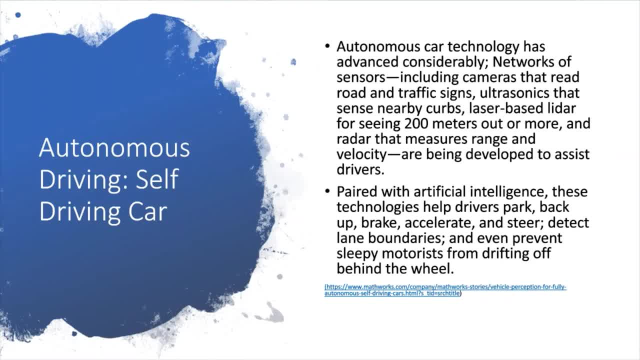 So they have a lot of again cameras. they have a lot of sensors. So now what these sensors and what these cameras do? So these cameras empower the car to read about where is the traffic lights, where is the signal, and they're different. 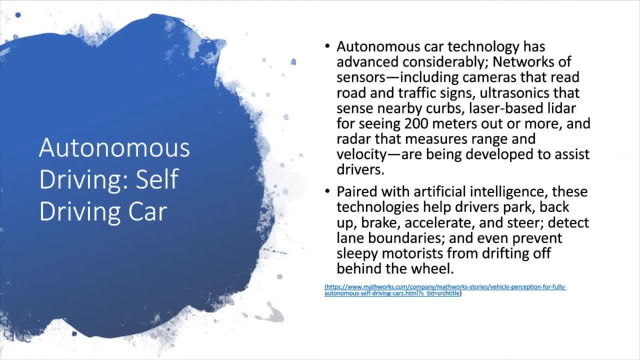 They're ultrasonics, they're LIDAR, they're laser-based LIDAR technology. They can see beyond 200 meters. So they have a lot of these sensors And now, using these sensors, we also have to process this data very fast. 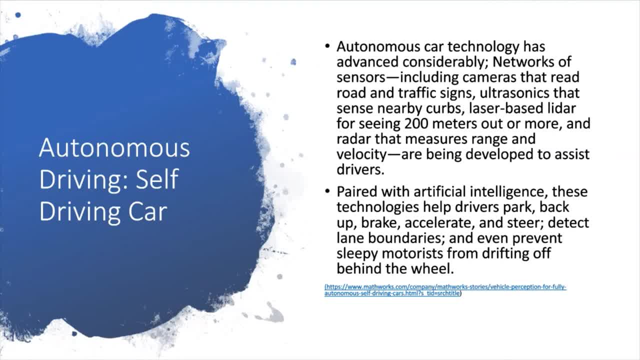 Imagine if you take a decision late. you have to. you are about to hit, like you know, some objects, but the process is delayed, So you were already made to accident. So that's why it's very critical, The same time, the accuracy. 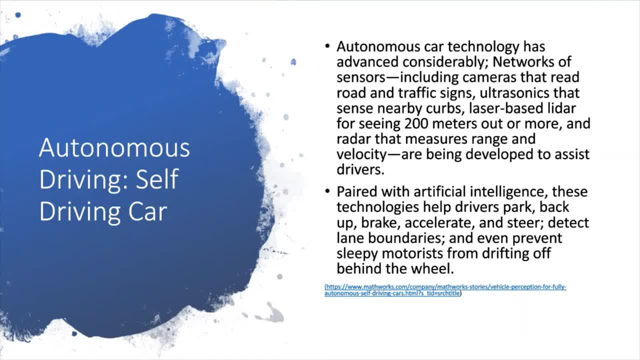 and then your computation power. That's why there are a lot of technologies and there's still a lot of research is going on. So now it's again those paired with those, AI and computer vision, And right now we are also using 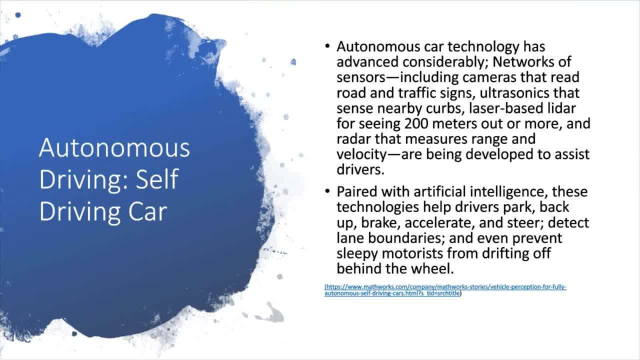 in India also have a lot of, I guess, these facilities nowadays In United States also we have these. So we also gave this autonomous feature in partial manner. So partial manner what we, they enable us, you know the automatically. 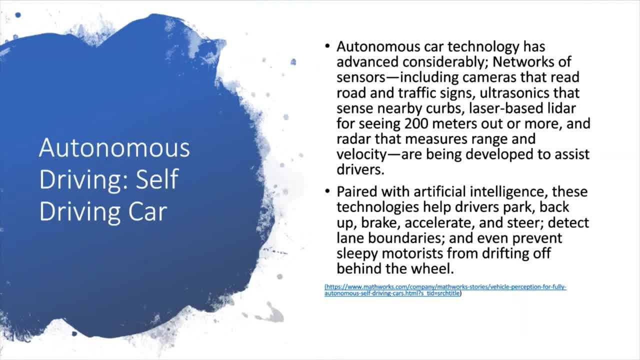 they give us lane detection, lane boundaries. If somebody is a sleepy driver or somebody drunk driver or something, the car will assist you. Like you are not driving straight, They're gonna give you a response back They. the car is now helping you to find a blind detection. 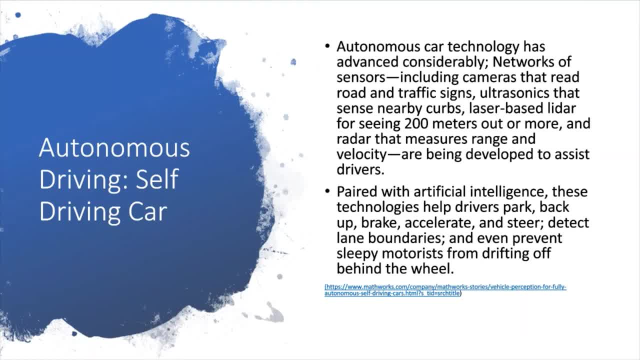 you know, or you're changing the lane or if there is also collision prevention options are given. it is not guaranteed, but when the car sense it is about to collide, they will have automatic brake. There are a lot of features coming. 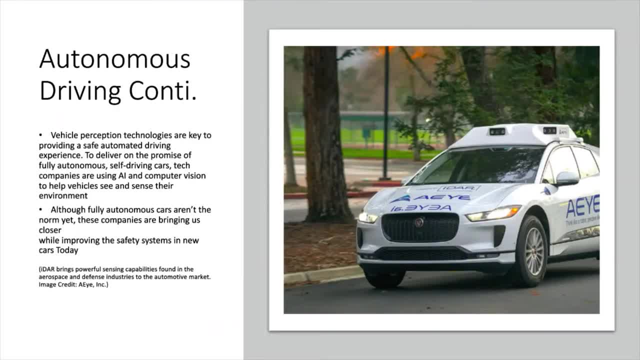 but they're coming into the part. So now, like one of the, I have taken from one source called AI INC, So they're AI INC. this car basically has this. they are also working on those lighter technologies And they would say: 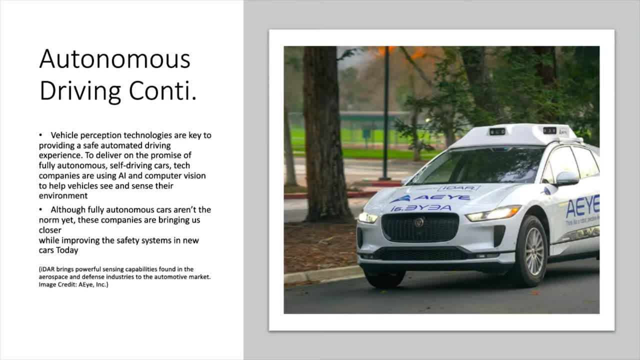 yeah, fully autonomous car aren't the norm yet, but these companies are all are bringing, they are working very much into this area. Now I guess different companies, the Uber, now people said Uber, right, Uber also working on those automated car. 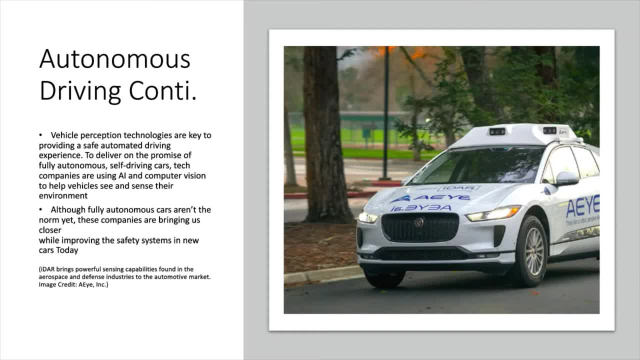 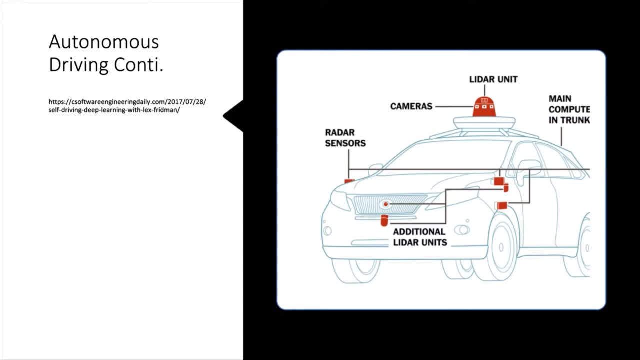 like Lyft also working. Then many companies in San Francisco are working in this automated car. So again this last one in the automated car section. So we'll see what are different components, right? So this in the car you would see this: lighter units. 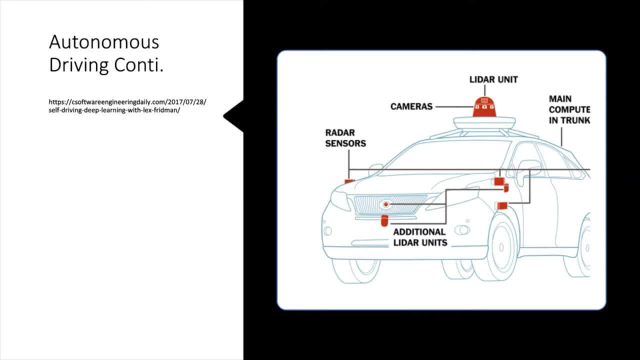 So on the top, like they are also actually the costly sensor, There are different cameras and the camera see in 2D and 3Ds. There are a lot of point cloud computation and different later section I'm gonna talk about. There are sensors, there are additional lighter units. 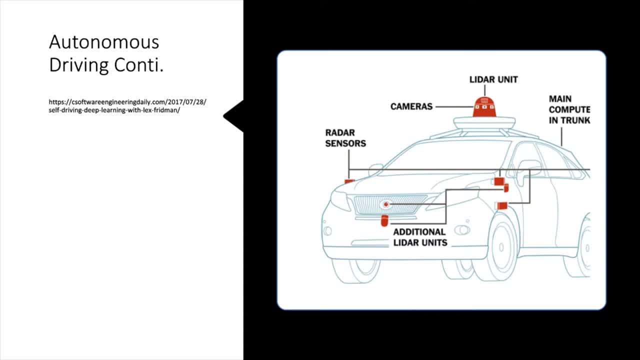 and there and then the back they can have them make main computer in trunk, So every data has to go to some computing process And then it's more like a brain, like we are seeing and taking input from different sensors, and then like a brain in the software. 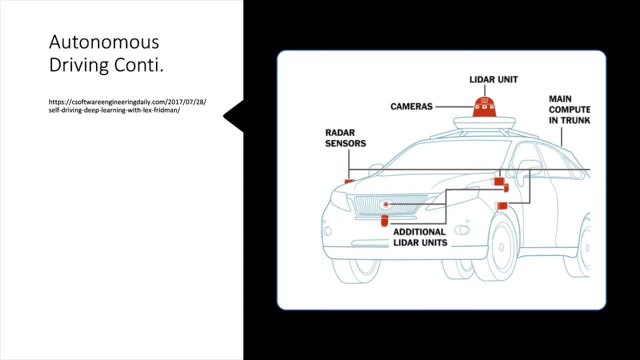 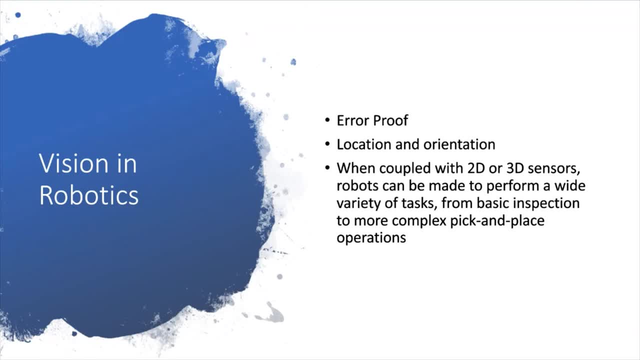 like a main computer. It has to process this data. Now we'll go back to the again. there was the general applications. Now we would see vision in robotics. So, like in general vision in robotics, like what our applications are, Angle of vision is. 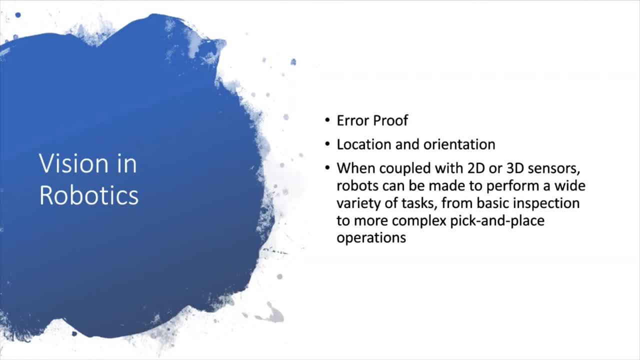 applications. if you just focus to the robotics area now, like if you use it, so error proof. so again, if, if the task is given by the human, there are human errors, there are chances like welding error or something or painting error and all. but if you do this task with the robot, there are less. 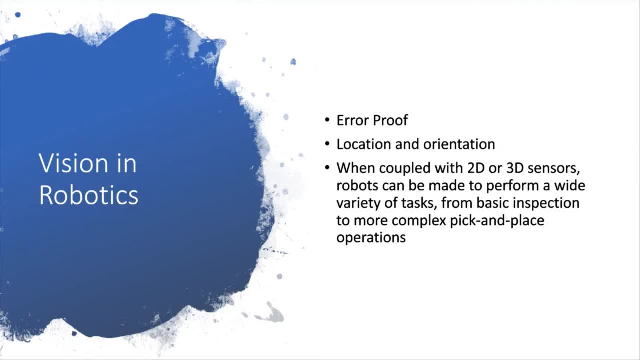 chances of the error. then again, robot has to pick and place something. so using the vision we can have this location and orientation. so when coupled with 2d or 3d sensor, the robot can me to perform very, very different complex tasks, like suppose i was talking about. i would have. 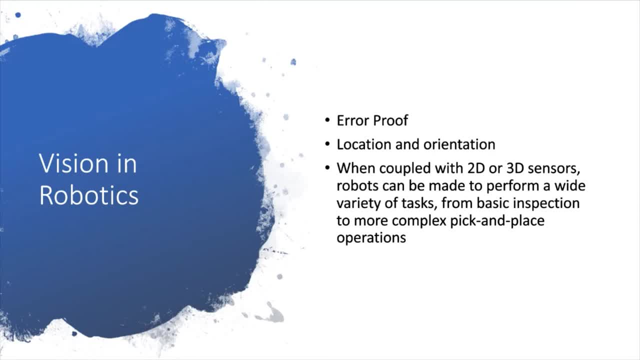 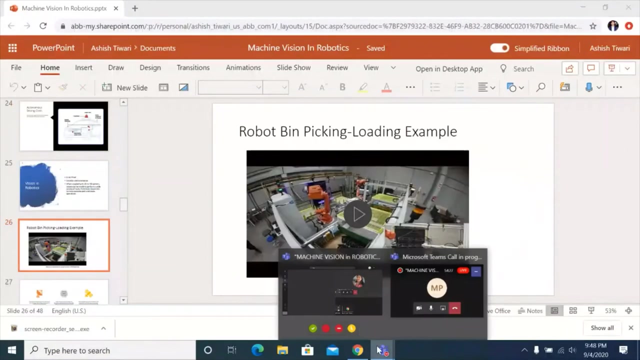 some video, i guess for this. our company robot, like some applications like pick and place. the robot has to pick something from the bin and then place and then into the warehouses or factories there are conveyor belt and like amazon warehouses or anywhere like you can name it- different applications. so now in the robot section. so let me see if i have enabled the. 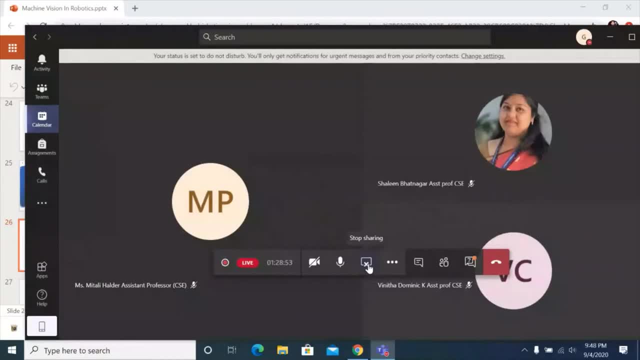 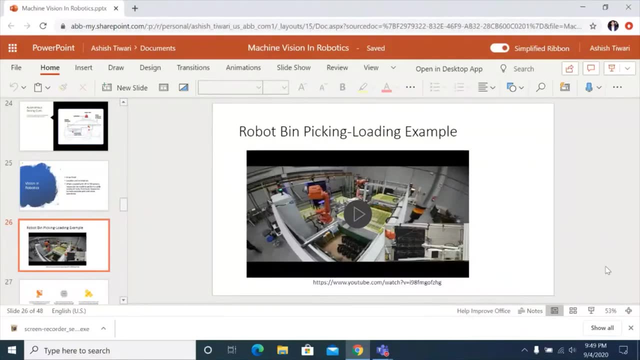 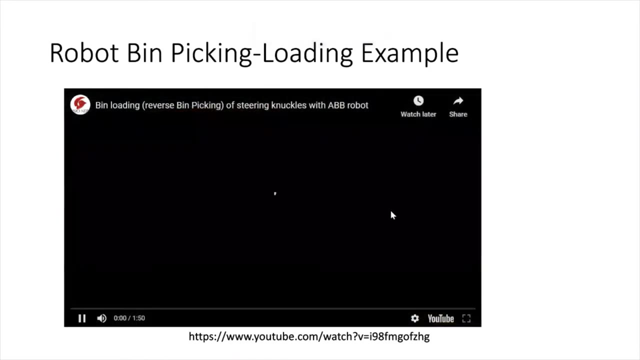 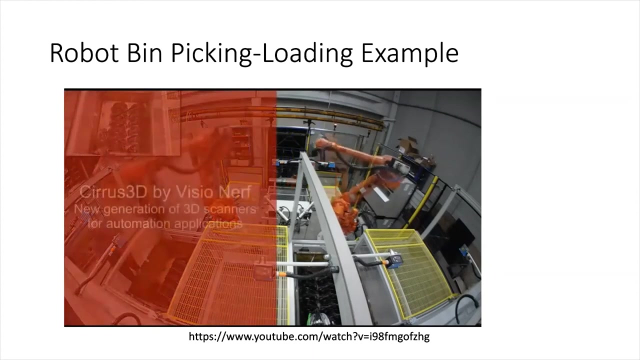 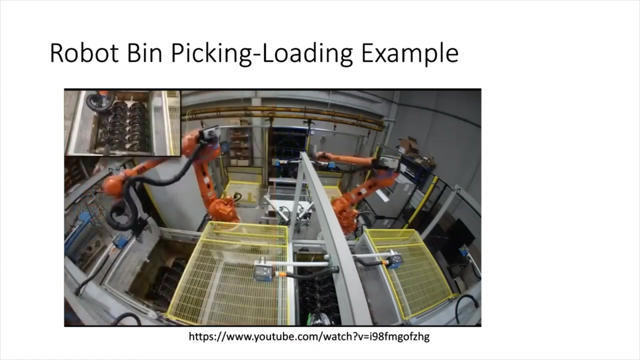 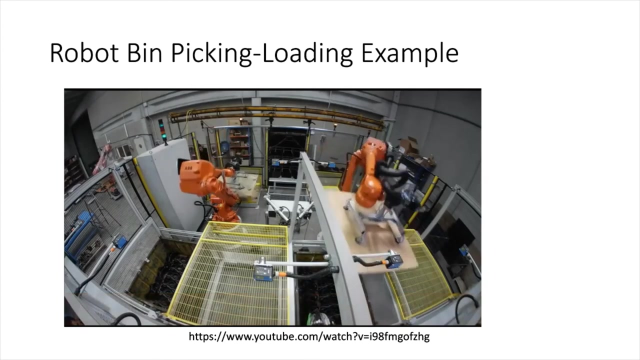 just a second. you guys should see, i guess, the audio. so now this is the robot bin picking application. this has the sound as well, so you should see the sound. it's basically a bb robot so you can pick up the sound you want, and then you can use the sound to pick up the sound. 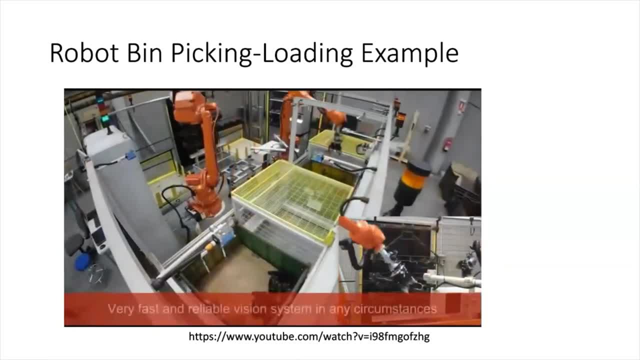 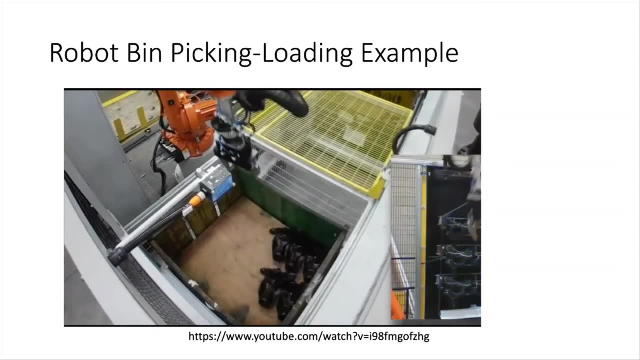 you want. so right now i'm turning this on and let's go to the sound section. so if you want to start the sound in this video for the first time, you can start the sound in this video, but you would have to use voice over, which i'm going to go and turn it off first. so 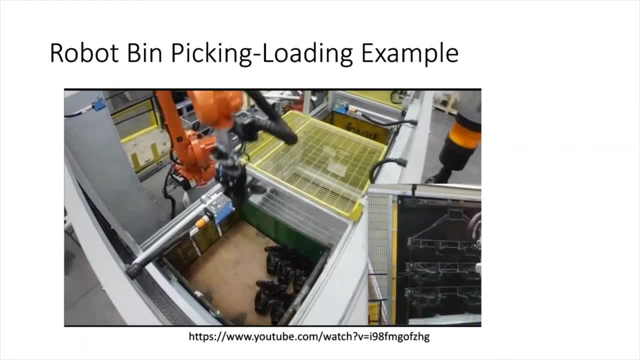 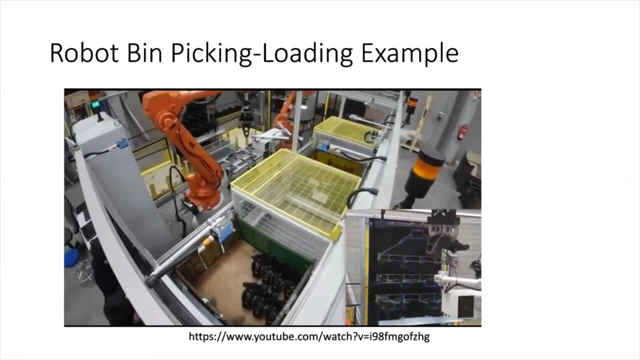 all you have to do is turn off the volume and turn it off so that you can hear all the sounds in your home screen, and when we can't hear, you know you're working on something like a computer, which is a computer that you're using right now. we're going to go ahead and 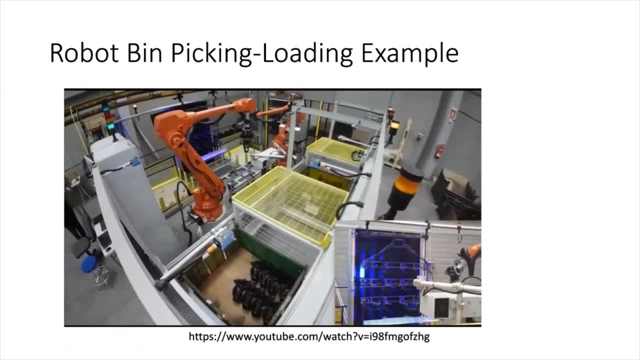 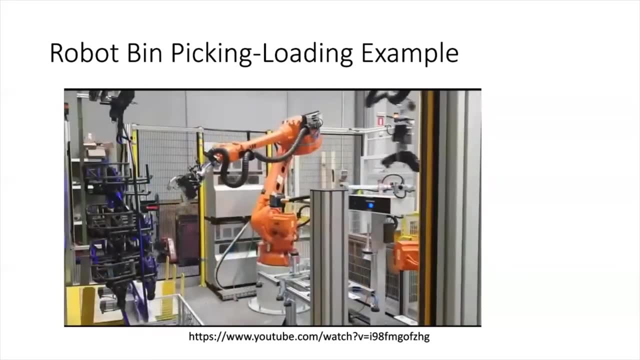 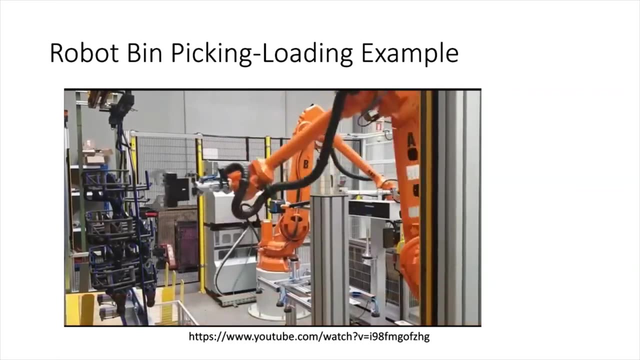 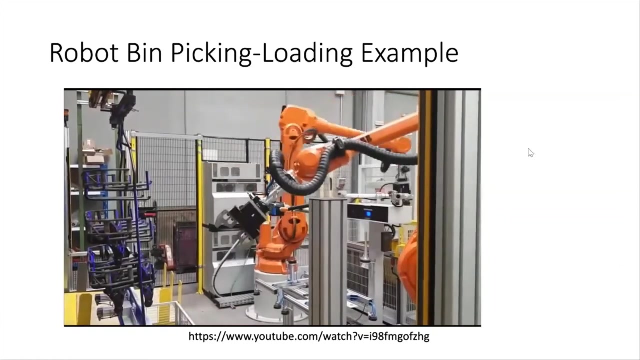 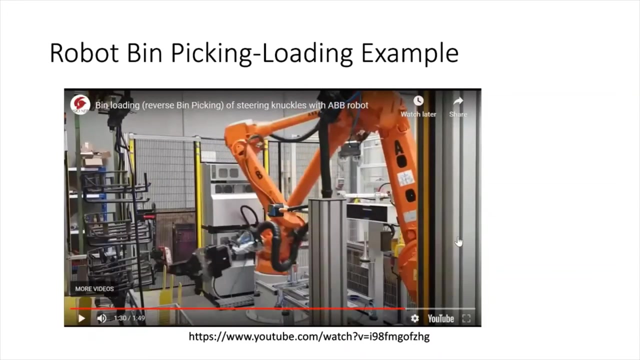 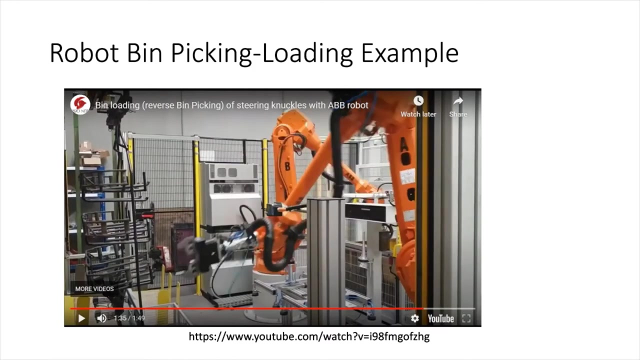 All right. So basically the idea. maybe this much would have given some idea, So we would also have to cover different. So here I would like to say so: if you can see in the videos, the robot is trying to pick up. it's the reverse bin picking, basically, And we are loading the bin We are taking. we are loading the bin We are taking. So what empowers these robots? So you would see some camera on the top that is taking a picture. There will be a flash in between, So someone has to see it, right Then only it could be enabled. 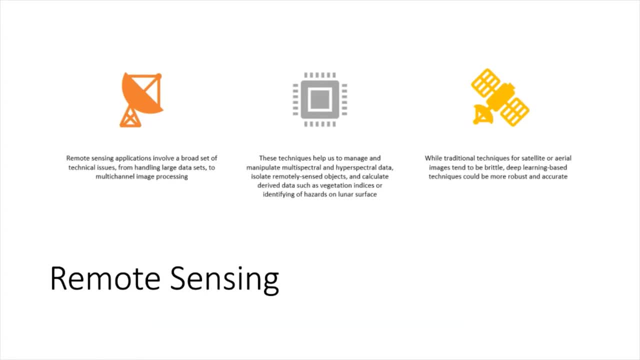 So now we go to the next section Now, different application, Now in a remote sensing. you would have seen, these days we have a lot of drones into the picture in US, also in China or every country these days, And the computer vision also can be used in the remote sensing applications, right, And also maybe the satellites data are coming or we are going to the Mars or going to the moon and we have to, you know, like process so many pictures like high, so that the 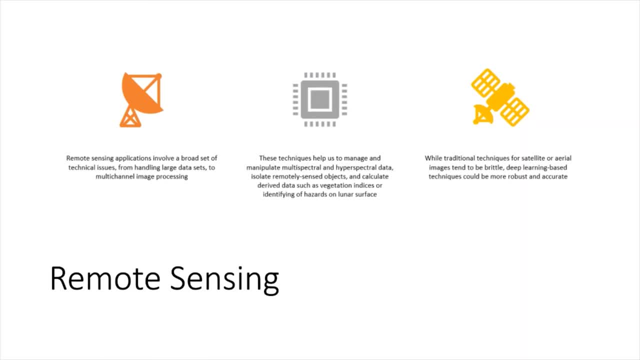 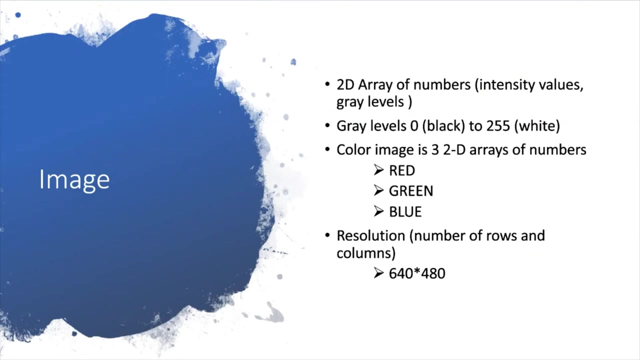 vision also would be helpful there. So again, I would not go more detail into this. but, like you know, conventional technology was not that you know enough or giving the good results. but using a computer vision or deep learning we can have a more robust and accurate results. So I'll go to the different section. So now, if you guys would like to have a career or would like to have a more interest into the computer vision or vision in robotics, So you would like to have- you would have to. 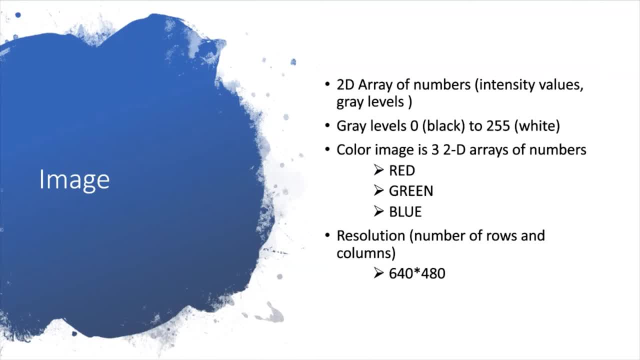 know the basic things about the vision. So what enables it? So, basically, the image, So the basic elements of the computer vision or the machine vision. these are the image. So what are the image? right, We say image tells everything. So, without saying a word, we can see things, we can guess things from the image. So image is nothing but it's just a 2D array of numbers and these numbers represent their intensities, values, their gray labels. So now we have, we say, zero is the black and 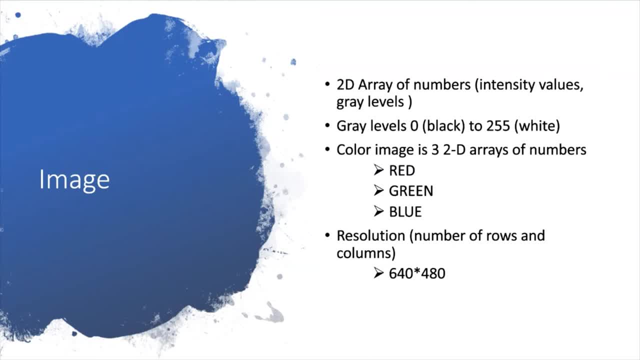 255 is the white, So they vary from zero to 255 and in between they will create different colors. So now the color image. color image is basically the three two-dimensional array. So each two-dimensional array, one is for red, another for green and RGB, basically So the red, green and blue, the combination of these three channels, we make a color image. Now what is resolution in image? So if you say number of rows and number of columns, these are called the 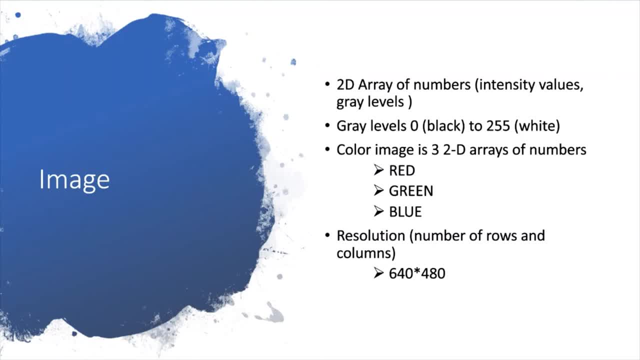 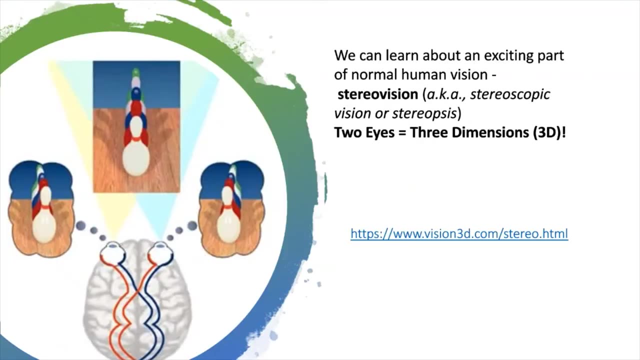 resolutions. So we say now this much megapixels in the picture right is the camera. So basically that's the resolution. So right now we have 640 by 480. We can have also 1280 or something. Previously it was less resolution. These days now, images are, you know, coming with high resolutions. Now the another good thing I want to talk about, when you know I was passionate about, if I talk to like I was working in a Bangalore, you know, as a software engineer, and then I was passionate, or you know, to go to the research. 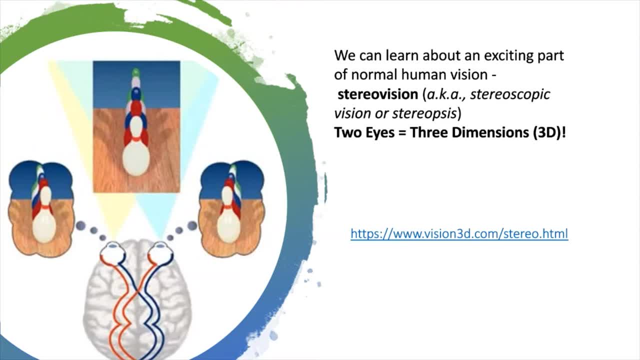 and I came for my master's and then I went to machine vision lab. So then, the first thing: it's passionate me. you know how things happen and where this stereo vision concept comes, why I was relating that story to here. So I had this, you know, lesson in my class, So I would like to share with you guys, you know. So, basically the human, we have a two eyes, right, And these two eyes is basically the three dimension and they call it like it's a human vision. 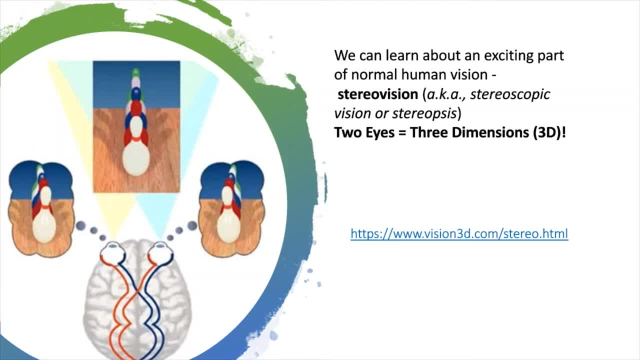 is actually very, very complex. We just say it's a simple, but we say like stereo vision, stereoscopic vision or stereoscopic. So what happened? if you see in this picture? so in the behind we have a brain and thanks to God, we have our eyes side by side, not like a horse, like horses are very on the side. So if you can even do one exercise, so if you guys are seeing this image, our each eyes take a picture differently. Our left 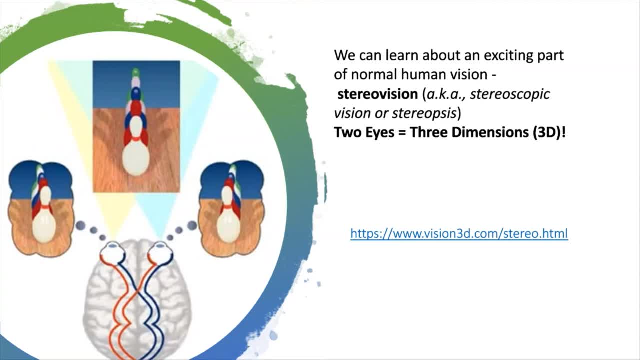 eyes see most of the left portion of the object. Suppose if you guys go to the bowling and all. So if you see the left eyes is taking most of the left side of the picture, if you close, if you can do even one exercise, you can have a. you know, cover your right eye and see the, your finger or some object in front of you. then you would see a different image, like seeing from the one eye. Then then, after this, you cover your left eye and then you see same thing with your right eyes. 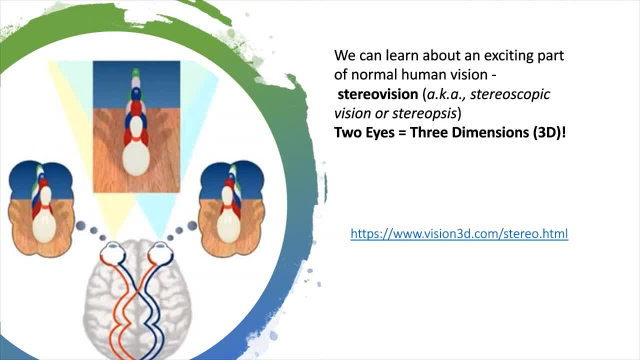 So you would see the object in like the different views. So now what happens? So these two different views taken by these two different eye left and right, Now both image separately sent to our brain. like in our brain in the back there is some processing units that will process these both images. It will combine their differences and it will make one image, buying, making that one image. The brain will guess it right How much is. 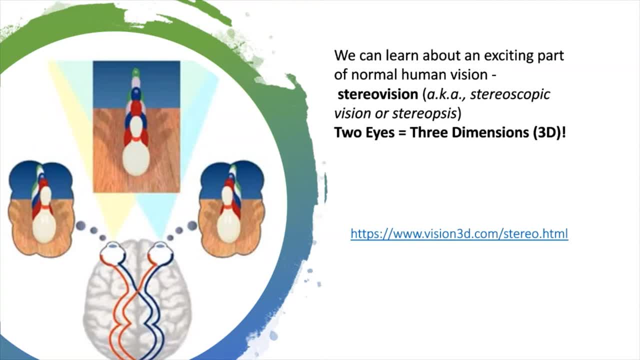 the width or orientation of these objects. By this, if you have to grab some glass or some cup, you know how much your finger has to go like otherwise you see things in 2D. You can guess someone is very thin or someone is having, like you know, dimension also you can guess it. So this is very fascinating And this is the motivation for the computer vision, This is the motivation for the cameras. All these camera technologies are basically based on. 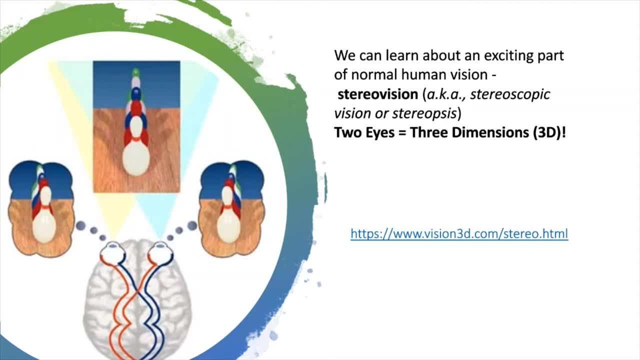 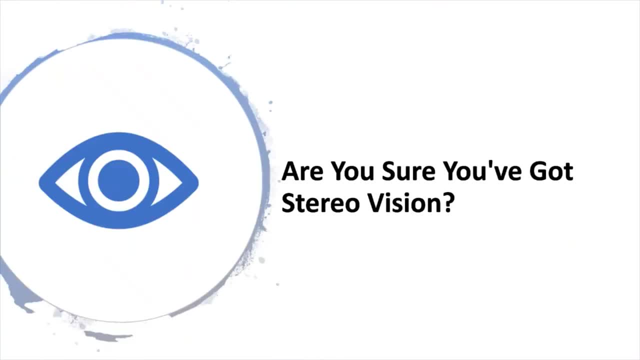 our human eyes. So later I have another slides for this. This is the exercise you can see. You can go to this link and they have another funny games also and very, very good games Now. so by seeing this, are you guys sure you have got a stereo vision? 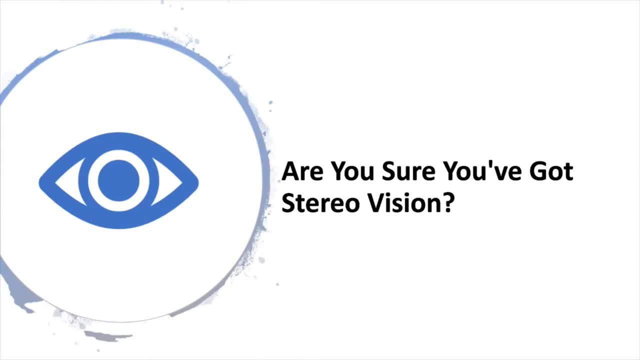 I think every one of us got it, Sometimes knowingly, unknowingly, we don't know. but you can see, some people are very good at it Seeing, you know those 3D movies or you know something, and some people have less. but you can do this exercise. 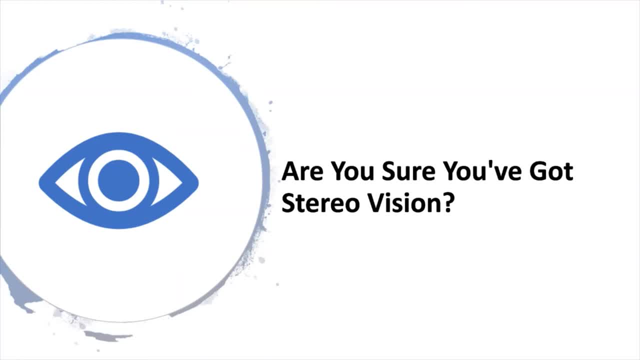 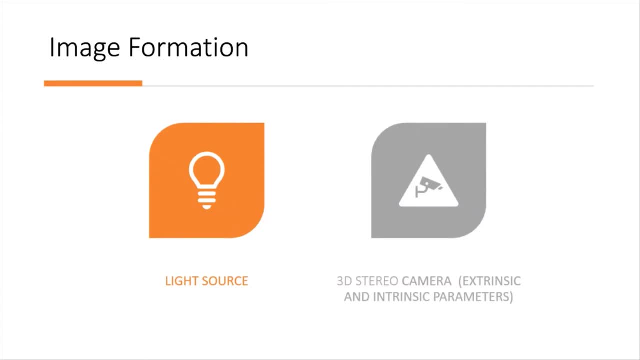 You would find out. So we have stereo vision now. So I would. so I would go to the different topics called image formation and computer vision. So the what are important factors for the image formation- So there is one- is light. Light is very much important here, So light intensity. 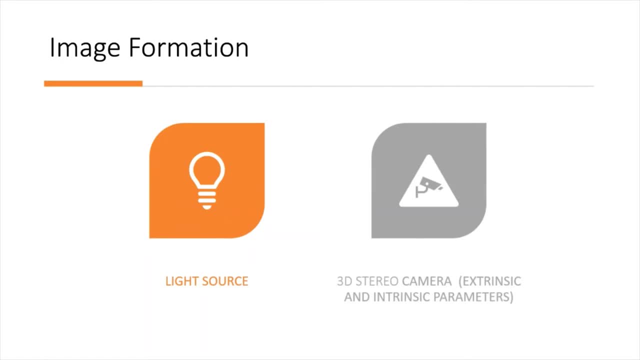 There are. you know what is the label. We can also have a unit for the light, So the light. And then here I'm assuming, because I'm mostly talking about 3D, 3D vision, So here like 3d stereo camera. so there is like extensive or intrinsic parameters. uh, you don't have to worry. 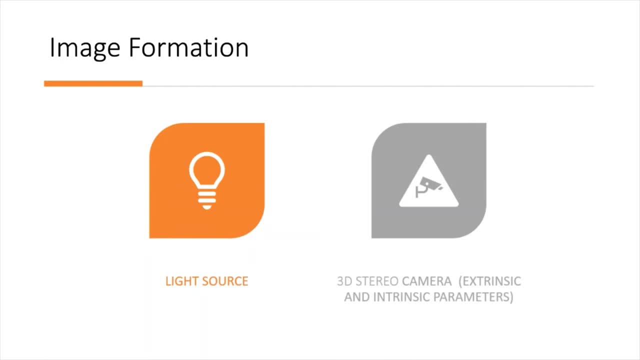 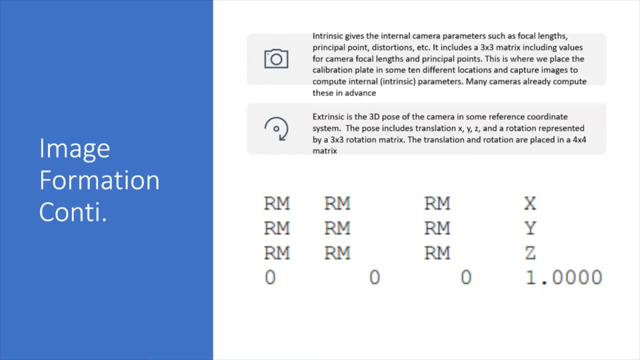 right now, because they might be the new word for you guys, i'm going to talk a little bit about it. so so, basically, image formation happen using these two information: light source and their extrinsic, intrinsic information. now, if we say the intrinsic, basically means is internal to camera. so 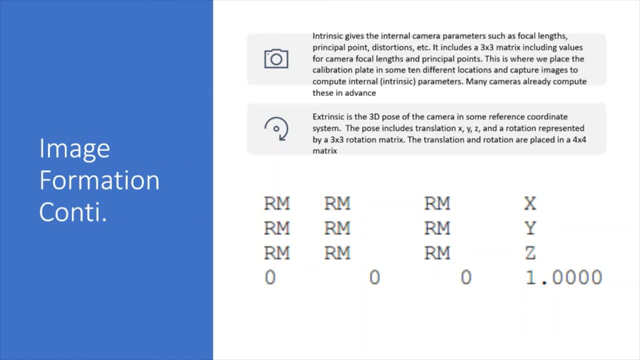 now we happen right. camera can have an error. so it's basically: uh, we have the values for you know, camera, focal length and their principal points, and they can have some errors. so some examples: we can place one objects in 10 different place and take up pictures from the same camera and then we can. 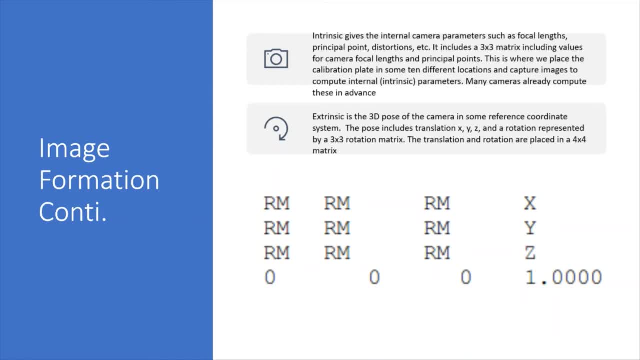 find out where is the gap, where is the accuracy problem. so these are the intrinsic parameters that give their, how much offset we have to give for getting a good result. now the second parameter, called extrinsics. now, as by the name, extrinsic means external or outer world. so, and then in the later slide i'm going to talk about, it's called you know, 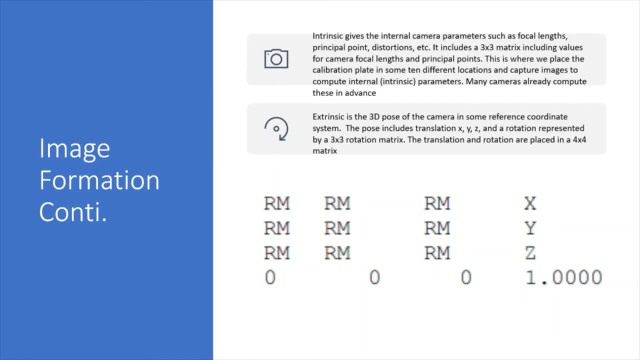 uh, the coordinate system. so basically the extrinsics are into a helpful in the world coordinate. so if you are like we all are, some, somebody are sitting in a room, right, so you can see in your room, you can have, you know the width, your, uh, your width, height and your length, so like, 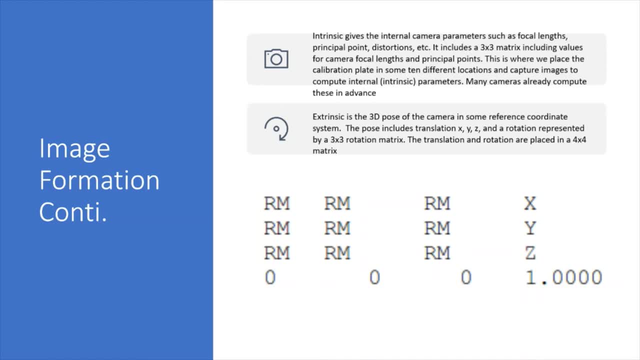 if you divide things in xyz, your your wall. you can imagine, like you know, we have a three dimension so we can have all the things. so now, similarly, so we have something into camera coordinates. uh, you don't have to worry about again, i'm gonna give maybe some examples and then how this thing. 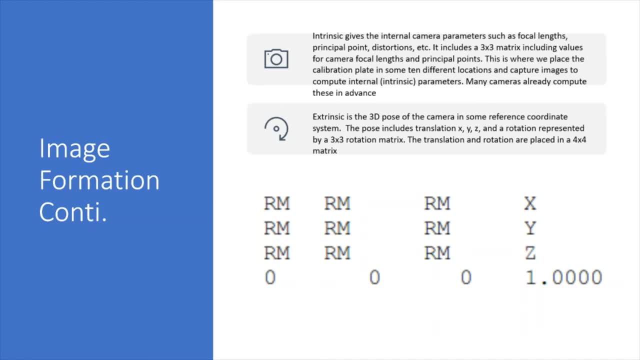 will happen in the world coordinate or some robot coordinate system. so for that information we need this extrinsic parameter. they are basically represented by uh, four by four metrics, or among that we have a three by three rotation matrix and rotation and translation. again i'm going to talk. 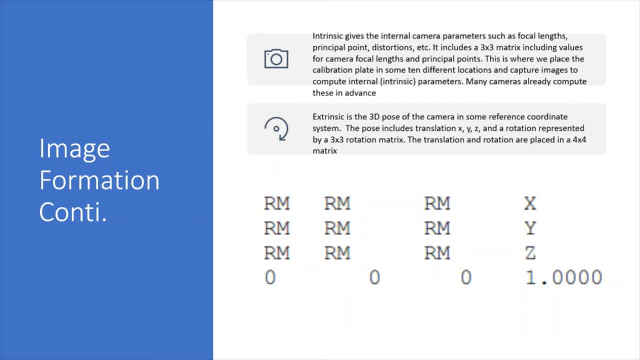 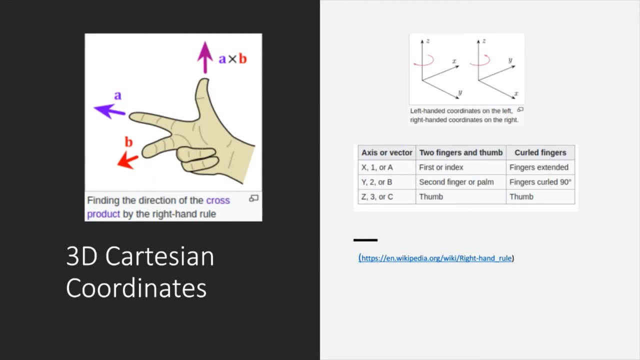 about that in a minute. so we have a three by three rotation matrix, and then rotation means what is their angle or their orientation, and all so now if you see another information in the robotics, so we follow here basically right hand rule. so if each one of you guys are seeing maybe the 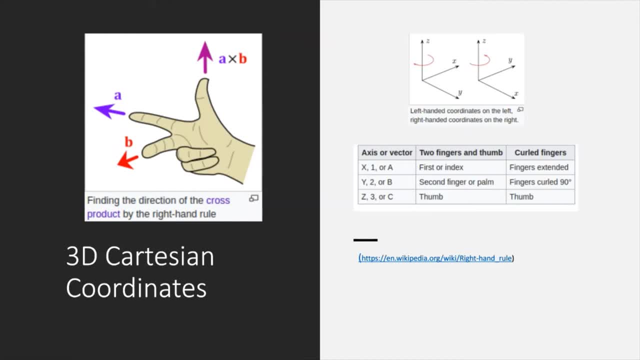 presentation. you can have this little exercise. if you have your right hand. you can just have the your hand, like in the image. so if your thumb basically is pointing to the upside and that actually z axis, that's a cross b of the two vectors. if we say a and b is a vector, so the 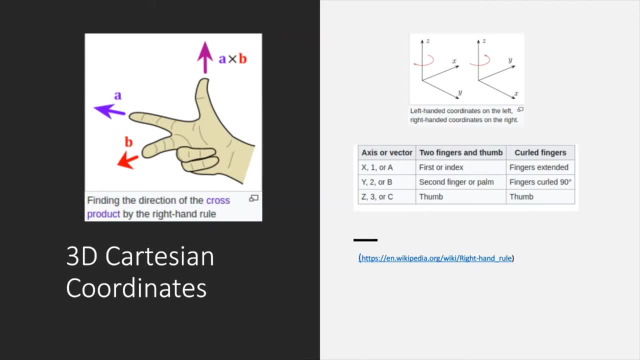 z basically is the multiplication of those two vectors. and your first finger is pointing to generally x direction, then we call it vector term is a, and then your second finger or palm, basically into that y direction. that is basically the uh v in the vector terminology. so we follow in this. 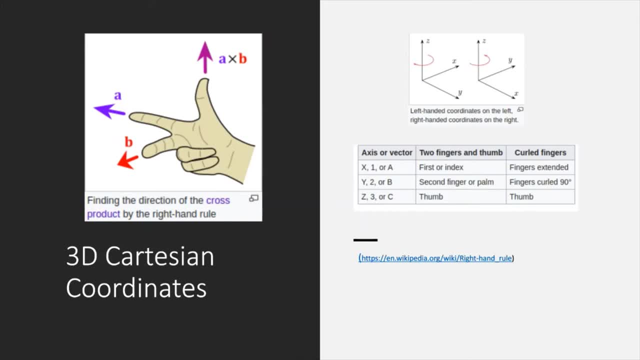 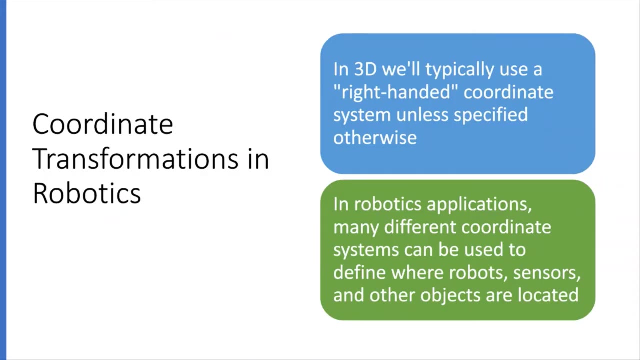 robotics until, unless it is told by default, we follow right hand system. all these researchers, this is more like a right hand rule: three cartesian coordinates. in the left hand it will be like different. so now this is kind of a coordinate transformation robotics. so, robotics as i told, by default we have our right-handed coordinates. 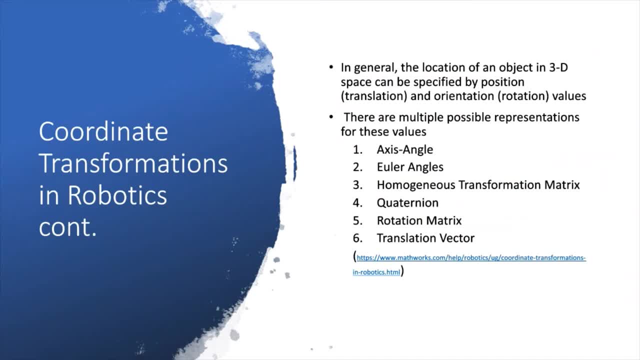 now coordinate transformation and robotics continue. so how we can represent these coordinates. so now, um like as you like, as you have seen in the previous slides, i was talking about translation and rotation. so basically, if some point like into some world coordinator robot coordinate system, that point can be represented by x, y, z. so that is actually specified by position and that we call it. 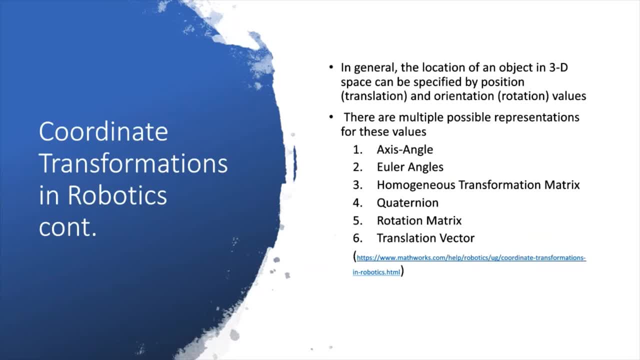 translation. so now robot has to move how much from its base position to reach to that object. so suppose it has to reach this much in x direction, this much in y direction, this much in z direction to reach and just pinpoint to that object. now the orientation. orientation basically is the rotation, so object can be on that particular point, but it could be. 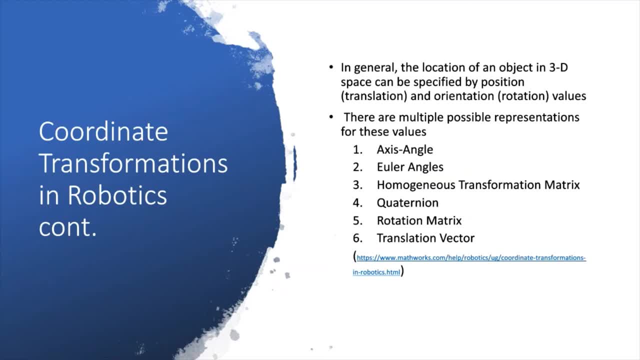 tilted right, it could have some angle: 90 degree, 45 degrees. so this is basically the rotation. so it's very fascinating if you have to hold something, how, if you have to hold something by our hand cup right, you have to tilt your hand, or how much you have to reach your eyes. giving this information to 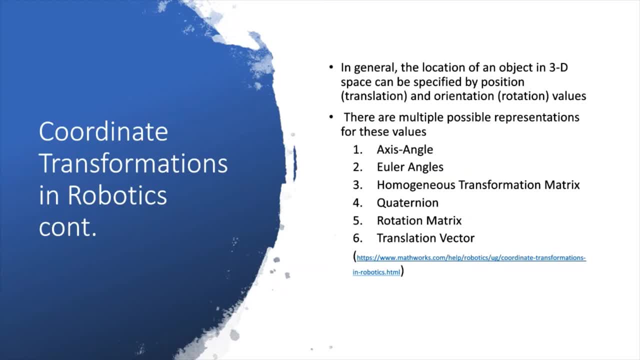 the brain. this object is this much far and you have to reach this much and you know the distance, where is your hand and how much your hand has to move. this similar manner happen in robot. it's. it's very much the same thing. so now the different representation of these values. 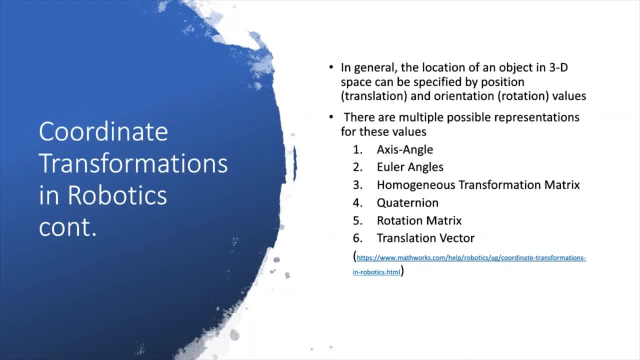 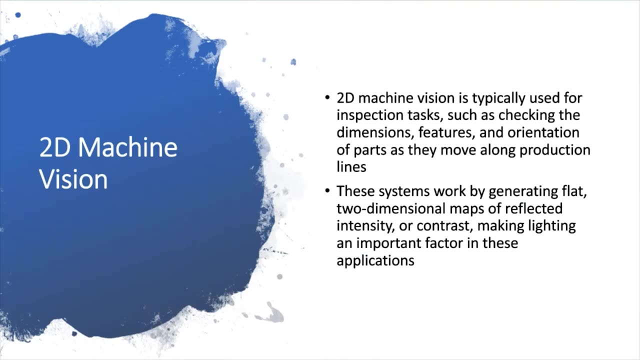 uh, you can again, uh, read more about these. uh, there are axis angle, euler angles, a homogeneous transformation matrix, cotonians, rotation matrix, translation vectors. these are more. if you would like to understand more now, if you say now i'll go to the different topics because, uh, there's like 2d. 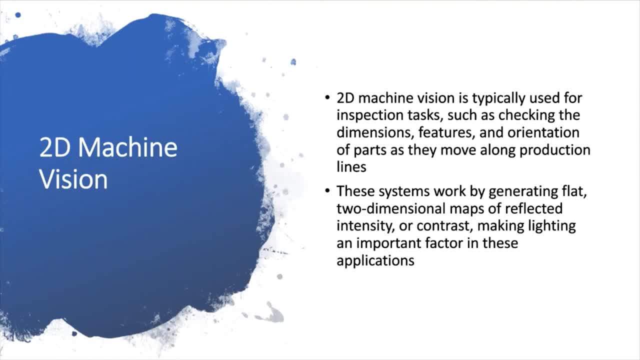 machine vision. so now the vision can be divided again in 2d machine vision and 3d machine vision. so now what is 2d? so so again in two dimensional, basically x and y. so, like in mathematics, we have generally right. so if you see the, the basic example, here is the funny part. if many of you 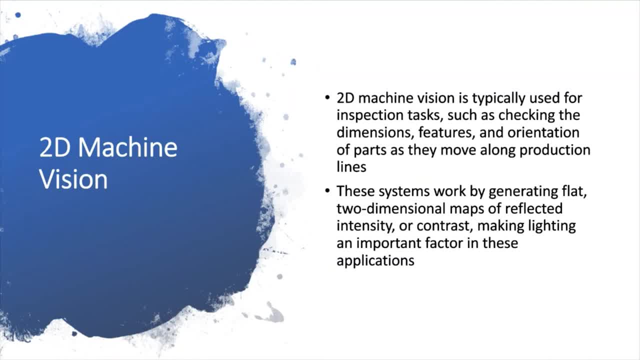 guys would have been into the plane right. if you go in aeroplane and if you too much height from the top, you see what are you able to figure it out? any tower or something. mostly we think see things in a flat right, so everything is a flat. so representing things in a flat and 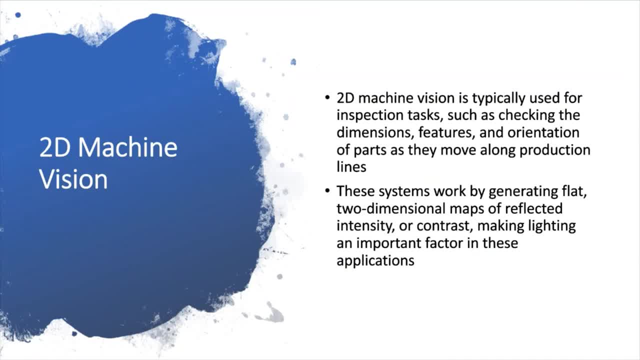 we have basically represent things in x and y. so this is also could be advantages and disadvantages of the 2d things. so basically, uh, giving those flat information, this x and y, this 2d machine vision we can use in inspection task. we can also have here detection and all. but it has its own limitations. 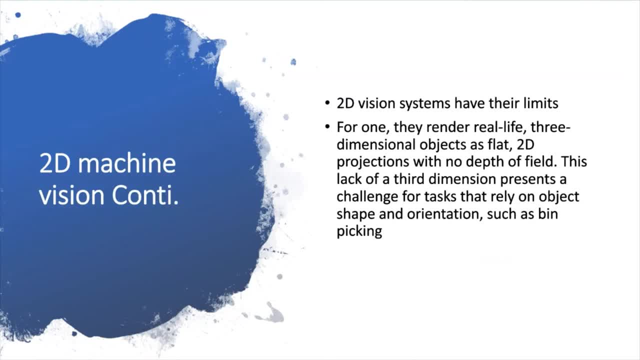 so now? so what is applications? so 2d vision, uh, two divisions, can be again used into that uh inspection task if you have to find out, uh, uh, suppose, uh, this, some paint is done or not, or or some other information. they are basic, their depth is not required right the node, because it doesn't. 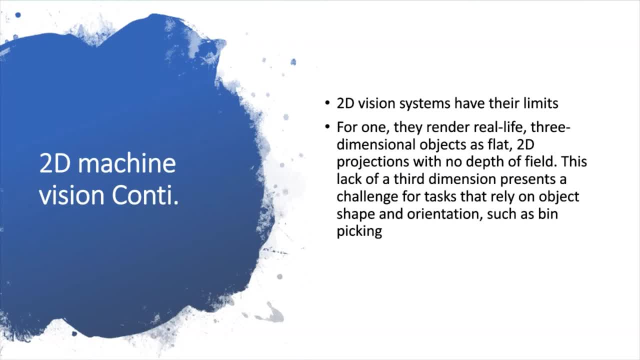 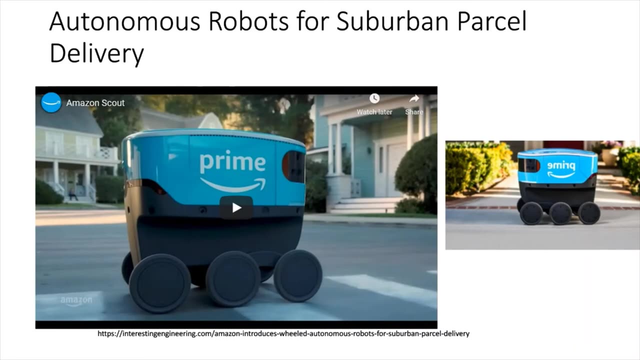 have any z information. there's no depth of the field, so, but sometimes again it's challenging because we have a lake of third dimension. so for the complex task it will not give you good results like a bin picking so now. so i will tell you that another like very motivational. so now using those. 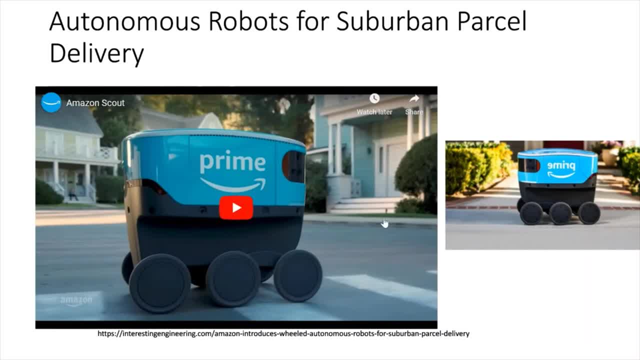 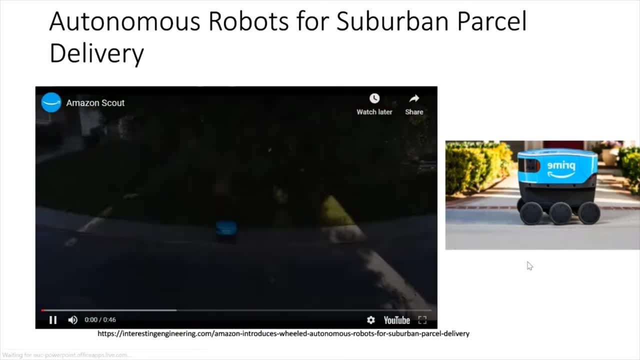 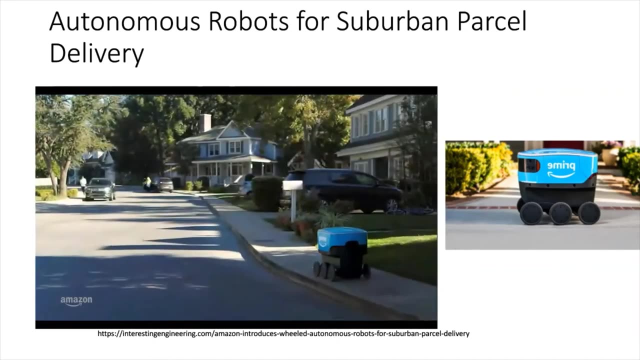 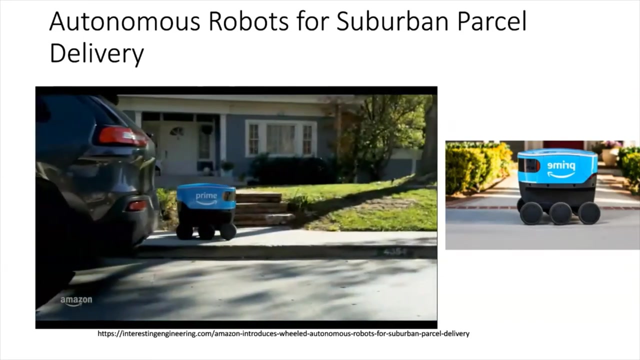 2d and 3d visions. so you guys would see, maybe this so amazon with- come up with this autonomous robot, so they have this pilot test in seattle and so now they have a packaging industry for this. this is a type of thing you can use if you're a bagger or whatever you're not. 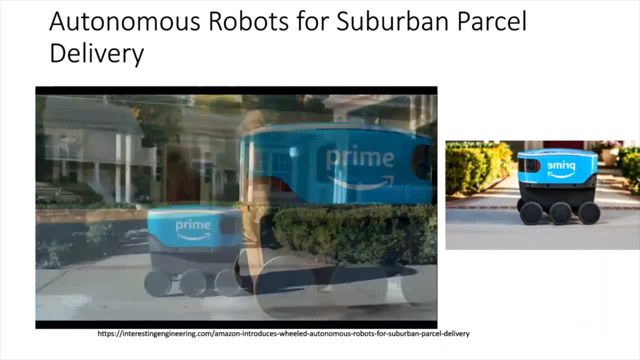 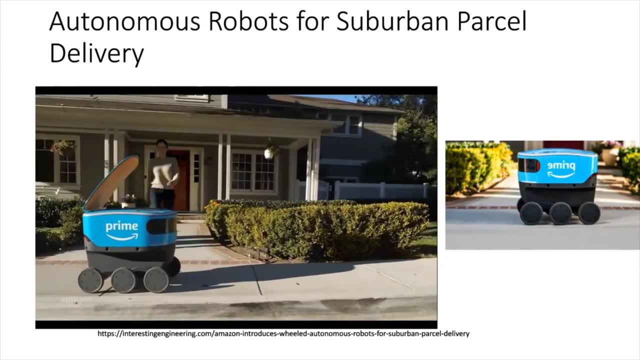 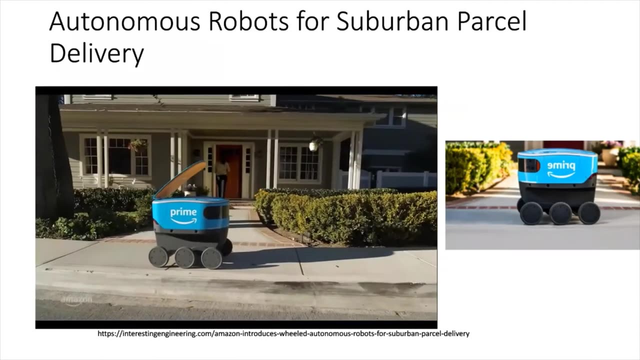 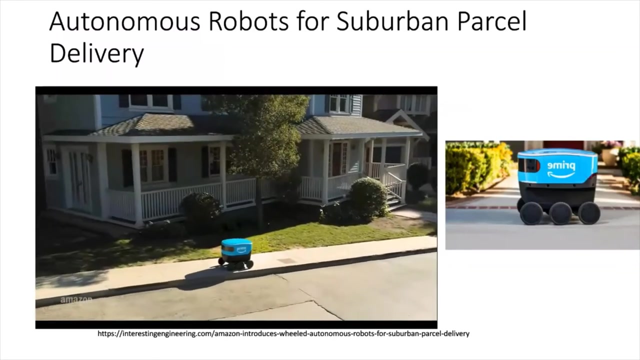 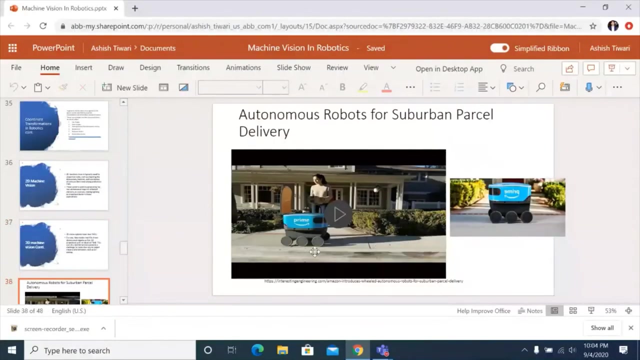 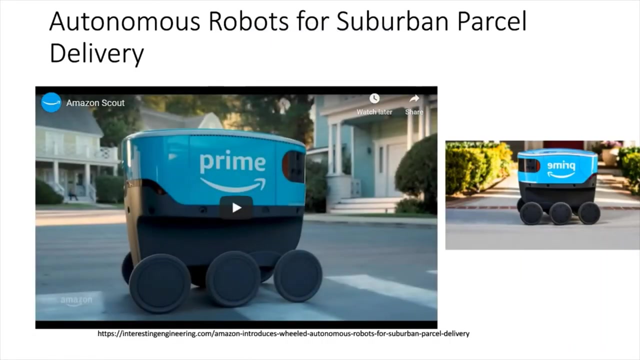 going to sell anything for let's see. so, oh, so, so, so, so, all right. so you guys would have seen, right. so the amazon is, the amazon is using those 3d vision technology for delivering their packages and i don't know like. again, i'm saying: 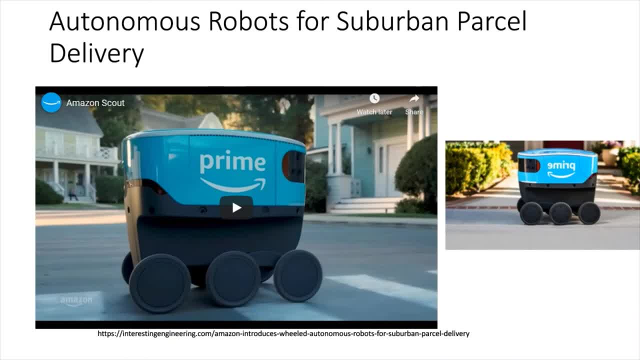 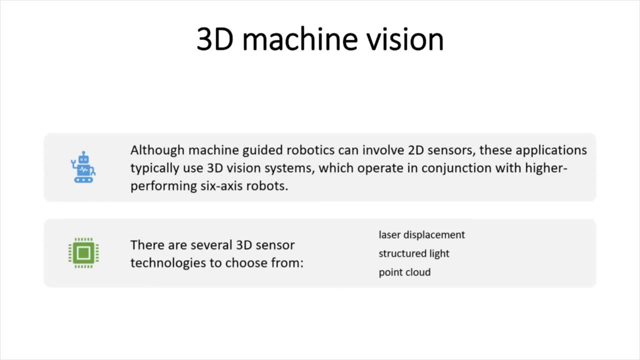 this is not very far. maybe 10 year, 20 years packages could be delivered by drones or this. so it's, they are in experimentation mode right now. now we go to the 3d machine vision. so this is uh, so very much, uh is a current trend. so a lot of application using the 3d machine vision. 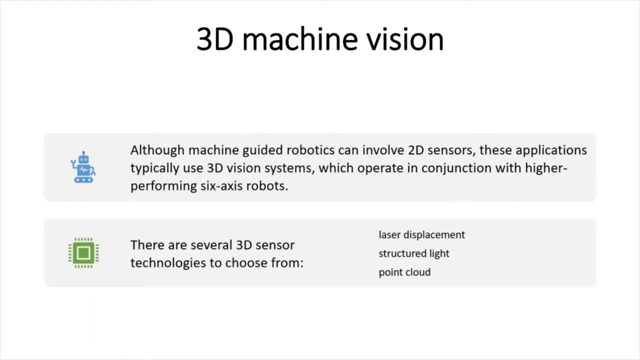 so, although machine guided vision- uh like it- can involve 2d sensors, but, as i said, they have their own limitations, we use mostly 3d vision system and we have because using those six axis robots. so the previous video i showed you, there also we have those six axis robot you can. 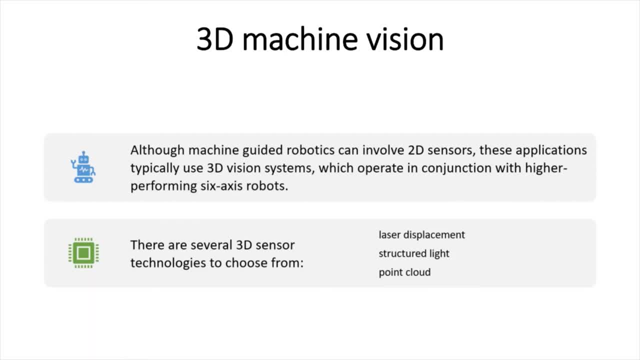 google about it, they can have a six degree of freedom to moving. so now, like our hand, also have like freedom, right? so similar, like our hand have, i guess, three or four degree of freedom. so now there are several 3d sensor technologies to choose from. so we have a laser displacement, we 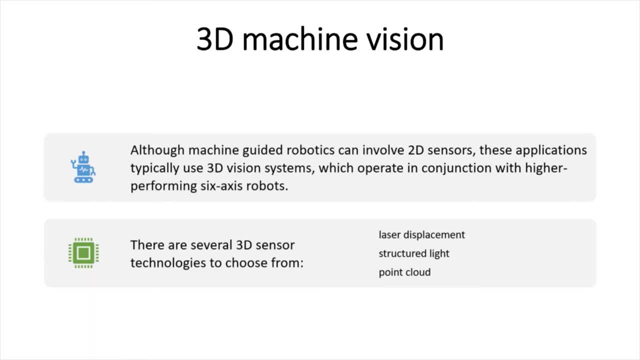 have a structural light, we have a point cloud and this point clouds and all i'll tell you. maybe, if some of you students and you would like to learn, there are some open source tools and libraries that is very useful for doing experiments and learning in three dimension. so now again same. 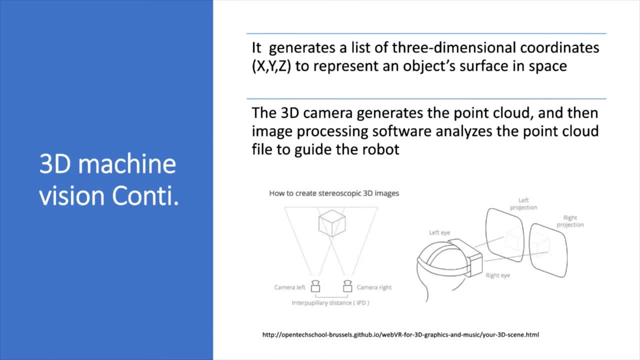 thing. so we have seen that stereo, uh uh stereo examples, right stereo visions. so similarly, these cameras having the similar motivation to the eyes, generally those 3d uh cameras or stereo cameras, have this uh two sensors, generally their left side sensor, right side sensors, and they they put the light on. 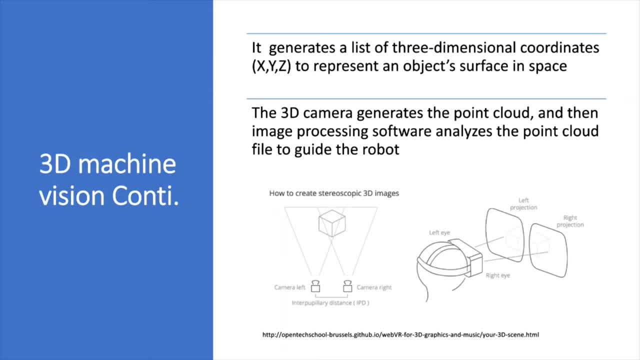 it and then reverse, they take two images and then they combine that one image and basically so, and they represent that one point into that three-dimensional coordinates that we call it xyz, and then 3d camera generates the point cloud, right? so one of that point cloud is basically again is: 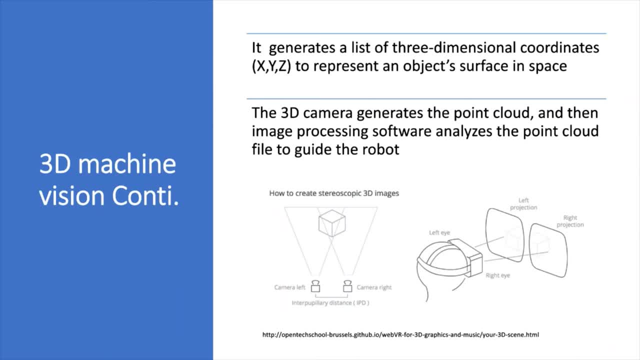 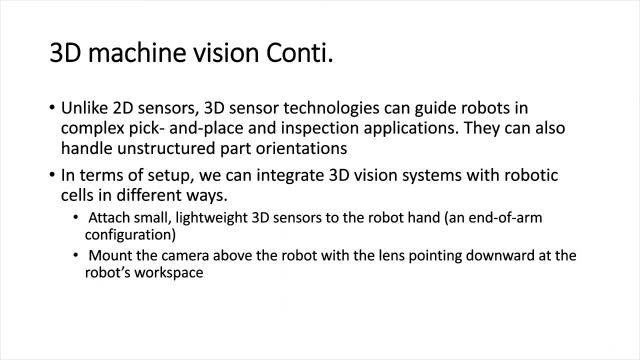 a collection of points in 3d xyz, then image processing software, analyze, and we can guide it. so there are different applications. so even, uh, those autonomous cars, they use this 3d, 3d vision technology. so now, as i said again, 2d vision has its own limitations. uh, with 3d sensor technologies, 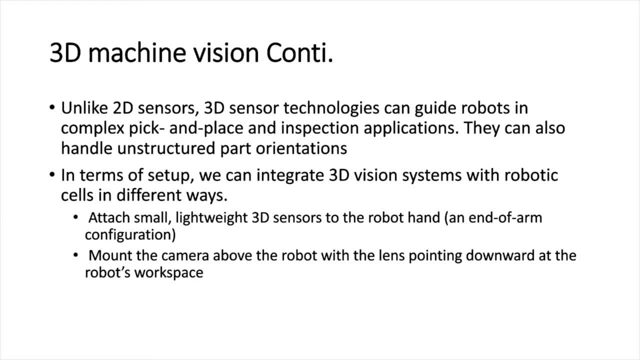 we can do more complex tasks and we can do more complex tasks and we can do more complex tasks there. we need more uh depth information like pick and place that bin picking. the previous video i showed you with abb, they were using 3d machine vision technology. so again, but again with the 3d. 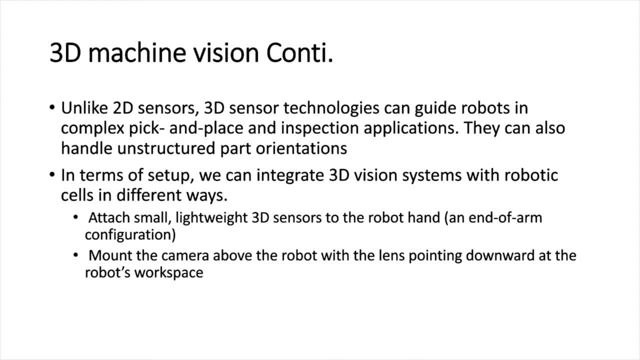 vision system. we can have a different type of setup. so so now, like we have i fixed in our then we have two eyes and one head, like now. robot has the option: either these robot eye or this robot vision sensors can be attached to the robot hand or it can also be a little bit further. so either we can attach into the end of the arm of the robot. 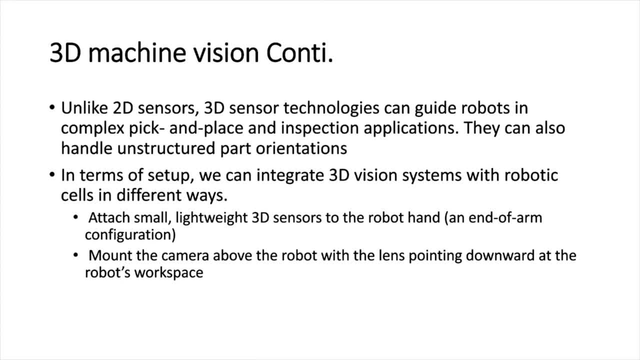 or we can mount the camera, maybe above the robot, but then it have its own limitations by the height. some, uh, the cameras have their range right if you have to be this much meter or within the range, but they are, they mounted above the camera, above the robot, and then lane pointing to uh, downward of. 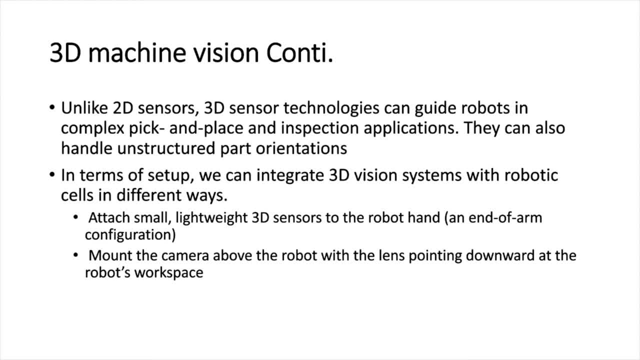 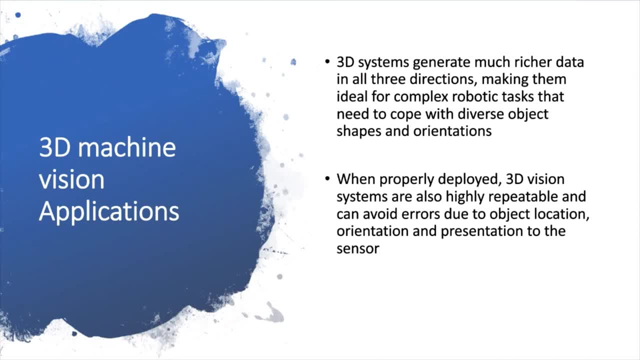 the robot workplace. so there's two way. uh, we can have it. so now, different applications we can use, because those 3d systems give you more, uh, you know rich data. we have different applications. right, you know, like we can have shape there, we can have orientations, we have a bin. 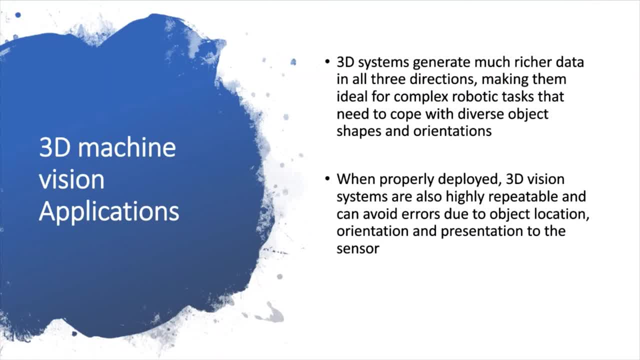 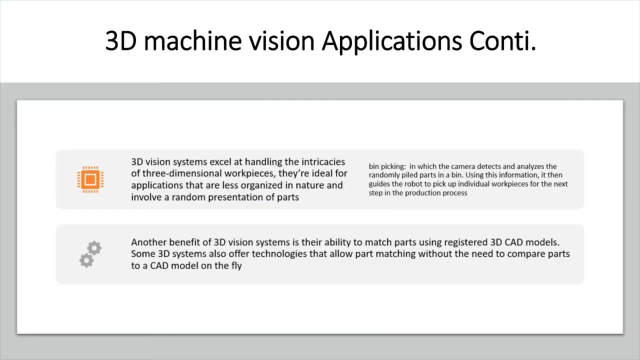 picking and then if we can properly use these 3d vision technologies, then we can avoid a lot of errors because we have a accurate their location, their accurate orientation and accurate uh presentation in our world coordinates. now they're basically the application- the video i showed you this, basically that bin picking a lot of applications. 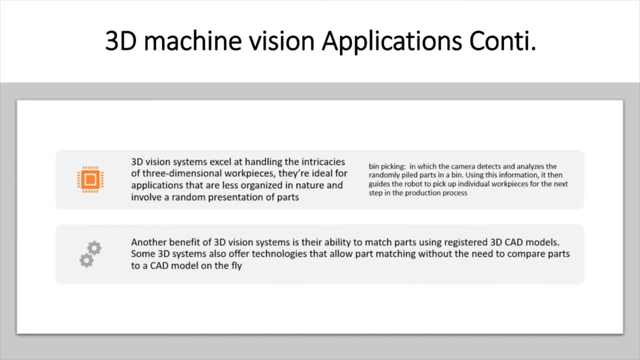 that in industrial robotic segments, lot of like uh bin picking. we have those uh. warehouse automation. there is a conveyor belt and we have to pick of a object from the conveyor and we have to place in some objects. then we have uh another benefits of 3d vision. uh, we can also have those object. 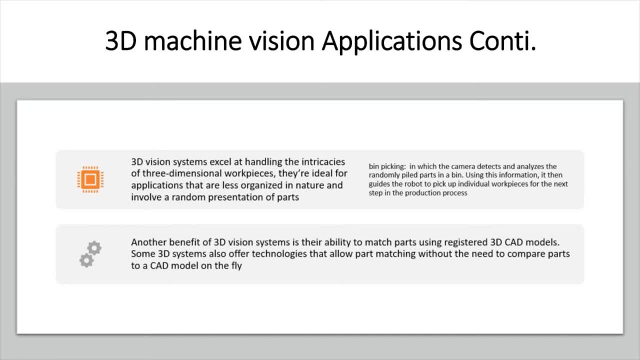 detection. we can match the part. we have some existing registered, maybe cad model. if you guys are mechanical or something where, like using those matlab or you can create a mac, uh, mesh or cad models, so you do this- uh, existing registered 3d cad models. we can also get unknown objects. we can compare with existing 3d cad. 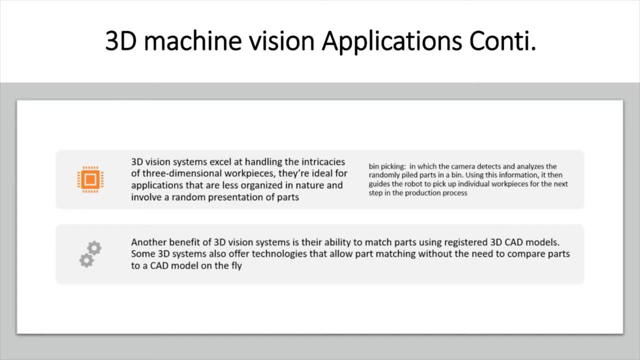 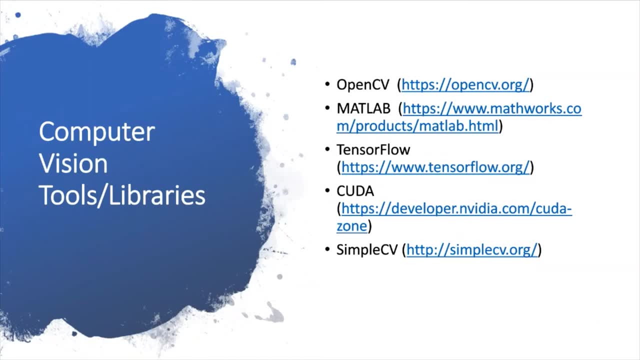 models. so that's uh, this also empower us for this 3d cad model comparison. now for the like, as i told, uh, those who are the beginners or would like to have a career in computer vision or these tools to do your, uh, your college projects or your thesis. you can like, you are welcome or you can, you know. 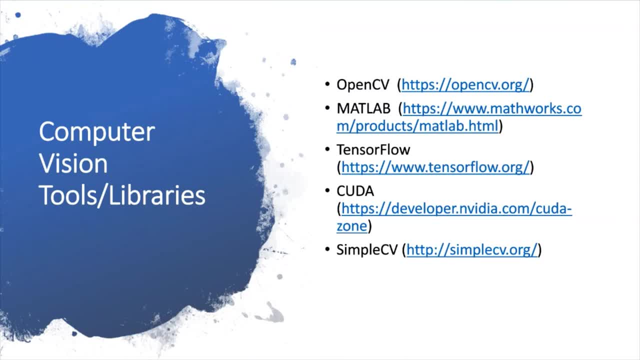 say different, very important tool about those computer visions, so this one like maybe it will be. uh, it will be not complete without talking about these tools like opencv, so this like open computer vision. so i have also given here link. so this opencvorg, so a lot of these computer researchers. 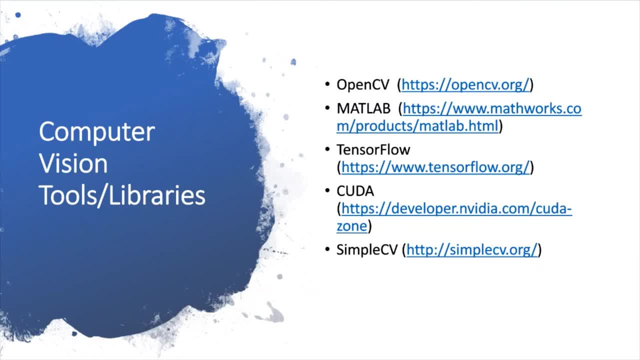 we, we use this heavily. so, like i'll not talk about more about my project, some of the projects we do in you know, just proof of concept or confidential ip label, but i can just say about technologies. so, yeah, we also use this. opencv things, a lot of lot of opencv uses, and it's also in different language you can use in. 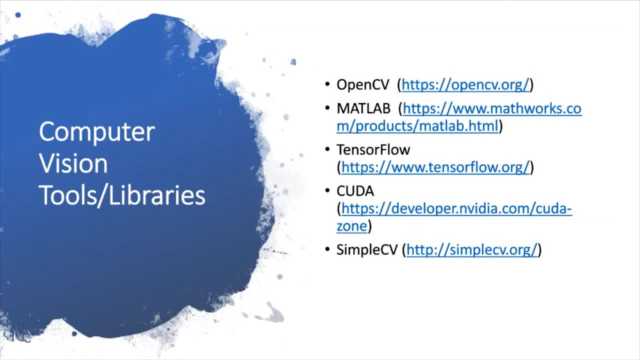 c plus plus you can use in python. so i guess they have a different version, so another one is like a matlab. so if you do your masters to your phd or whatever, so it's very much- you can have a lot, of, lot of mathematical, your matrix computation, your lot of things. you can be, we can be like: 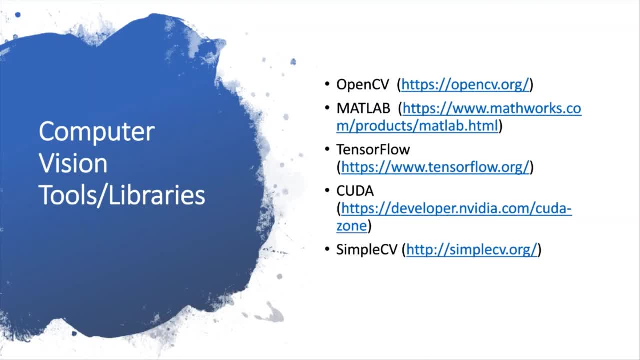 achieved by using these in matlab and other, these computer vision tools and libraries. i would maybe some of you already know these popular details like a tensorflow. they are basically, you know, like a google big pioneer in technologies. there was internally. they developed it, i guess, 2015. 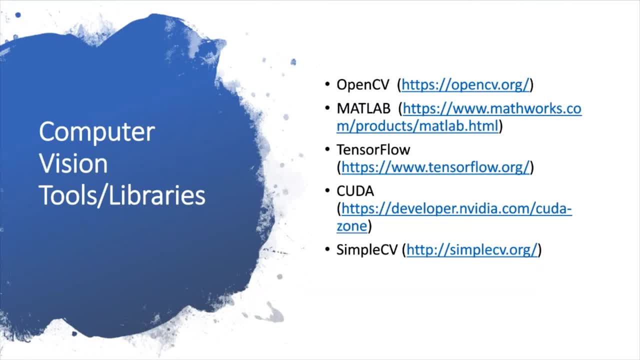 they, they did it open source. they make it, uh, they will. they make it available for all over the world. so and then tensorflow is growing from them. it's mostly in a c plus plus uh. it can also be like sometimes, you know, resource hungry, but they also have its advantages and disadvantages. but it's a. 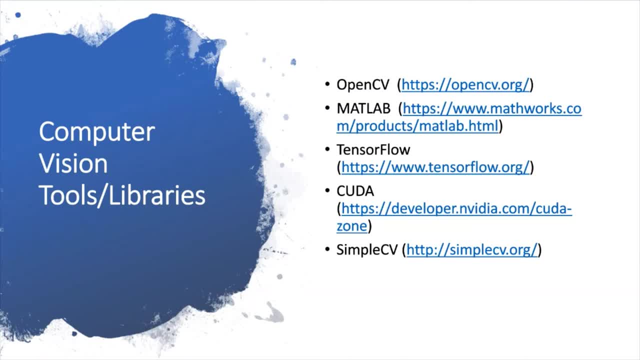 lot of, lot of examples, lot of libraries and a lot of, you know, pre-trained model. so if you would like to do any experiment, or even also you can include, i guess, your python applications- uh, you can make your basic examples of computer vision, object detection or recognitions. or you have your toy robot or you want to play, you can do a lot of things. 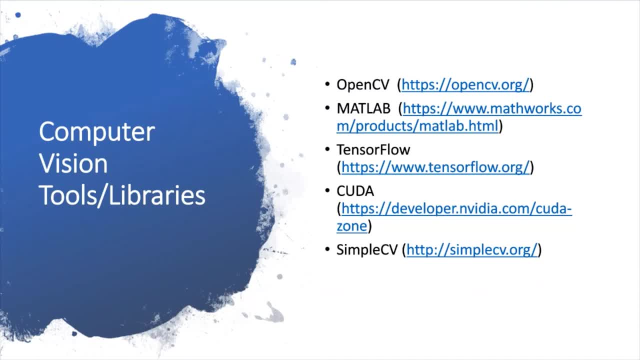 then other tools called cuda. so cuda is actually basically uh is open source softwares developed for you know those uh, you have those parallel computations, so it will make very your computation very fast. it will basically utilize your graphical memory. right? how much your graphical memory, if some of you guys are- definitely you guys are playing uh. 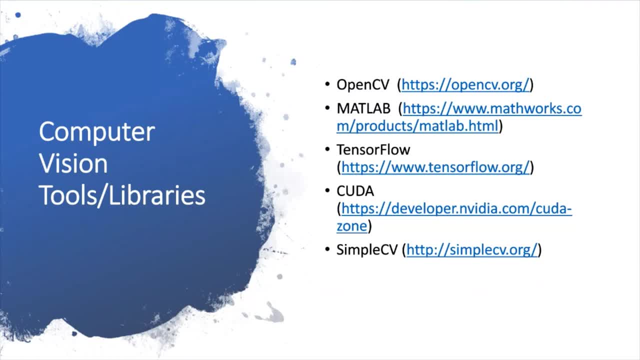 maybe video games, and all right so. so if you play video games, you would have those, you know, you would know about those graphical memory and all. so cuda is basically utilize those and that, uh, it enables to do those color computations so developed by the nvidia there. 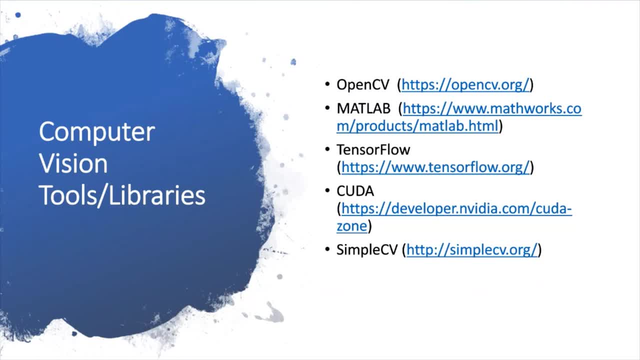 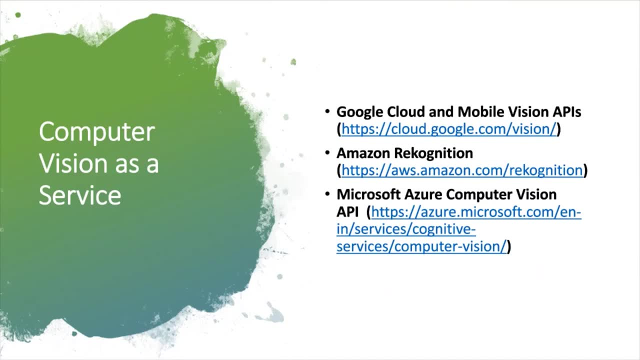 is another called simple cv. it's basically more like open cv, but it's very simple and lightweight. again, you can utilize and do it a lot of. and now then i guess we are almost close to the end of the, so i would also talk now. this industry is growing, so now this is very popular in computer vision. 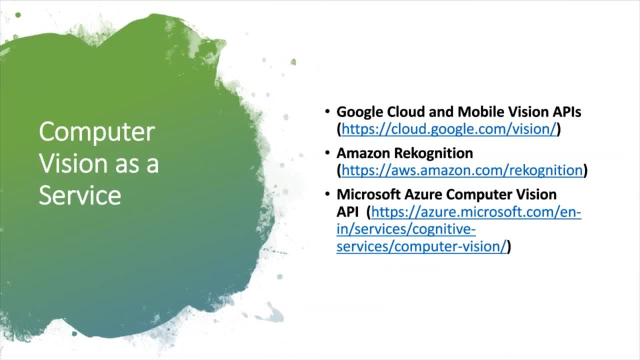 also making as a service. so now, these days, now google cloud and mobile vision, apis again because it's required. you know a lot of resource, a lot of applications, so now google also giving them as a, you know, as a service. now, similarly is a amazon recognition, they say. 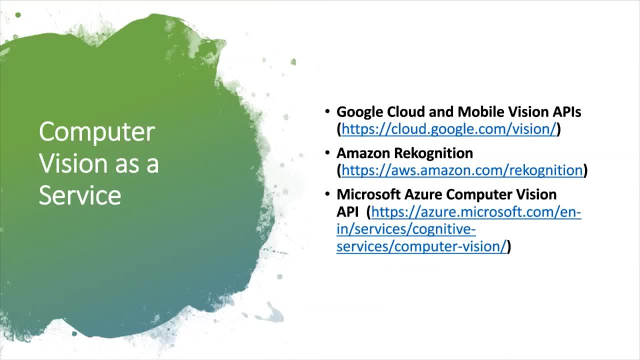 recognition. so they're also giving. using, uh, using these services, you can have your, your lot of images, you can have your identification recognition, your labeling. then other another is from the microsoft azure, the computer vision api is the same thing. so these all companies, uh, they are also helping to communities, uh, maybe using their cloud technologies, amazon. 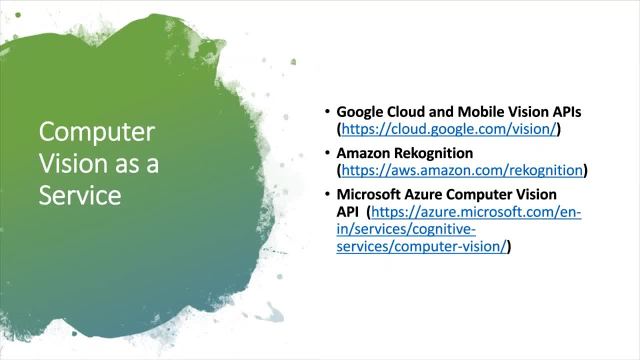 have aws, the google clouds and amazon microsoft zoos. so they are. so, if you guys, these are a very good resource, if you would like to do experiment, you would like to learn and i would like to say you, you find your passion where you would like to grow. what, what you would like to learn? 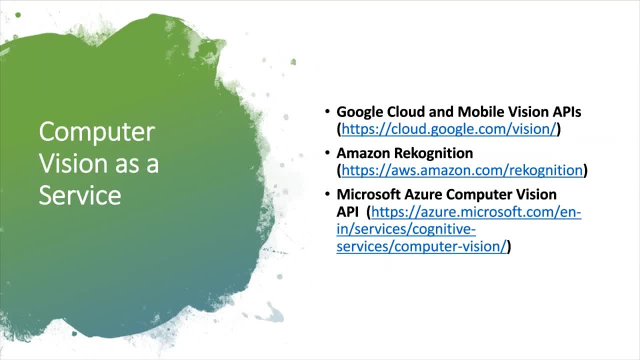 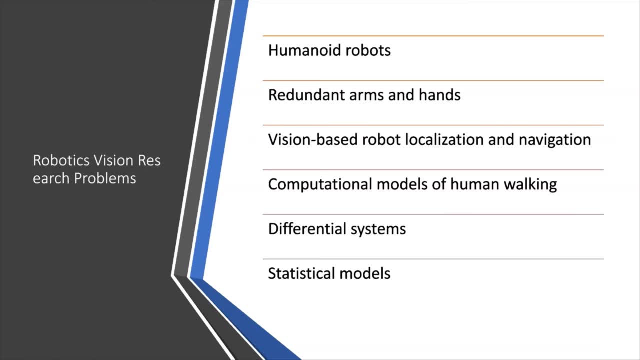 like and then then you decide on this now basically. now last topic i guess here. so if basically where the robotics vision, research problems, these open problems, where this going on, robotics vision, basically now humanoid robot like robot should do, basically like a humans until it see and think, then we run the entire man hands, then we have vision based robot localized. 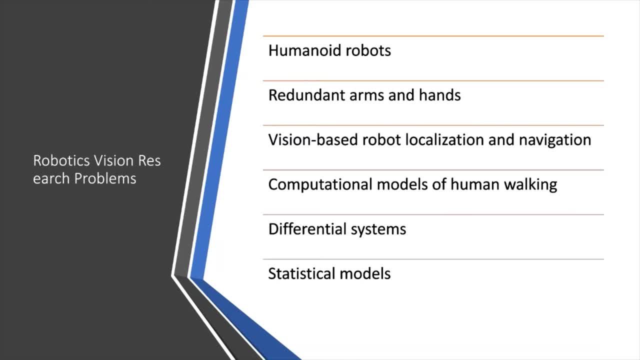 and navigation, uh, computational models of human walking, so like how human walks. so we have to find out and learn it like, because we are a lot of adaptive as well, we can run, and then there is a differential system and there are a lot. so these are different applications, right, and again i would 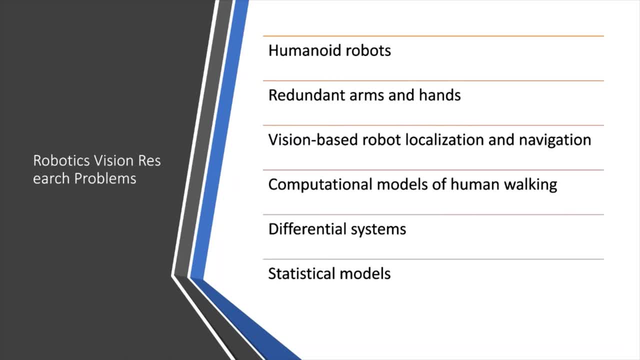 say we should have, you know, passion about things you would like to, what you would like to learn, what you would like to know, and if you, you, you try to solve something, um, some problems, you know, say we say like, like a invention, like necessity, is the mother of. 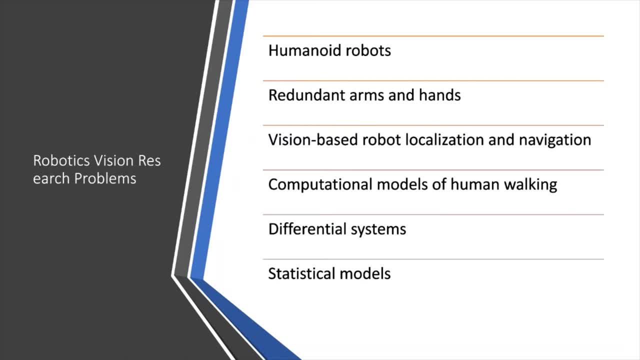 invention. so there are a lot of problems. they are unsolved. so you pick up one problem if you try to solve and that is getting used by many people, then, like you can make a better world, something like that. so the one famous quote i would say i would end my presentation with this: 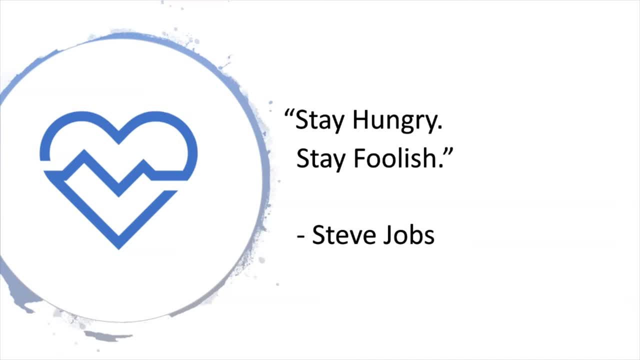 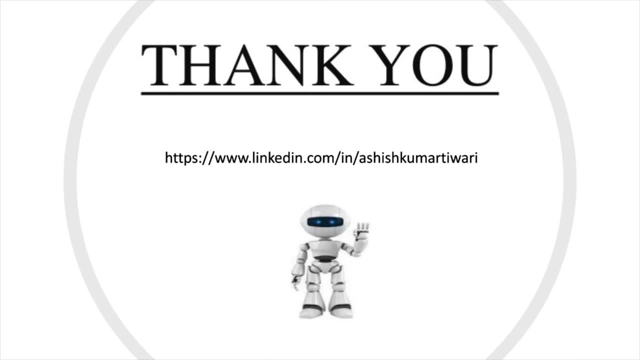 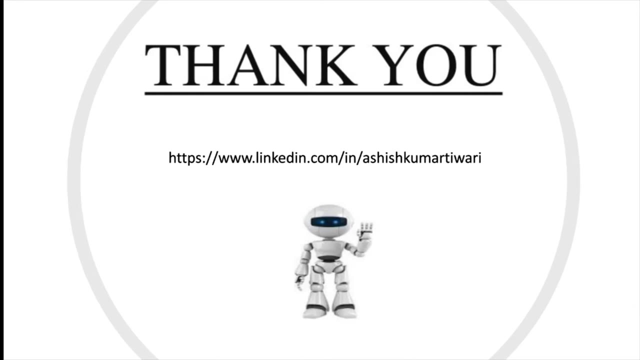 like steve jobs quote: stay hungry, stay foolish. all right, thank you, and there is my linkedin link here. so if you would like to use, if you would like to contact me or have more information, you can contact me in linkedin or some social media. all right, thank you. thank you guys. 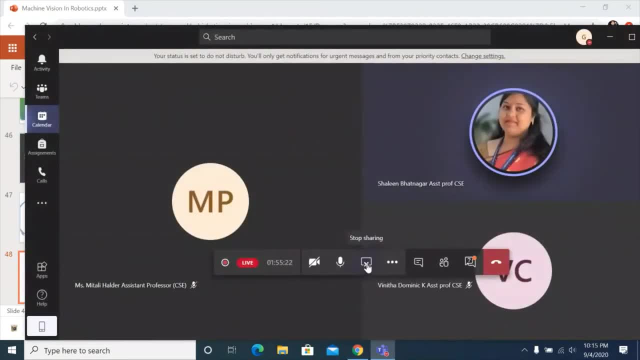 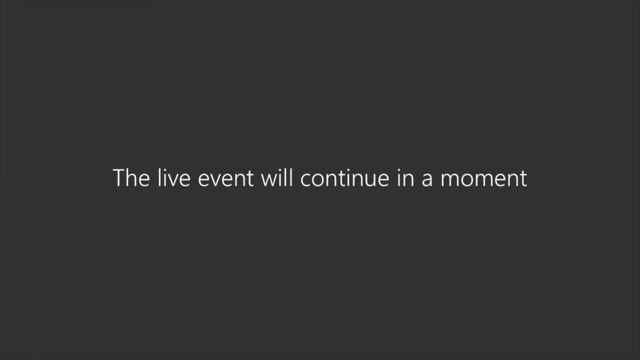 thank you so much, sir. thank you for sharing your deep knowledge with us. the session was really insightful and enlightening. we will go ahead and take some questions now. so just a reminder to be sure to all the participants that if you have any questions, please do not hesitate to ask them in the Q and A. 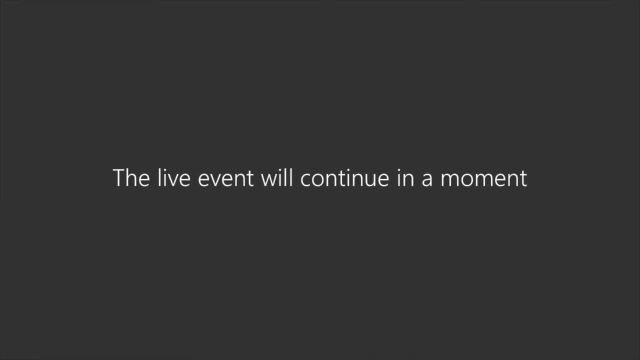 and we are going to answer those questions. sir is going to answer those questions. so it looks we have few questions here. so, sir, i'm reading the questions one by one and you can answer. so mohit is asking: what is the difference between machine vision, computer vision? 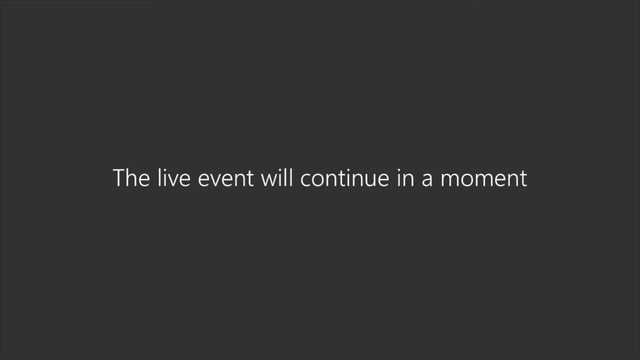 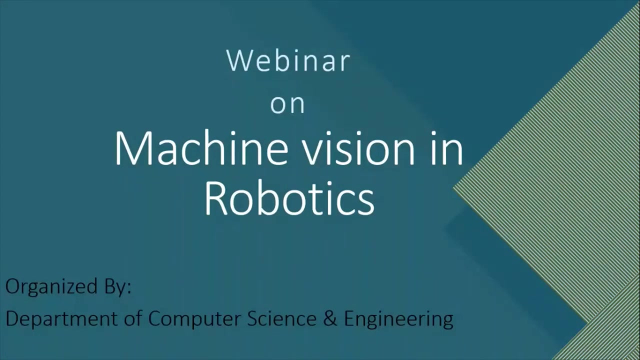 and robotics vision is all are the same. it would be like a good question. i would say it's more like they all are same. so we just call it robotics vision means more focused on the robot. so we are giving into the robot perspective, because robot has his own- you know- limitations, or a robot has his own. 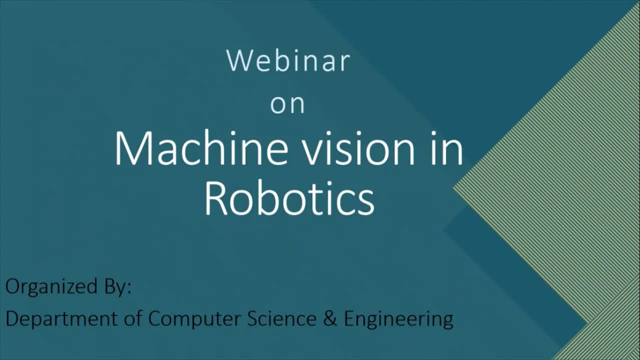 coordinate system. but when we, and then the, pretty much it's become like a sensor for the robot. but when we say the computer vision, computer vision also couldn't be used without the robot. so they say, like machine vision in robotics, so in. but in other terms, again i would say one term. 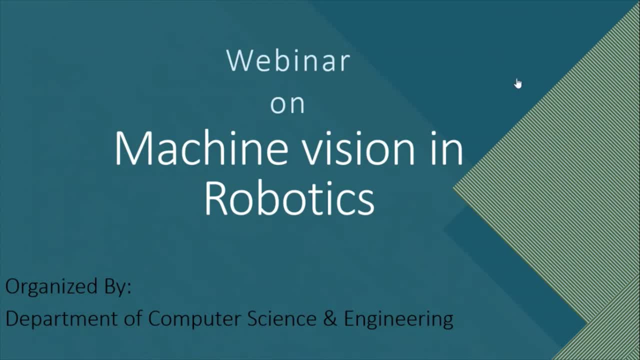 machine vision or computer vision is deep learning, so even in automated car we use it, so they are almost also same. yeah, okay, thank you, sir. uh, arnold is asking. i had underwent training on robotics- industrial robotics- back in 2018. machine vision wasn't much implemented, it was in the 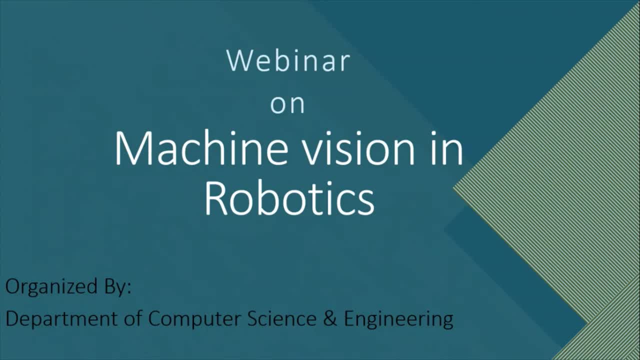 research phase many. my question for you is an industrial robot. is the machine vision used only as the end effector, camera fix at the end effector of the robot- or is it implemented to the entire workspace of the robot? if the machine vision is implemented to the workspace of the 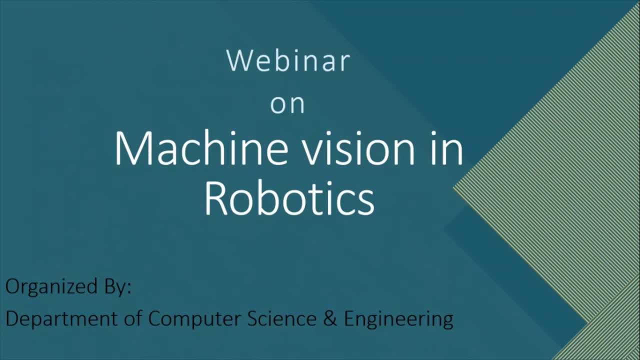 robot, then is it only to detect human entering the work, workspace when industrial robots? one minute when industrial robots are in action, or in any other main purpose of the same. okay, so so let me, let me try to give, uh, maybe a little bit a detail about it. so well, i know kuka. 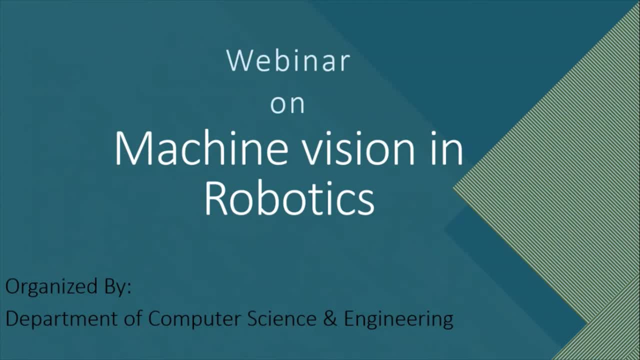 robotics. so basically they are one of our competitor. so if you go in industrial robotics segment, so the there are two or three only leading companies, so like abb robotics and our companies, and then this kuka robotics. so yes, i would say: uh, still this computer vision, this is still a child. 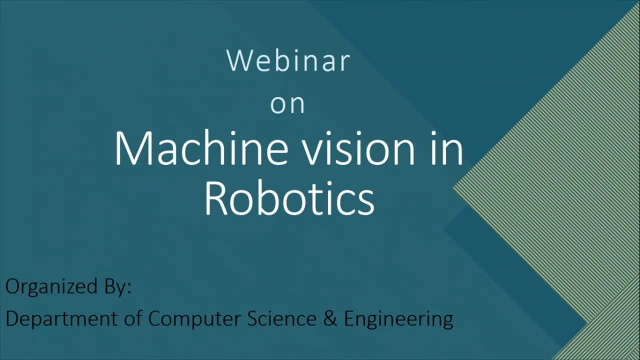 still it is growing. it is still not matured enough. like automated car is not yet the norm. but similarly we are having machine vision applications, but they still not that much mature. i would call it so. but right now again there is a focus: applications. so we have some application, maybe kuka robotics or some of. 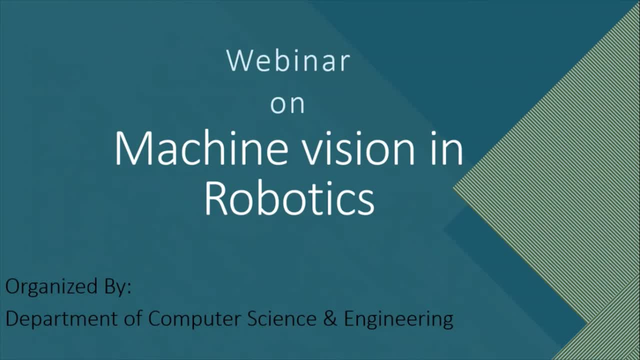 the projects we are also working on, or they are also working on, but like i cannot share so much detail about it, but in general there are there. there are applications that are being implemented in industrial robotics. now robot has to do some warehouse automation, so they would be used. 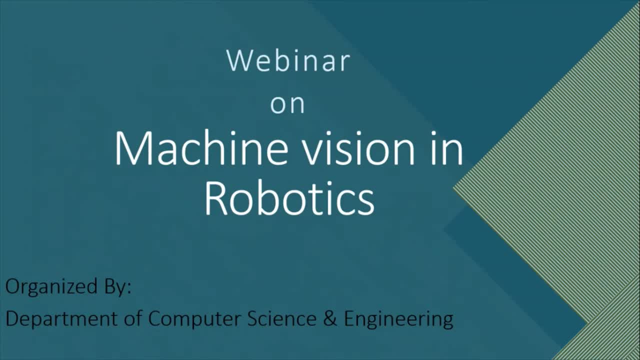 basically in this section and i guess they are now popular, more popular in this bin, picking applications, you know, like we have to in warehouse and replacing those humans for doing those packing and barcode readers and pick and place or deep elitizations. so, but some company, i guess, started. 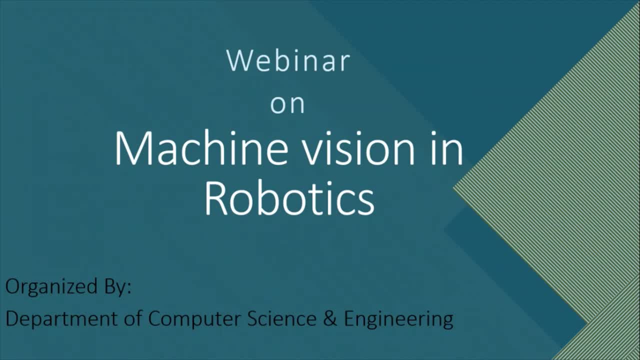 using it, but still it's in a, like you know, growing phrase. okay, i? i hope you would have answered a little bit. shubhadeep is asking: if the road condition is bad like indian road, which sensor sends those? yeah, so, yeah. so i also grew up in india, right, so i've been there, like i have seen. 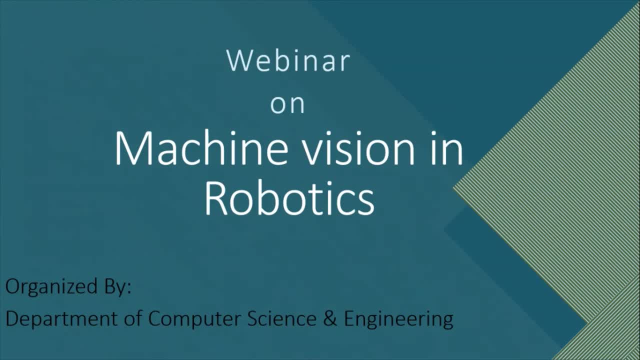 even bangalore traffics. i used to work there and, yeah, these are, there are some of the challenges. so again, um, so that's what i said. it's not a norm yet, but it's a road is bad condition. similarly, what about, like, uh, we the the camera is seeing the? 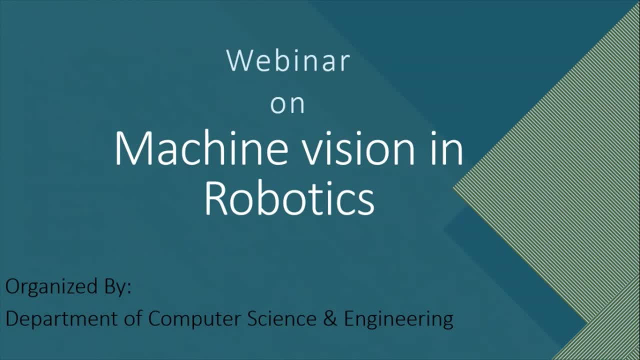 length of the you know, uh, the road. right we have like a white, uh you know, strip or something. but what about when the road is bad or there is a heavy rain or there is a snow? in united states there are a lot of snow in some areas, so road is completely covered. so now this only seeing by the 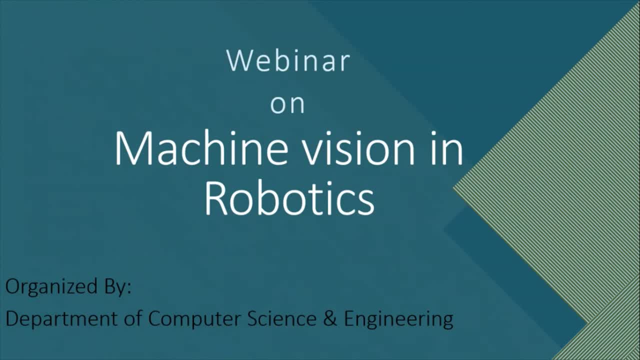 camera or just having those color images or pine cloud would not be enough. so they actually there are researchers working on different technologies, like using radar, radar or lidar technology, so they don't have to depend just by seeing, by having their mapped. so if they know, if the you know the, 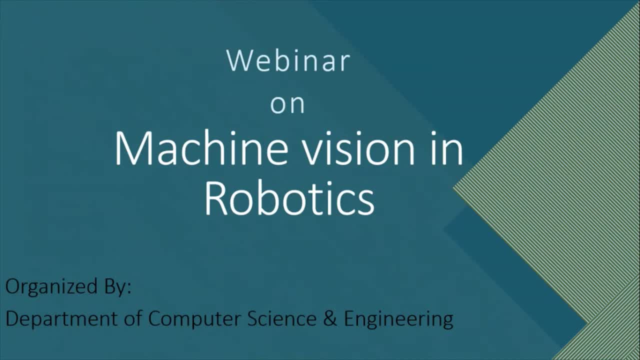 total width of the robot. the road is this much: you are in the west side of the road, but again, again, i'm saying it's difficult, it difficult in those uh, difficult terrain of the road. so but they are finding some solutions. so mixing, but again the lidar and using 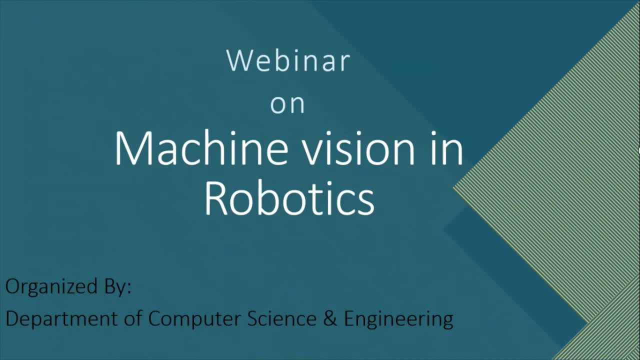 radars has become costly. so they are mixing technologies and still in a growing phase and i'm sure these researchers are working. so one uh presentation. like i shared one guy from, i guess from mit, one video i showed you guys would like to maybe visit and see their videos. they are like into that good. 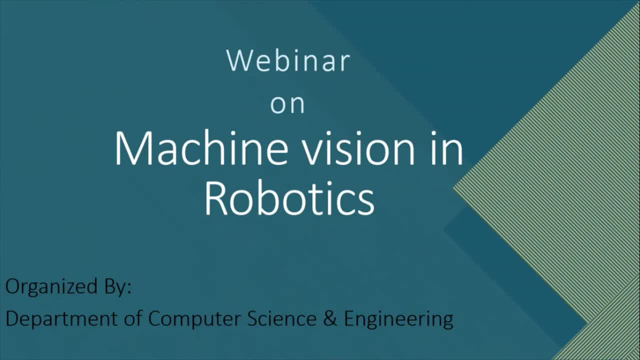 research and different companies. i hope deserve help. yeah, okay. next question we have again from arnold. according to you, what that means, is that the one main thing which is making india lag behind and research in ai or machine vision when compared to the foreign countries like us? is it because the unavailability of the resources or any other reason? 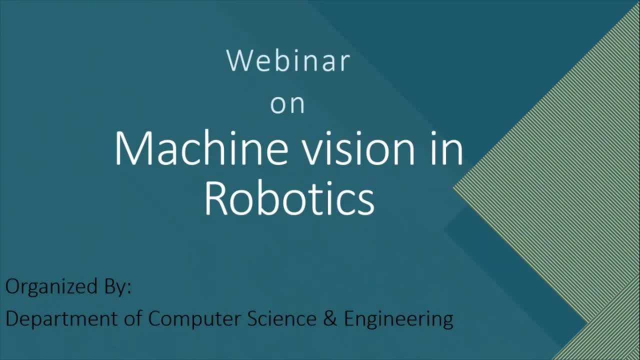 apart from this, only technology or even things like this, which does not support our organization. the high level of research of solutions makes it very hard to educate and guide an individual and help them to be successful when they are getting the information right and to help them to have their own. 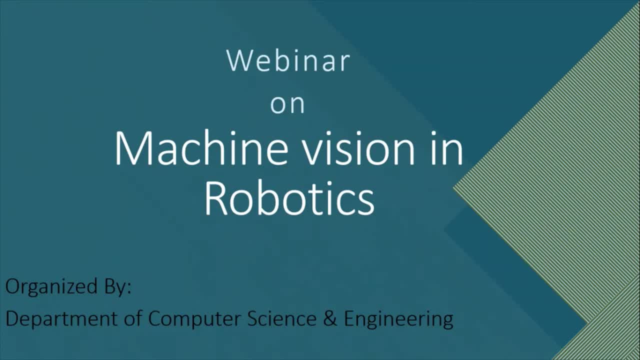 opportunities, which is not the case with the technology or the technologies being used in air fuel system, and we know that. you know, when you go to an aeronautical facility you are gonna be able to get your own of still, and we are adaptive, like we change things very fast. so there is a positive and 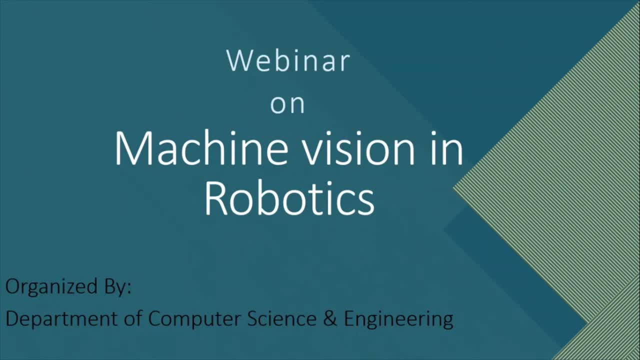 the thing's gonna change, but i guess it is slow. if you directly compare us technologies with the india technologies, i i guess it won't be a fair comparison in like in, you know, in a different context. so yeah, the both are growing, india also growing, but maybe in a slow phase. okay, so another. 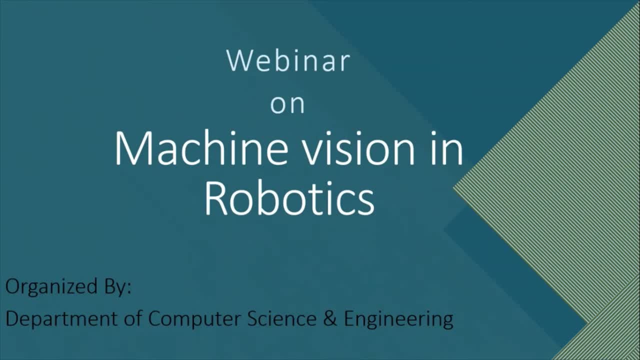 question we have: are sensor designed for all uh trains or, depending on the place each sensor is made? if so, how it is? how is it compatible? can you repeat like this one, what data number? uh, sure. so here is the question: are sensor designed for all uh i? i think i'm not pronouncing it properly. 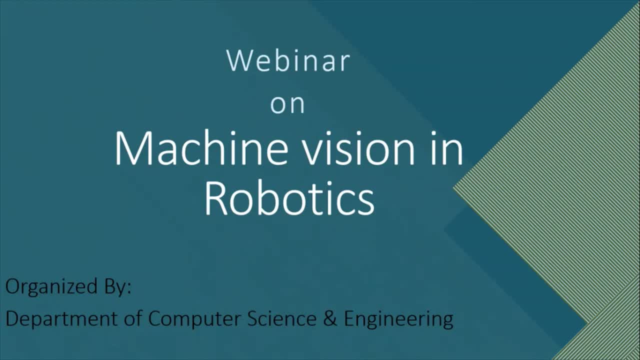 terrence or depending on the place each sensor is made. so, if so, how? it is compatible? um, so you can see all the question here. you can uh on your screen there is a question mark q and a q, okay, okay, yeah, if you, if you will click, you can read all the questions. so for uh, my end, the 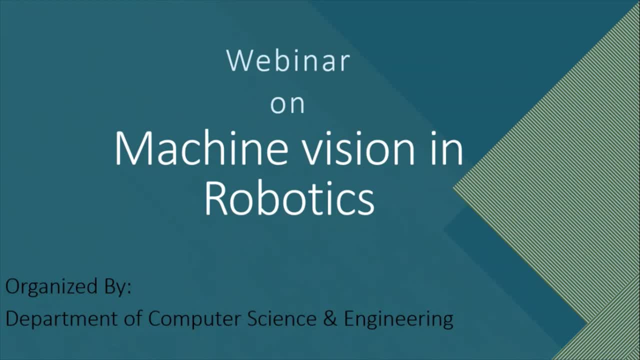 question: uh, someone is asked my end, i would say as a researchers, so there is a no one thing that is perfect in all the condition. so it's, you know, it's always using, you know different, so, like no one is perfect, so similarly, uh, sorry, so similarly, one sensor is not perfect, as i told you. like, uh, as. 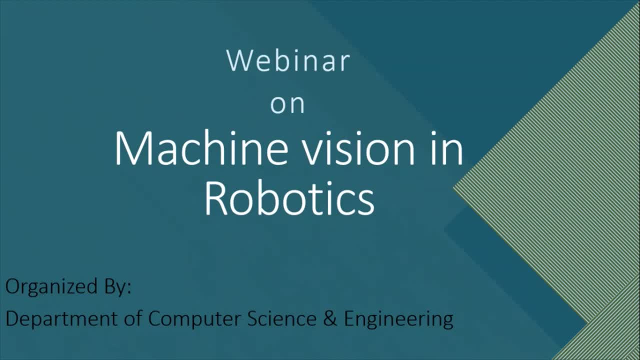 you said before, they are not using different sensors, but they are using different sensors, so this one. they are not using this one sensor. so if you are in different terrain, definitely they used to. they have to use the different types of sensors. some sensors are good in some terrain, some 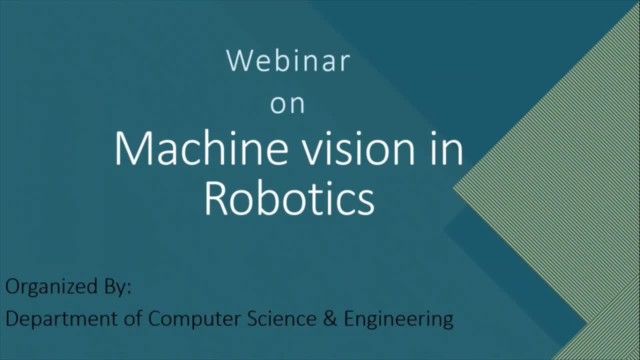 another sensor are good in different terran's. so, like there are a lot of slippery roads or there are, there is no visibility, or so they can use by different technologies and their resolutions might be different or their range might be different, but there is no universal thing. but they are trying to achieve it, but i believe 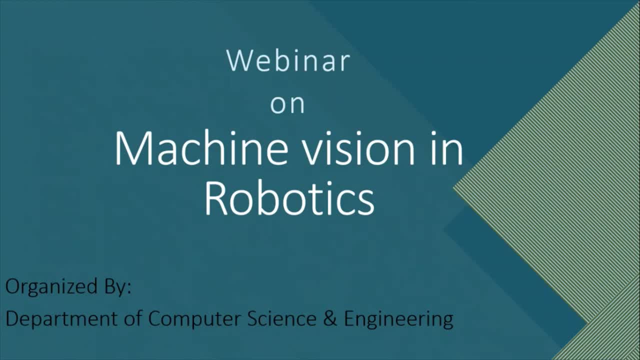 they might be utilizing a different sensors and come combination of different technologies. okay, another question we have. this is very interesting field to work. can you share some resources from where i can start as a beginner? what are the prerequisites to understand and grow in this area? so that's a very good question. i would say, uh, those who 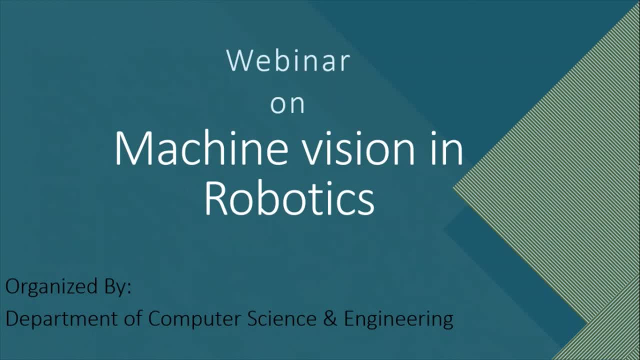 are the beginners and definitely would like to learn, and i will. i would tell you about even my story. so i was a software engineer. i i was good at like maybe data structures, systems, but i was very beginner. but i would, i had a passion about it. i would like to learn this machine vision or 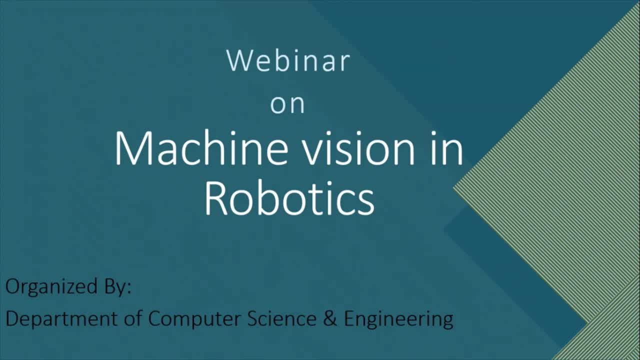 machine learning. so i i came for masters and and definitely having this background in, you know data structures, algorithm, it helps, so but you can start from anything from anywhere. and the sources: in my last slide i guess i have shared some of those tools. so those, uh, open computer vision, open cv. 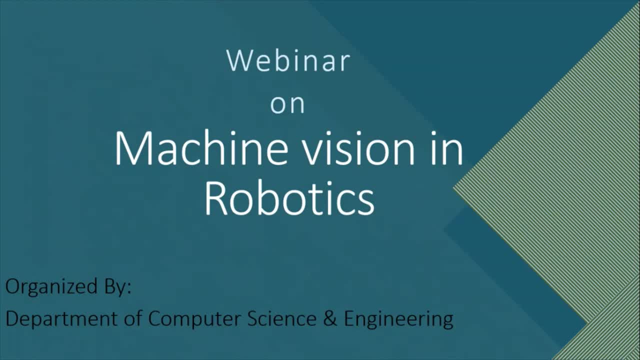 open cv and point cloud libraries and using even open cvs. they have a lot of examples. so if you know even limited knowledge of python, that would be enough, or if you are good at cc plus plus, that would be also enough, and then you can start learning about those. 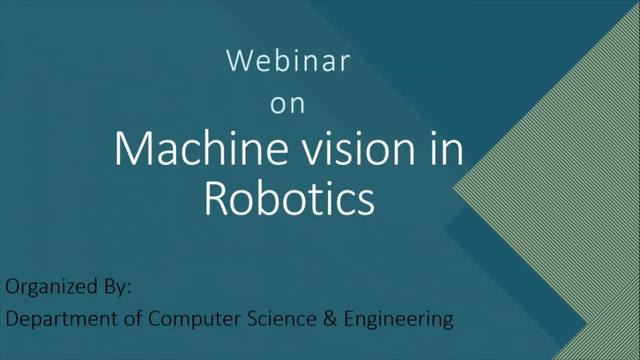 uh coordinate system and then basic your. they have their examples so you can start using those open source libraries. they are available in internet. using the git you can just download and you can just run, and there are also some of the online uh examples of tutorials. so i think it's not that. 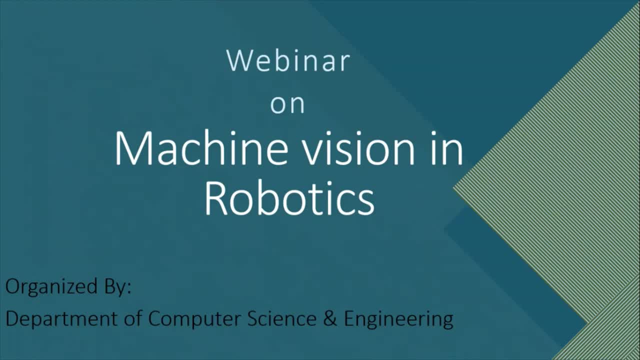 difficult if you are passionate about it, if you wanted to learn it, you can start it, okay. next question from paul and kumar cnb: help, is it speed when the signal went off? i think about automatic car. he's asking okay. so, if i understood the question correctly, uh, he would like to ask how it will raise the. 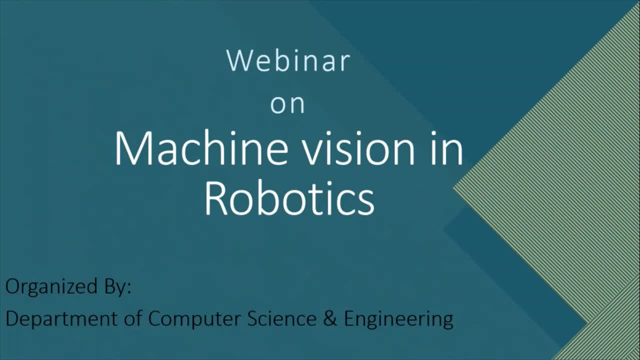 speed when signal is off, or it has to go fast because signal is going to be red, something like that. yes, sir. so if i would say so, it's a funny incident, right, even in india it's happened, even me, respect, my friend. so where you can say it in a green signal and watch where it goes, right. 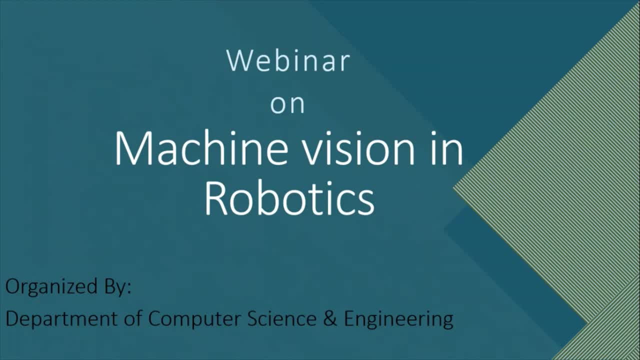 so that is a different case, like when laughed, but it has been a great at a green signal. so like people are the joke around, like when green signal we just go right. when it's a yellow and just, and when it's a red signal we just see nobody's watching. then we can go. 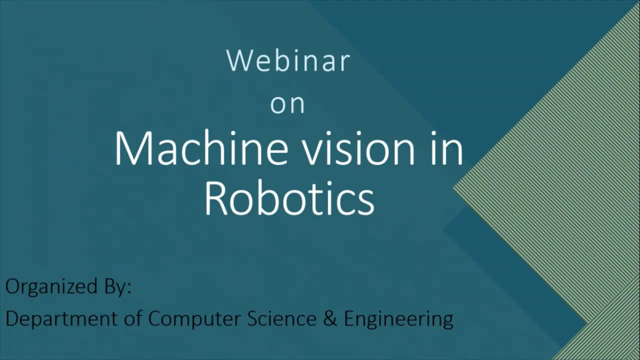 but it's not like that. so so i would say, uh, so in the like it has a prediction about right. so it's like yellow means like ready to stop experience. basically, when it see the yellow signals, uh, it is tend to stop. generally when you have a yellow, wherever you are, you try to just finish if you're half of the signal. 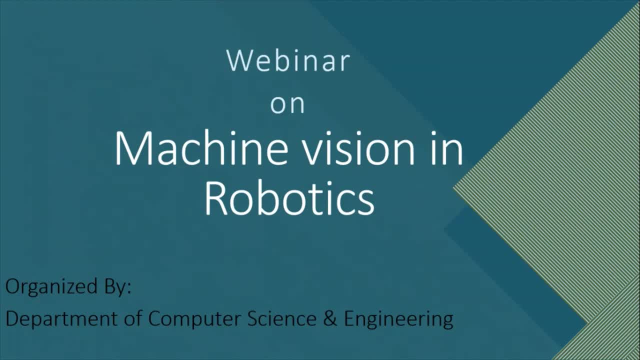 you just cross it but you are before the signal. the tesla car was stopped to the yellow and basically that should be, and when it is red definitely it has to stop. so i would say if all the cars is automated car in the road there is a less chances of even uh, collision or less. 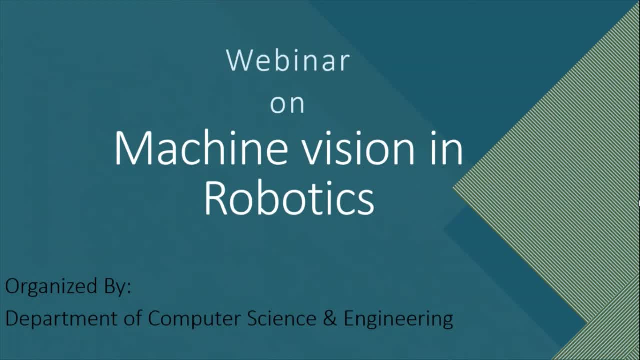 chances of accident. actually, it is good, we are the human, we do more mistakes, but the human and robot combined, it's again a trouble. okay, uh, sir, can we? it means, if the time is exceeding, uh, we can mail you all these questions and you can revert us back and we can share with the participant. 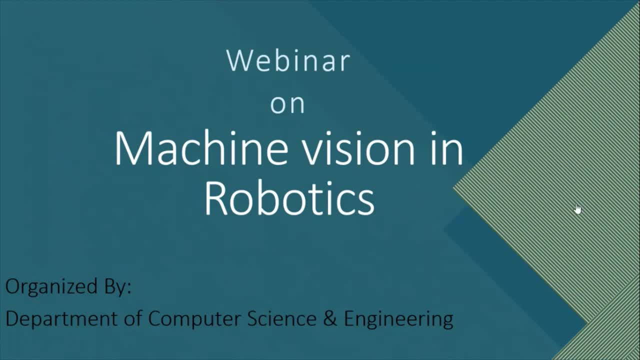 because so many questions we have. uh, if you say the time is exceeding, i can stop here and i will mail all other questions to you. yeah, that would also be great. yeah, you can email me and you would like to. you guys can reach, or yeah, if any questions or anything, okay, sir, can you share? share one more time. your, your, uh, like. 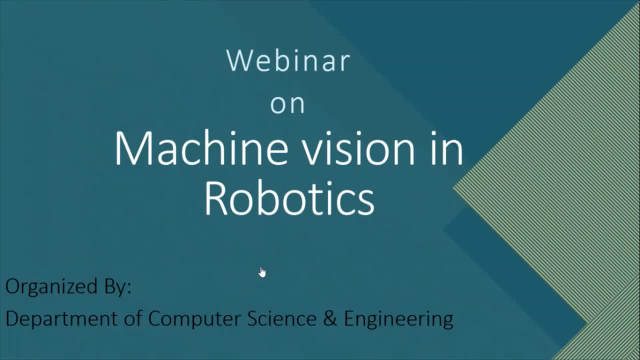 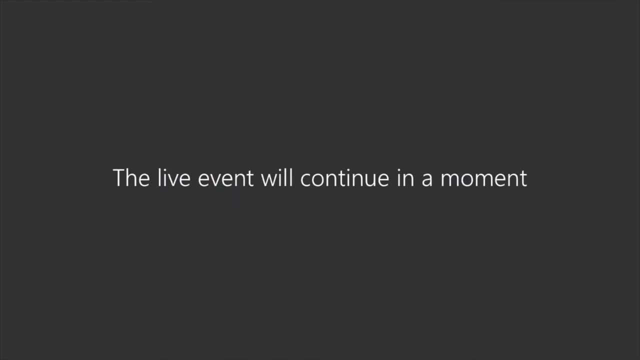 social link link link, profile link so that our participant can join from there. one more time. you can share it, sir. yeah, so they are participants. we are going to mail all the questions to sir and you can also join him on linkedin so you can ask or message him directly there and as soon as sir will revert back he will. 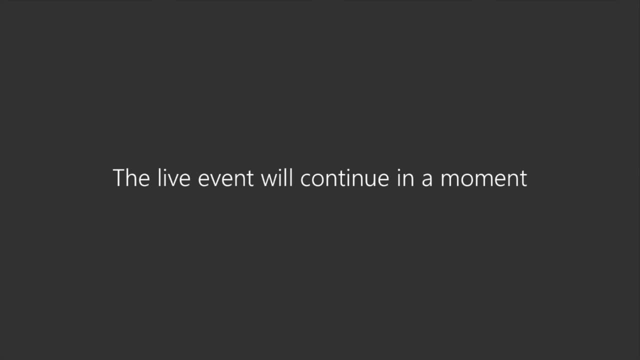 go through all your questions and revert back. we will be sending you answers for all the questions, because many questions i can see it was obviously very interesting session. there are many questions i can see here and uh, because we're already exceeding the time, so i have put into, i guess. 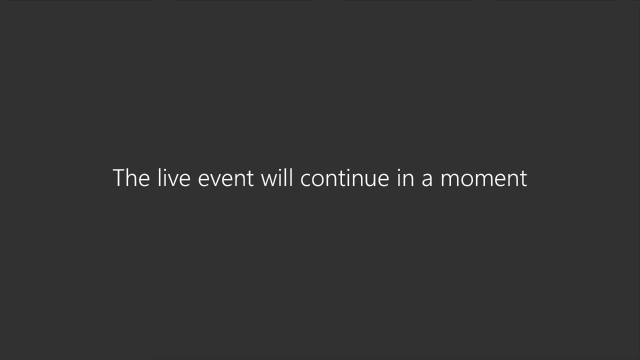 meeting chat. you guys can see that. um, uh, sir, i do. i think. like we can't see one minute, i will publish no problem here, i think i'll. i'm putting an announcement. everybody can see that, okay, yeah, okay, okay. so it's look like we are covered with everything. now i would like to request. 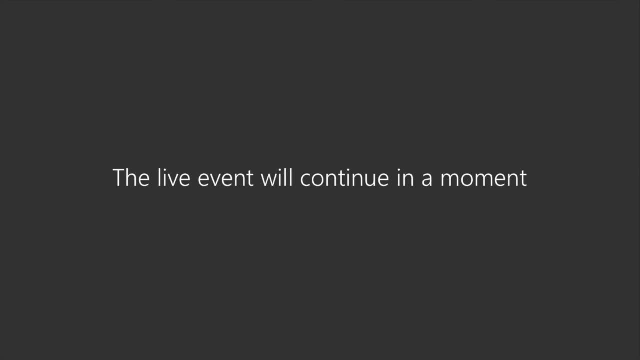 miss vinita dominic, assistant professor, uh, department of cse, to give away the vote of thanks. here we go. good morning to all. on behalf of ieee student branch presidency, university i, vinita dominic assistant professor, department of computer science, would would like to deliver the vote of thanks. 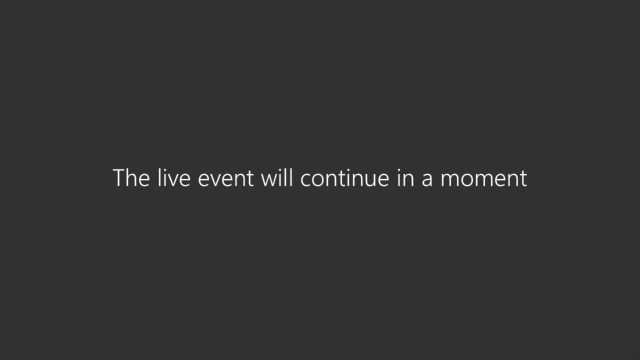 first of all, dear, i would like to thank mr ashish k tivari, senior software, senior software engineer robotics r d usa, for giving such an insightful webinar for us today. sir, we understand you have a different time zone. thank you very much for cooperating with us and doing the same and in 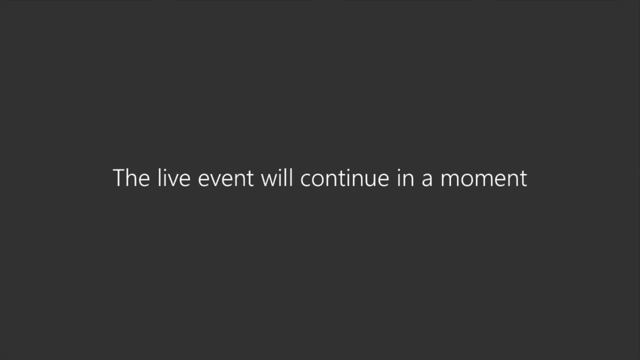 the same available time slot. thank you, sir. i'm sure all our faculty members, research scholars, students have really benefited from this webinar. thank you, sir. then i would like to thank dr nizar ahmad, chancellor presidency university, dr rada padmanabhan, ma'am vice chancellor, dr badri sir. 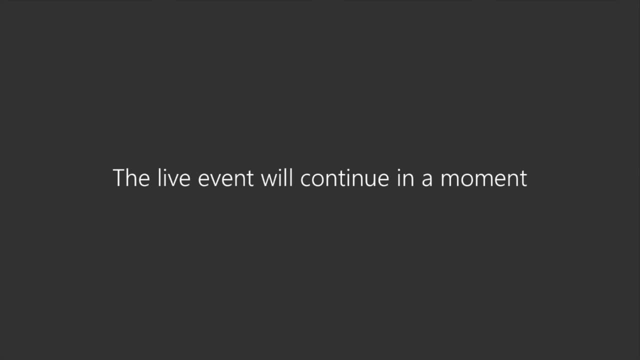 the registrar in charge, dr am surendra kumar, dean soe, dr kalai arisinsa, associate dean, school of engineering presidency university. dr k g mohan, professor and head of the department computer science and engineering, dr tivakaran ieee, faculty coordinator. then i would like to thank my 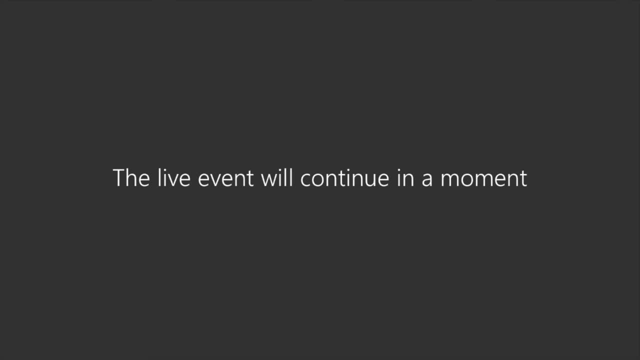 colleague, miss mithali ma'am, for organizing such an insightful webinar for all of us, for co coordinating it with us, sir. thank you, ma'am. then, last but not the least, i would like to thank miss charlene butnagar, ieee student branch counselor, for organizing such an amazing webinar for all of us and for 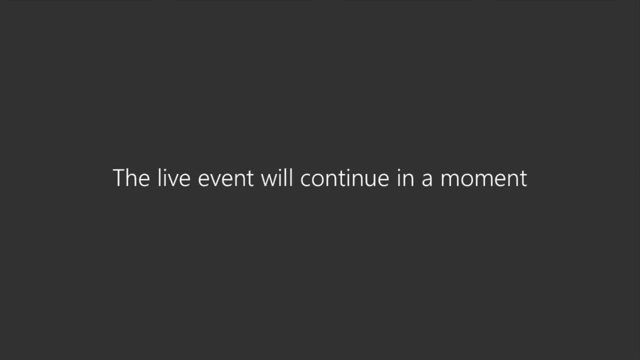 supporting it and providing a platform. last, i would like to thank all the participants who have joined us, joined us today. velita ma'am, your mic is mute. yeah, yeah. i would like to thank dr k g mohan, professor and hod computer science and department dr tk i i ee faculty coordinator, mithali ma'am, for organizing. 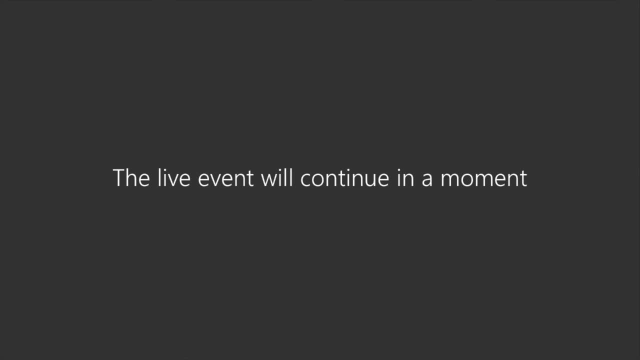 such an amazing webinar for us. thank you, ma'am, for sharing with uh, for coordinating with ashish ashish sir, and making this webinar possible. then i would like to thank miss charlene patnagar- i treat i triple e student branch counselor- for making this possible, for for standing as a support to 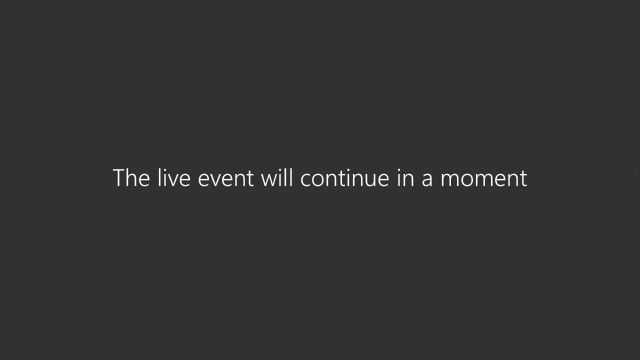 make this even such a success. last but not the least, i would like to thank all our participants- students, faculty members, i i t professionals, professors and everyone for participating and uh giving your valuable time to us. thank you once again. thank you. thank you so much, manita ma'am. 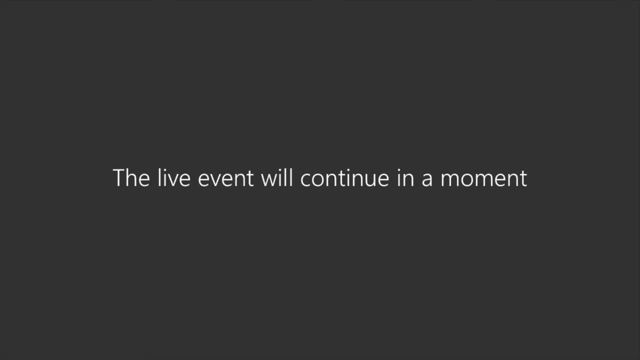 again. thank you so much, uh, sir, and thank you mithali ma'am. thank you, thank you, ma'am. so my participants- uh, the feedback link is shared with you. kindly give you a valuable feedback. we will be sending all the important resources to you, including the recording. so we will be mailing or we will be uh sending on telegram group you.